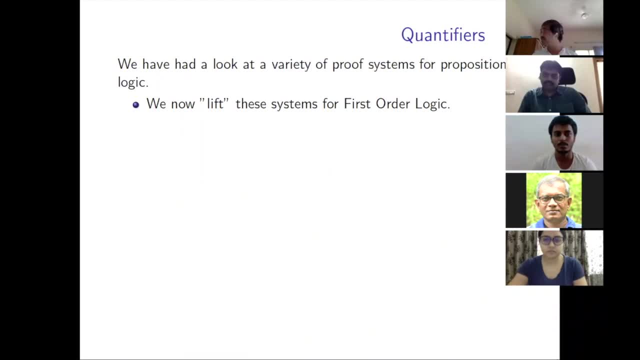 So we have looked at a variety of proof systems for propositional logic. We now lift these systems to first order logic, And so first order logic. what we have? well, the whole mess appears now right. We have a syntax of terms: constants, variables, function symbols. k-ary function symbols apply to t. 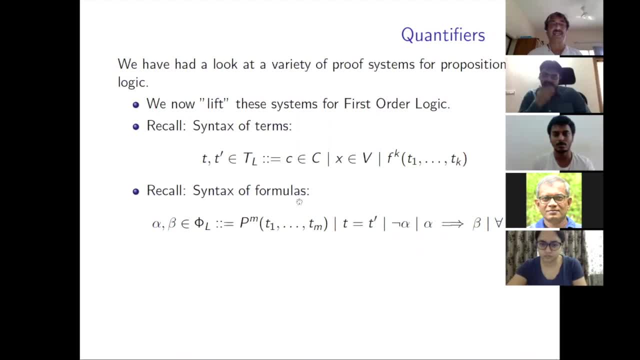 k terms. that gives you the syntax of terms. and then you have syntax of formulas. variable atomic formulas, which are predicate symbols, apply to terms, whatever the propriety. then you have equality, So… negation, implication: well, all the Boolean connectors, But, like I said, we'll keep for. 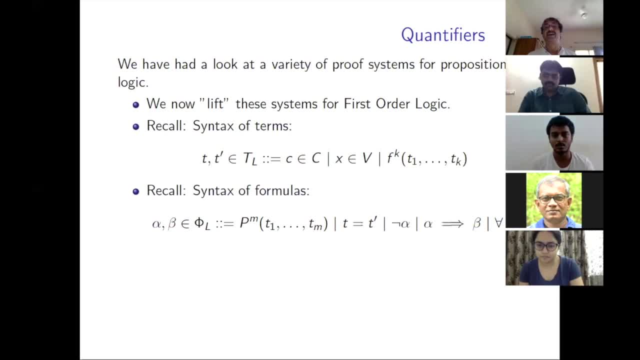 Hilbert system, we have only negation and implication and the rest is supposed to be defined in terms of these. And then you have quantifiers, Again for all alphas. enough, because there exist alpha you can define as not for all, not alphas. 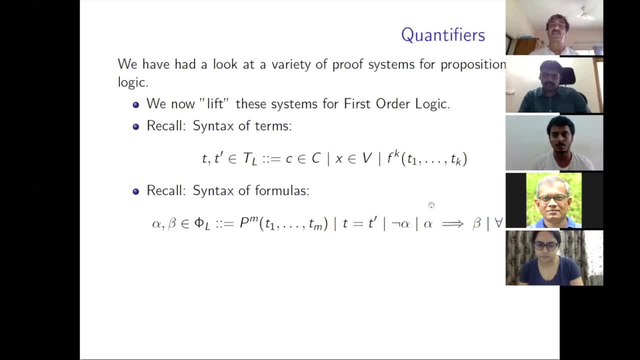 Yeah So, and mean syntax. So this is the syntax of first-order logic, and so this is what we started everything with. We have semantics by looking at L structures, interpretations for conscious symbols, function symbols, predicate symbols. that gives you L structures With assignment for variables. you get models and then in 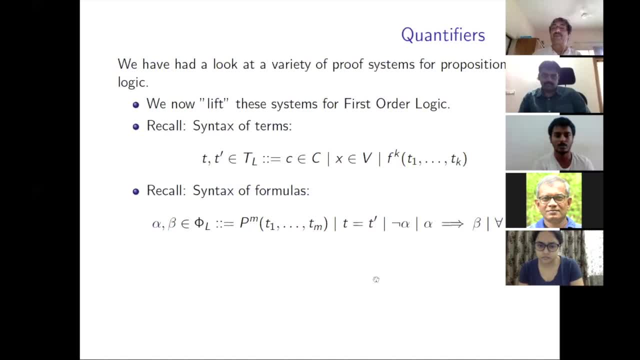 the model you define the truth of the formulas. From that we talk about the logical consequential relation and then the reductive consequential relation as a way of, as an alternative to it. This is how we did this whole business. So we first discuss Hilbert-style proof system before taking up natural reduction and 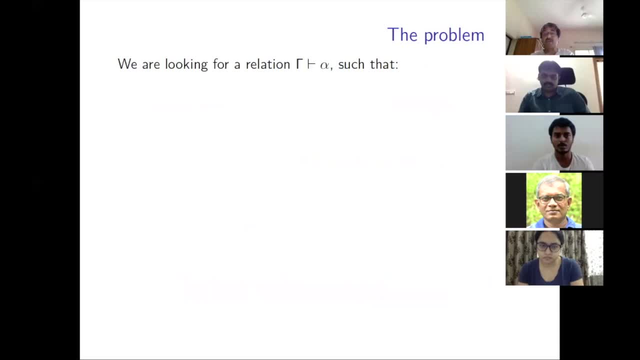 sequential calculus. So what is the problem? We are looking for a relation gamma turn-style alpha, such that whenever you derive alpha from gamma, there is a proof of alpha from gamma. Alpha is indeed a logical consequence of gamma and completeness There if alpha is. 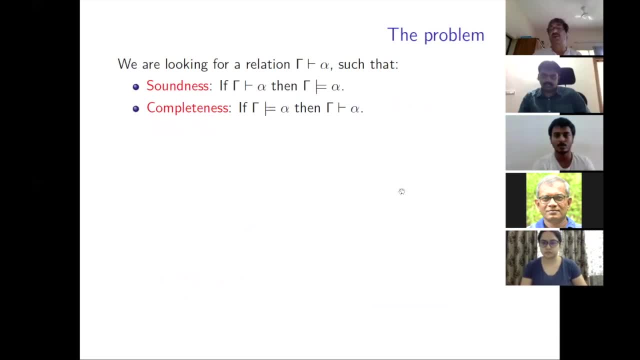 the consequence of gamma, then alpha is actually derivable from gamma. So to show soundness it's sufficient to prove that all axioms are valid and all inference rules preserve consequence. And there is this little mess about substitutional instance, What we call a axiom. 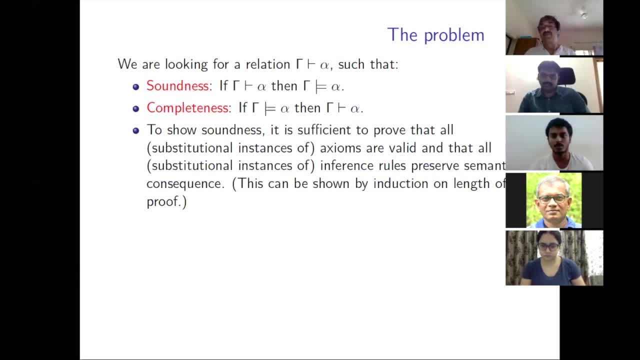 axioms are actually axiom schemas. so in general you have to talk about substitutional instance of axioms, so you have to show that all substitutional instances of axioms are valid. but that's, you know, very straightforward. and then your inference rules preserves the negative consequences. now we made one. 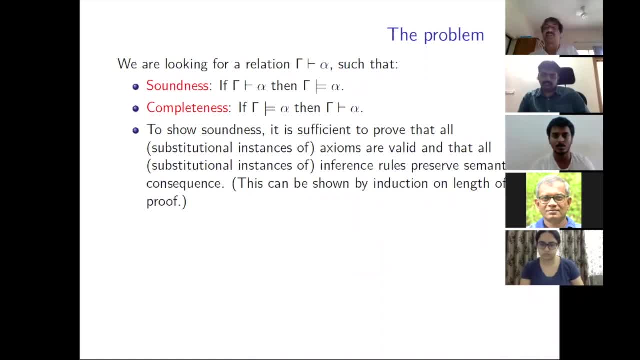 decision, namely that the only inference rule, we have only one inference rule, and that's modus ponens and of course that preserves consequence, straightforwardly. so that's something that you don't bother with and this is that sufficient? I mean, this proof of soundness is done by induction on length of proof and this is what 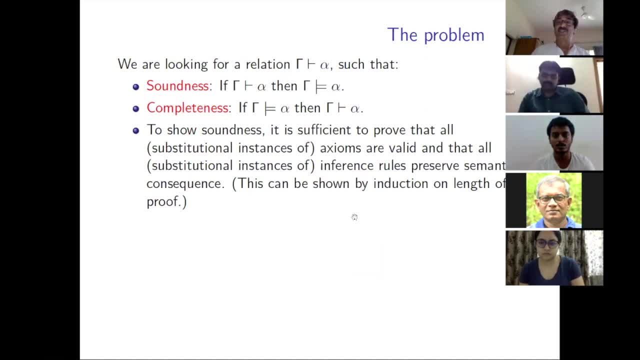 we did in propositional case, and the same thing holds in general. there's nothing to do with which logic. it's nothing to do with the syntax of logic. this is a more general statement about whatever logic you are dealing with. for completeness, you consider the contrapositive form, the way you prove it. 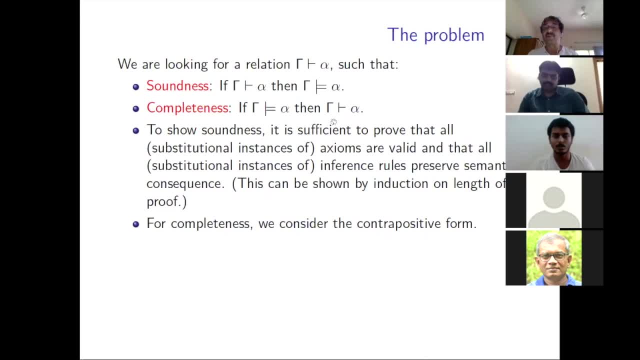 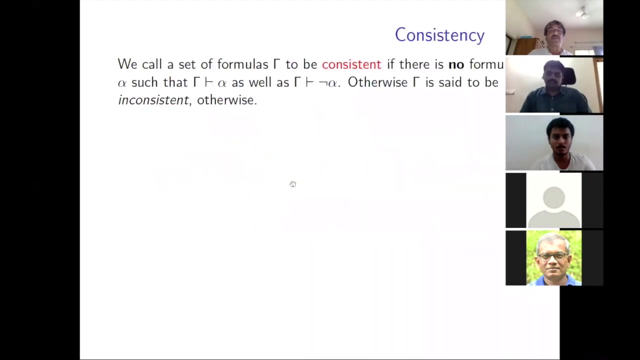 is that if you have a simple logic, you can have a simple logic, you can have a shift that you call the dagger algebra. in a little detail about that, but that that's just one建 drama. one is quite eight digits length, six digits length. one is in here eight digits. 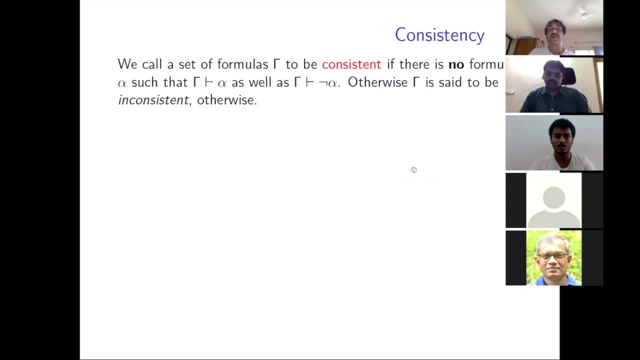 length, if you will, for your point. yea, and here that, back here here. if you hate me, you don't wait here. how do you use that? you choose your set of formulas to be consistent and have an journalists to answer the following- and we will talk about that in a bit, which is in the next section: just please ask here, you know. 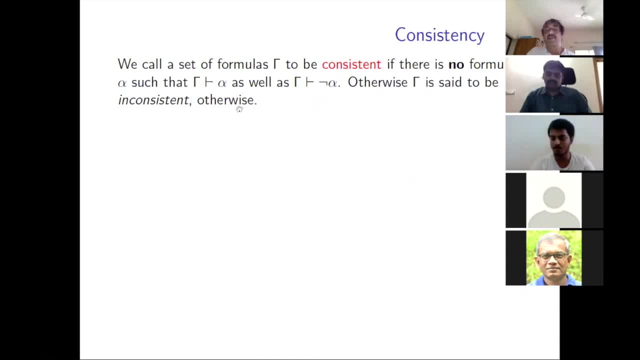 which one belongs to which one is非的 and if you are, in which one belongsation If there is no formula alpha such that you can derive both alpha as well as negation alpha from gamma. So consistent basically means that you cannot get a contradiction. 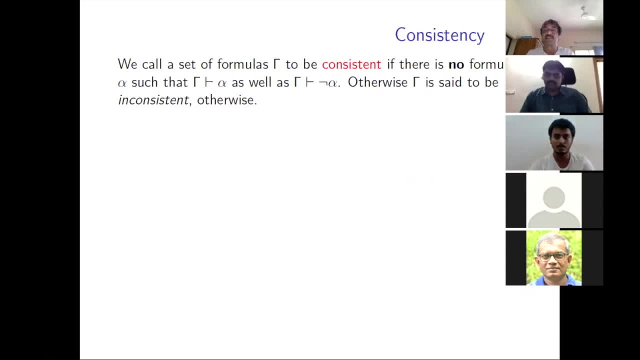 Contradiction means you are able to derive both the formula as well as its negation And you say that the set isn't consistent. you can't find such a contradiction. So remember, our exercise was that to show that, and I think this was in the problem set as well. right, 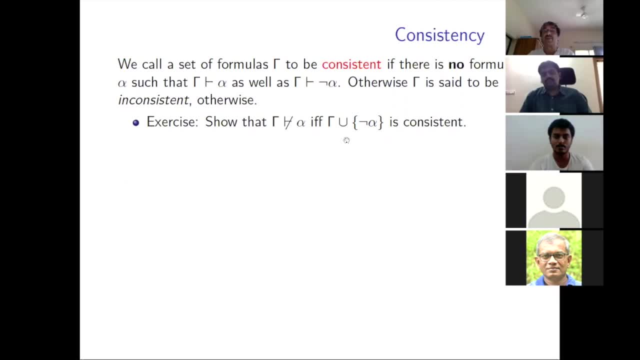 If alpha is not derivable from gamma, if, and only if, gamma union negation- alpha is consistent. And this is just. you use the propositional axioms to show this. So basically, all this is that a completeness theorem is equivalent to the assertion that every consistent set of formulas 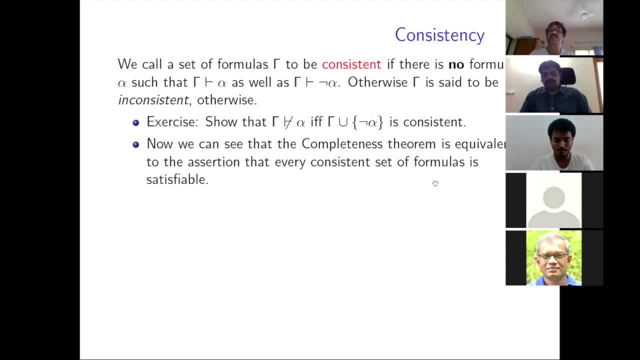 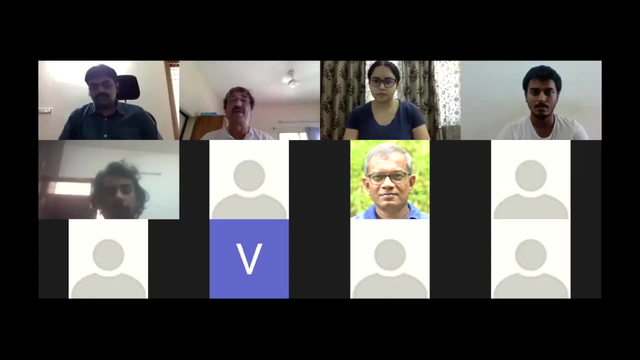 is satisfied. So you take a consistent set of formulas and you build a model for it. And is there any question regarding this? I am just recapping all that, but if you want me to go over anything particularly, we can go over it. 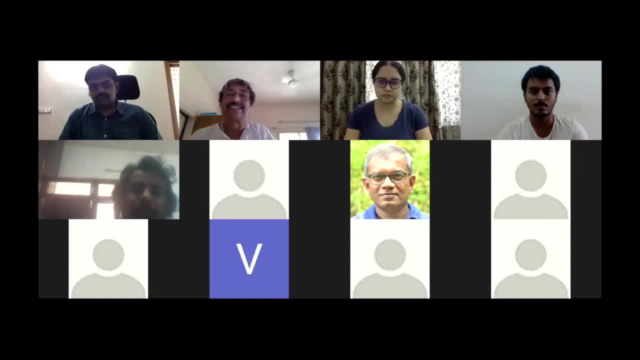 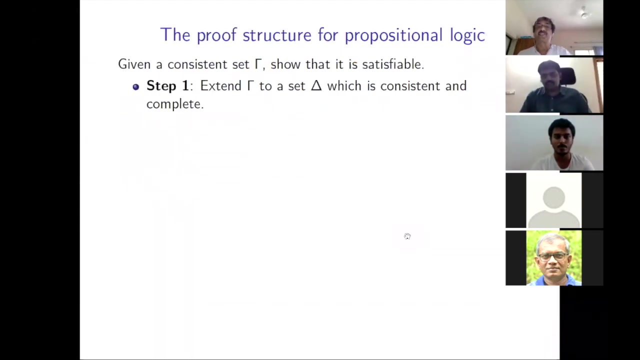 Is it all clear? Just a recall of what we did earlier. Shall I go on? Okay, Yeah, So how do you go about this for propositional logic? How does the proof? what is the proof structure for the propositional logic case? 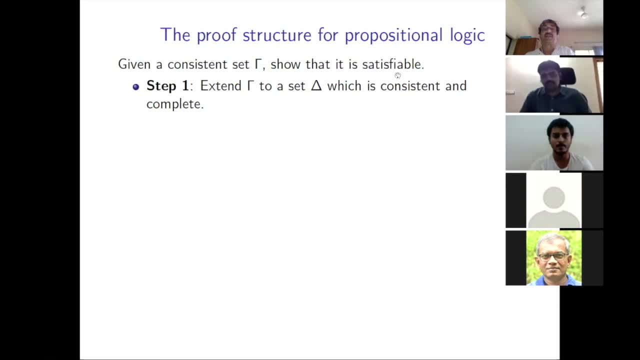 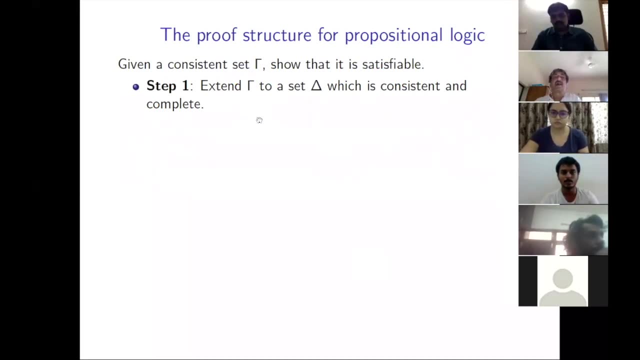 Given a consistent set gamma, show that it is satisfiable, Right And Well. how do you do that? First extend gamma to a set delta which is consistent and complete, And then define a model based on delta. In the case of propositional logic, you just have to assign a valuation. 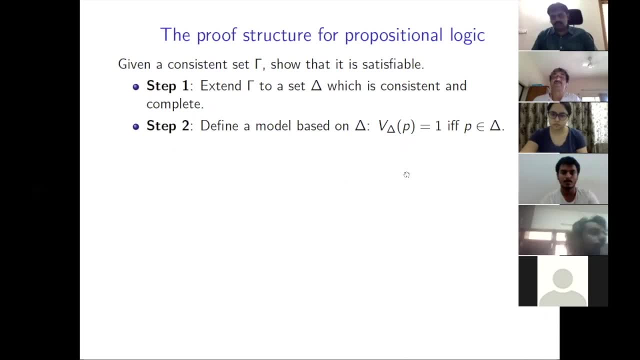 For p is said to be true if, and only if, p is a member of delta. And then you prove the truth, lemma, for all alpha. In this model b, delta alpha is true if, and only if, alpha belongs to delta. If you prove the truth, lemma, then you know that every formula in delta is satisfied. in this model, therefore, delta is satisfiable. and since gamma was a subset of delta, gamma is satisfiable as well. and you are done. 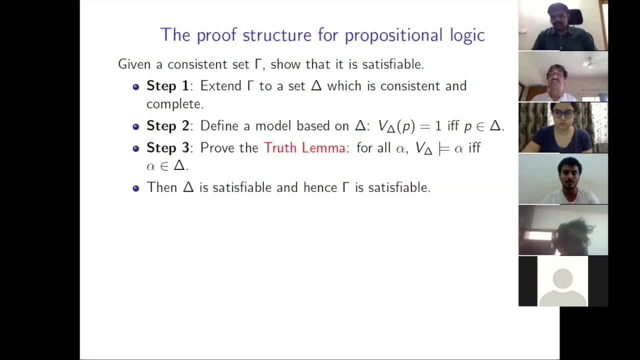 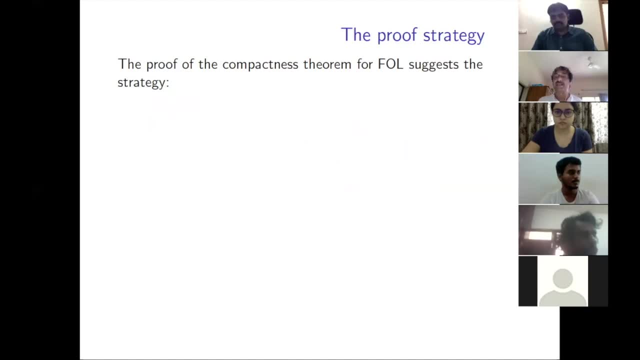 And this is the kind of recipe, this is the Hankenstein proof recipe that we follow for first order logic as well. So the proof of the compactness theorem, which we've pretty much did it at some length for first order logic. So just the same strategy, so the completeness proof same follows the same recipe as what we did for compactness. 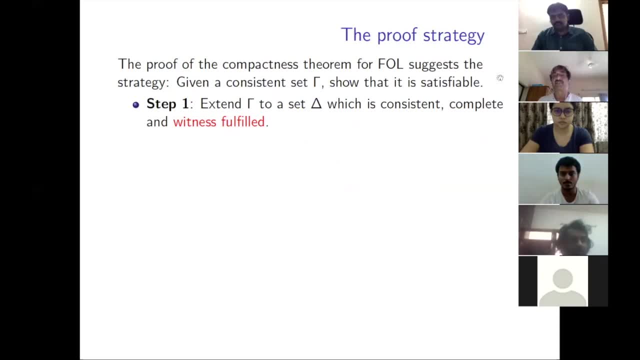 So, given a consistent set gamma, I want to show that it is satisfiable. How do I do that? The same step: one: extend gamma to a set which is not just consistent and complete but also witness fulfilled right. Remember, this is the extra step that quantifiers break. 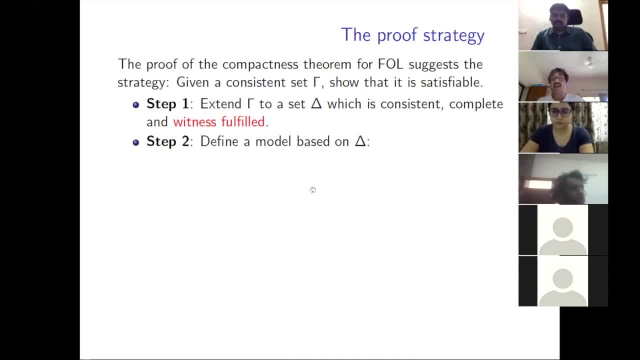 And Then define a model based on delta. Now, this is going to be a little more complicated, it's it's not just propositions being set to zero and one. the problem there is a problem with equality. So what you do is define a relation on terms, a binary relation: t twiddle, t prime. if, and only if, t equals t prime belongs to delta. 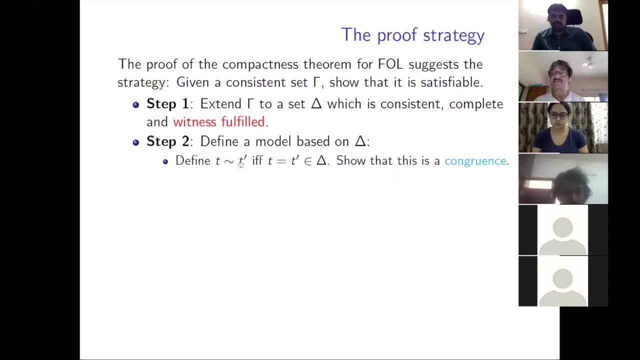 And now we show that this is a congruence, this is an equivalence relation right. And Then it's a congruence in the sense that if there are, if t one is equal to t one prime, t two is equal to t two prime, and so on, t k equals t k prime, then f of t one through t k equals f of t one prime to t k prime right. 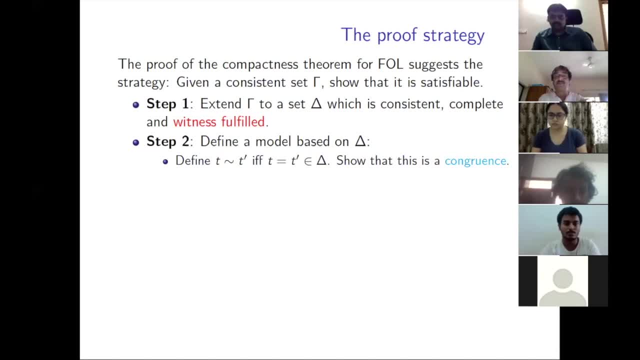 So in the context of application of function symbols the equivalence relation preserve is preserved. in the context of predicate symbols, same thing. If t one is equivalent to t one prime and so on, then p applied to t one to t one prime. take t one to t k is in delta if, and only if, p with t one prime except that's in delta. 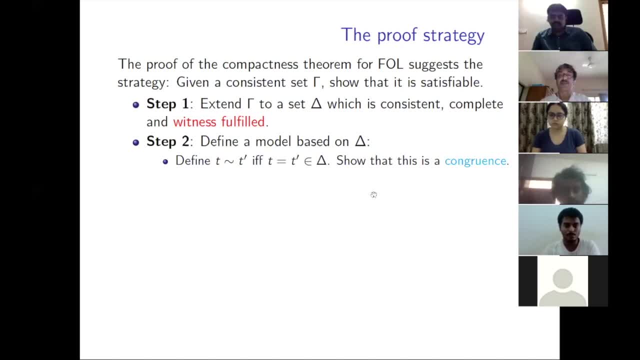 So this is what it means: for it to be a congruence And we show that, then that gives us the handle. then you take the equivalence class of terms and build a model- So the domain simply consists of Equivalence classes of terms- and then add the two points to the interpretation of p: if, and only if, this predicate belongs to delta. 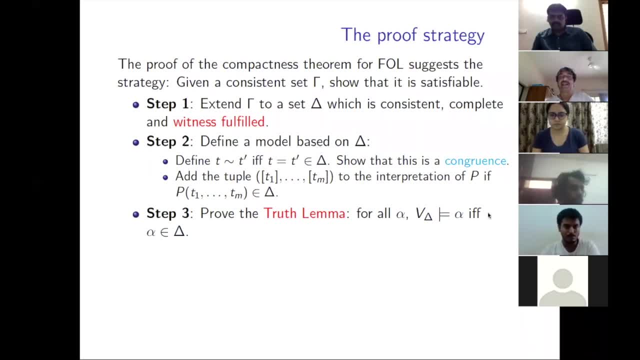 So this is what it means to say: it's based on delta. And then you prove the truth, lemma for all: alpha v, delta satisfies alpha if, and only if, alpha belongs to delta. And then this tells you that delta is satisfiable and hence gamma is satisfied. 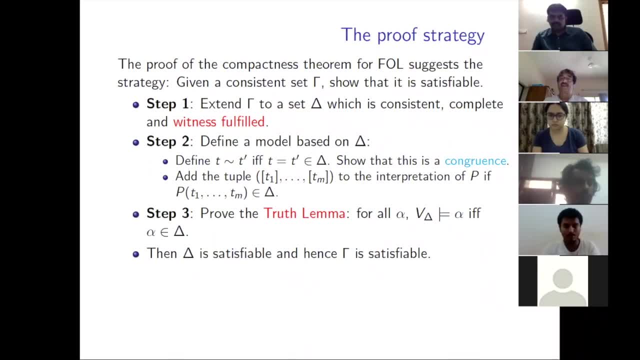 So this is really the proof strategy. Whatever we did for you- remember for FinSAT, in the compactness case, you were given a set gamma where every finite subset is satisfiable and you have to give them show that the set is satisfied. 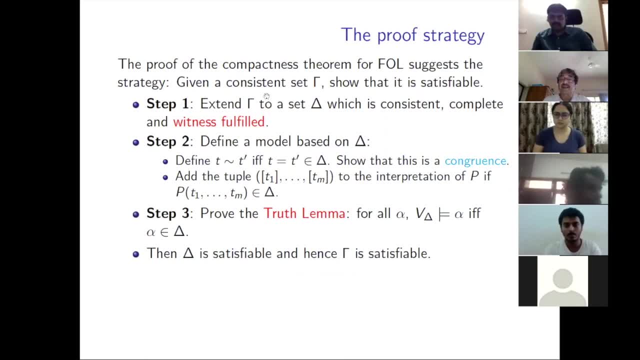 For that we did all this. Now we do the same thing with a consistent set. Now remember, even at the end of propositional logic, this thing that I said: of course you can also use the statement of the compactness data. 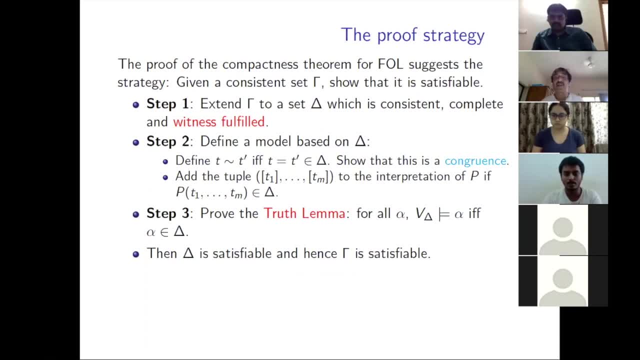 And then you should be able to prove that every valid formula is in fact derivable. right, then you, simply you can use compactness data to prove the complete mistake. What does it mean? valid formula? that means you're not. there is no gamma right. take any formula that is true in all models. you must show that there is a derivation for it. 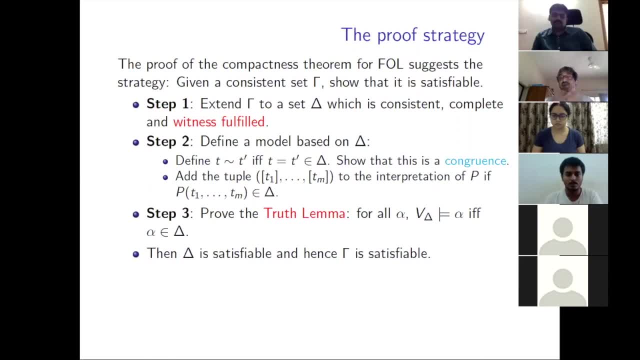 Now, in the case of propositional logic, you can do a direct proof. You just look at alpha, look at the fact that it has got only finitely many propositional symbols, and you want to say that if, okay, if there is got k propositions. 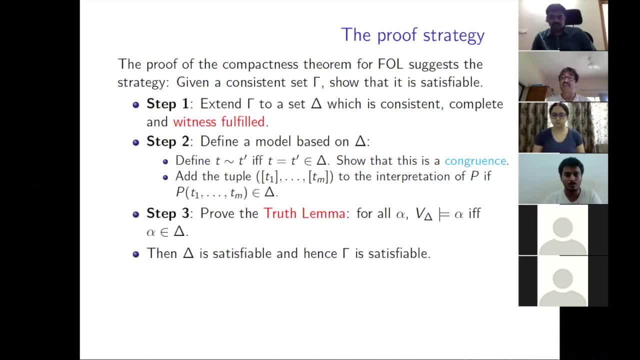 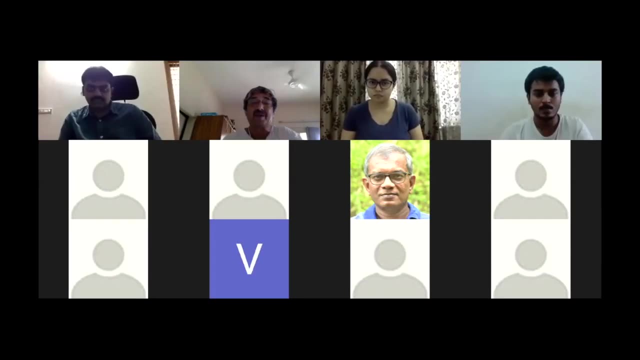 look at all possible. you know k tuples or Boolean vectors in each of them. it's true, and use that Now. one of the exercises that I gave in the problem set 3 is, yeah, so I think one of the exercises. 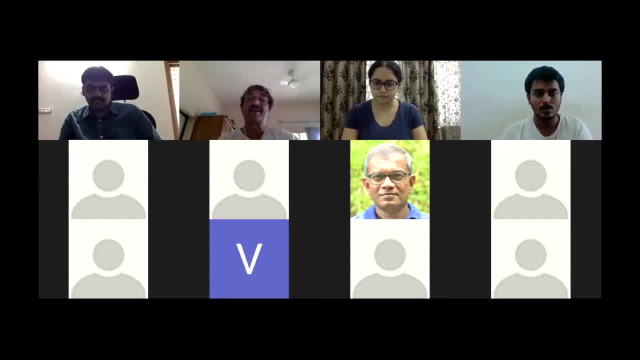 was to actually do a direct proof of that, show that every tautology is actually derivable in the Hilbert system. This is the Carnap style proof and there are enough clues there for you to actually do by induction on the number of atomic propositions. So once you have a direct proof like that, you can appeal. 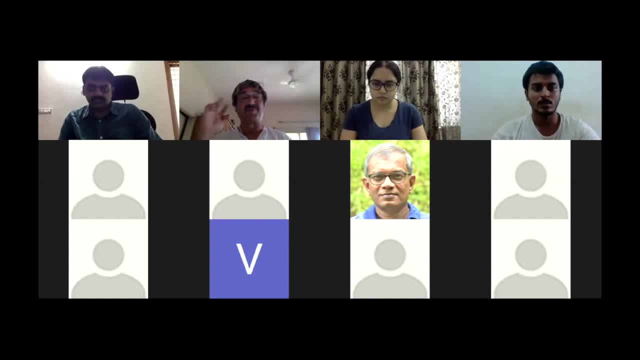 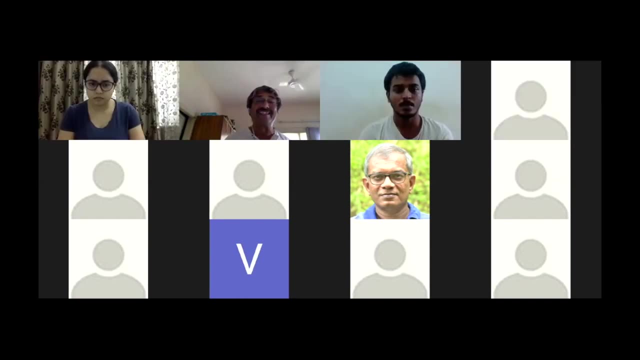 to compactness theorem and do the completeness theorem as proof. Unfortunately for first-order logic, it's not clear at all how you, even though alpha is a single formula, valid means what It's true in all models right? This is not like in all valuations. You can't just look at alpha and guess some. 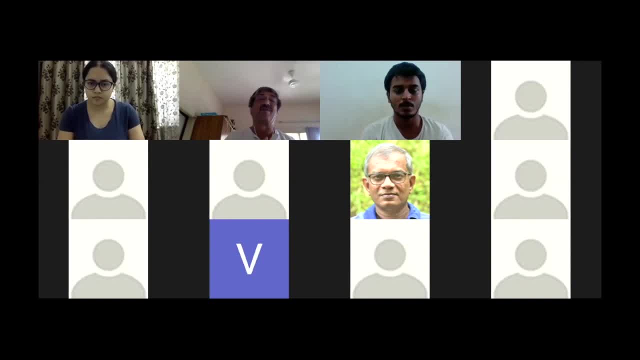 structure and then do induction on something. So it's not clear at all how you would go about the proof. So, in fact, the root is the what we have gone through, which, incidentally, will give you compactness theorem as a proof. So, in fact, the root is the what we have gone through, which, incidentally, will give you compactness theorem is a. 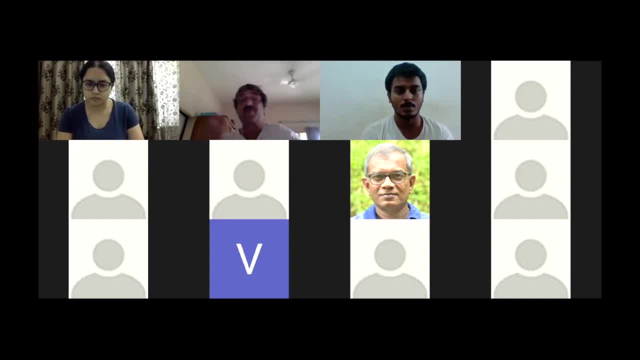 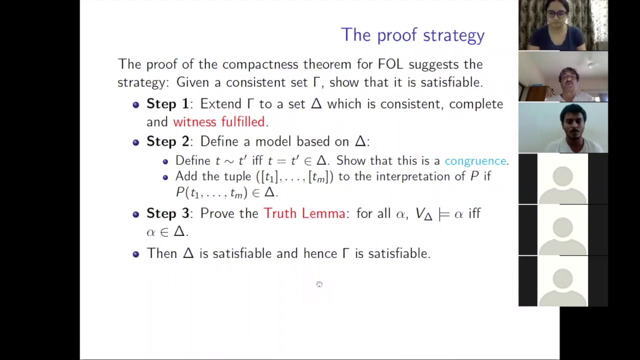 corollary. but you know, you have a proof of completeness theorem in the line that I was just talking about, where you start with a consistent set and actually build a model for it. So this is the recipe, and so how do we do the proof? Well, the first part. 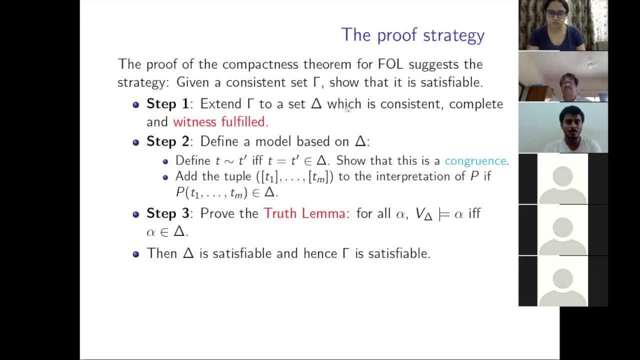 well, given a consistent set, you want to extend it to a consistent complete set. Complete means that for every formula it's got, you know, either the formula belongs to it or the negation of the formula belongs to it right Now. okay, and that's a. 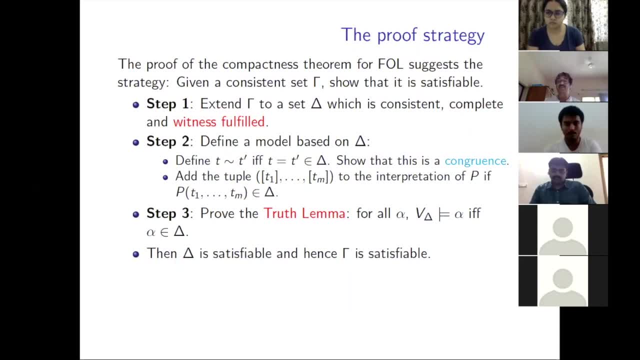 straightforward matter, as we have seen: Enumerate all the formulas at every stage. If you want to add it, check that it preserves the addition, preserves consistency, then throw it away. Then, sooner or later, one of the two formulas will come and you can prove that for every formula. if gamma is consistent, then for any formula either. 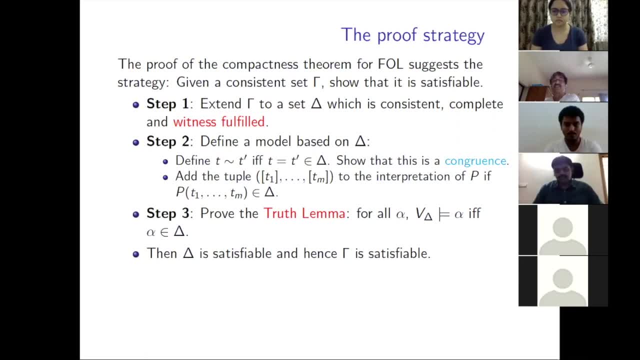 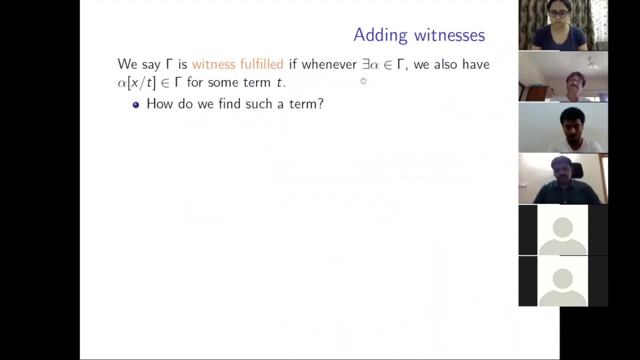 gamma union alpha is consistent or gamma union negation alpha is consistent. You can always consistently add one of them and that ensures completeness. But witness fulfilled, what does that mean? It means we say gamma has witness fulfilled if, whenever, an existential formula belongs to gamma. where? 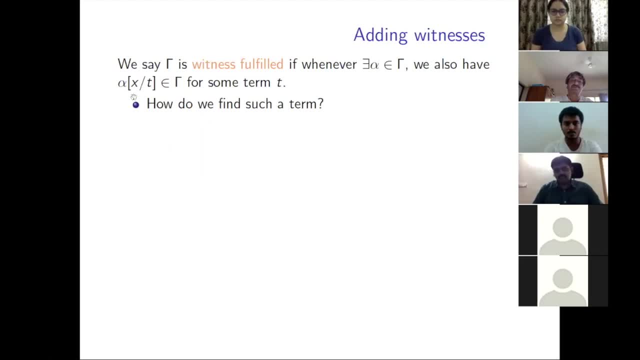 existence means that the existence of the existence, of the existence of the alpha belongs to gamma. we also have alpha with X replaced by T belongs to gamma for some term. T because we want to build a term model right For a term model, existential. if you say there exists X, there has to be some term in the. 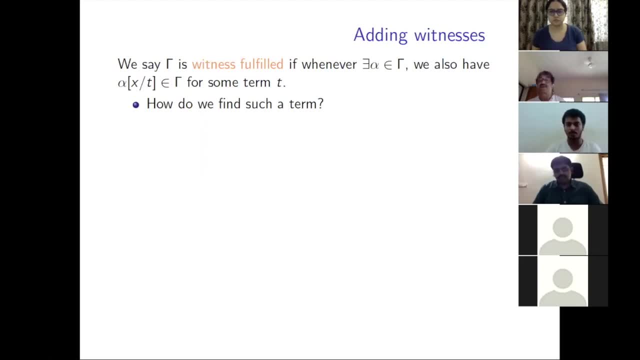 language witnessing that existence, right? So therefore, there should be something like this for some term T, in particular, it should be some substitutable term, right? so this is somewhat we want. but how do we find such a term? now? if you recall the compactness theorem argument, how we did was the girdle trick, and this is the 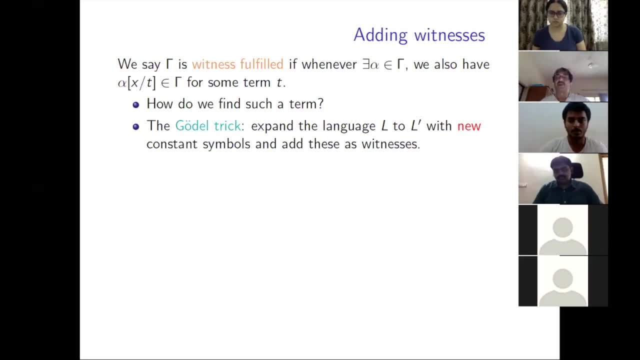 you know, very, very nice idea of girdle. expand the language l to l prime with new constant symbols and add these as witnesses, so these becomes names right, so that whenever? uh, so the key lemma is that whenever you have a set of formulas, an alpha, a formula such that 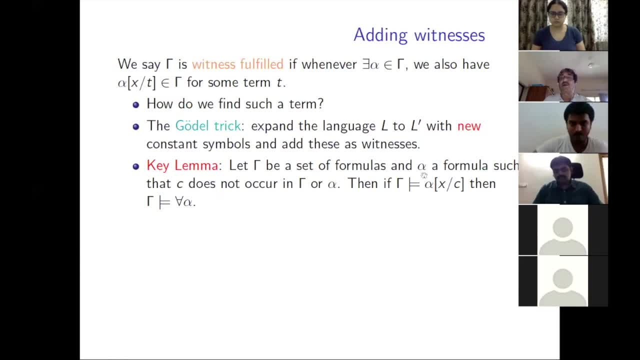 it is the constant symbol c that does not occur either in gamma or in alpha, then if alpha, with x replaced by c is a consequence of gamma, then for all alpha- oh sorry, this is for all x alpha, right? obviously for all alpha doesn't make sense. so this is generalization from constants. if 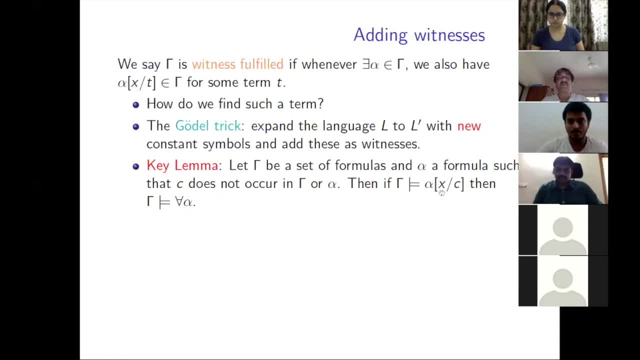 alpha is a consequence of gamma. it takes replace by c, then for all x. alpha is a consequence of gamma. this is the key lemma and you can now use this because whenever you've got there exists l x again. that's a mistake there and because of that there exists x. alpha belongs to gamma. note that. 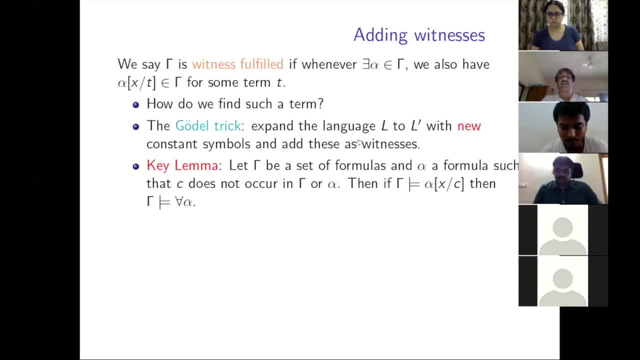 if you cannot consistently add alpha with x replaced by c, right, what does that mean? that is, adding gamma. you've got gamma as a consistent set if, by adding how to wait for the, it's too low Champa in the case of compactness, adding alpha with x replaced by this new constant symbol. 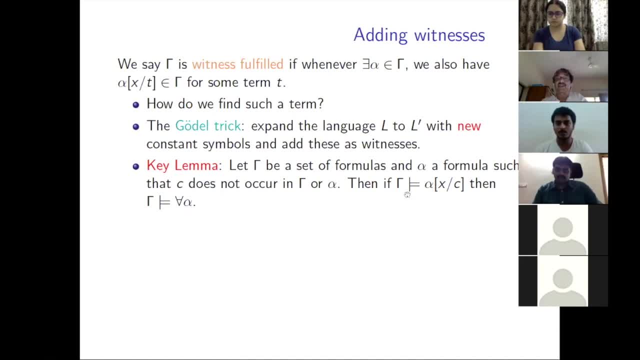 makes it violates thing, right. that means adding it makes it unsatisfiable, right. what does that mean? that means that negation of the formula is a logical consequence of gamma. and then you will say that for all x naught alpha and ch, alpha has a consequence of gamma which contradicts the fact that there exists. 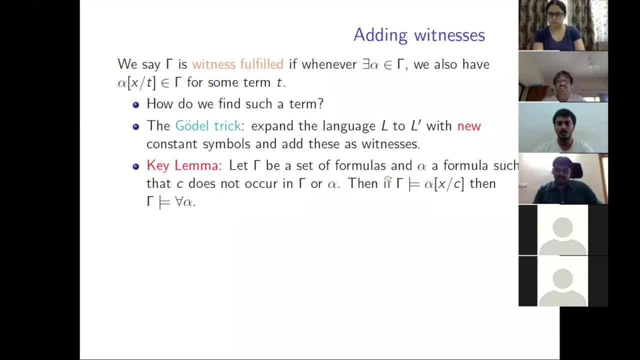 6 alpha belongs to gamma. This is how we did the proof. So this is the key level: Generalization from constants. Once you have this, it says that witnesses can always be added consistently. Now, of course, we can't use models. We have to do this. 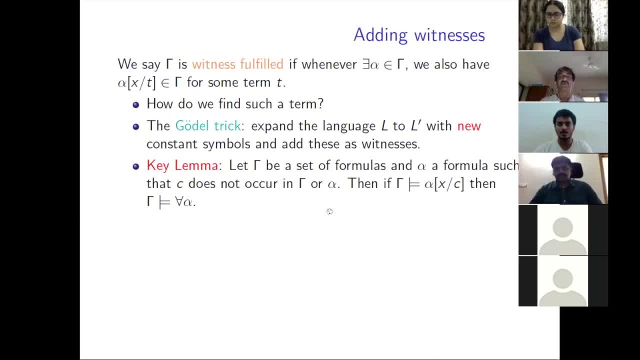 with derivations, But this is the basic idea. So from gamma we constructed this delta by adding witnesses and then finally, we showed delta as satisfiable. But when you say satisfiable, what you are constructing is an L prime model. L prime is the expanded 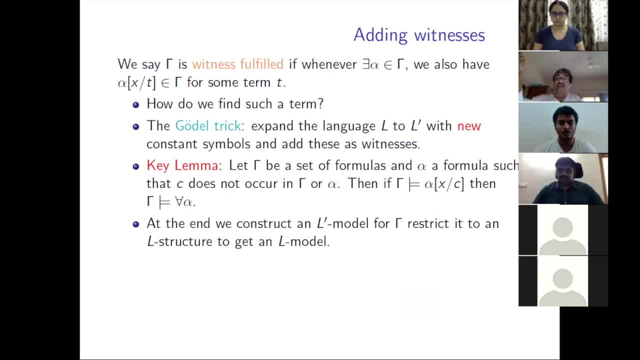 language. Remember, for the language L, you have L structures. The language L prime, you have L prime structures and L prime models And that's what you have got. So you've got an L prime model for gamma, restricted to the original language. That means your interpretation for 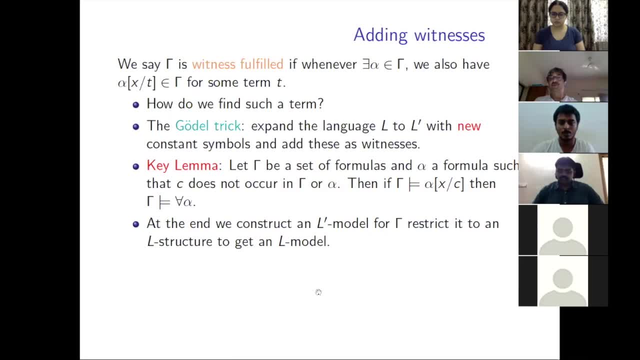 the new language. you take that and restrict it to the interpretation for the old language, And what you get is, in fact, the L prime. So this is the Gödel trick, and it works very nicely, So we need to do something similar. So now, of course, this is how the proof is done in. 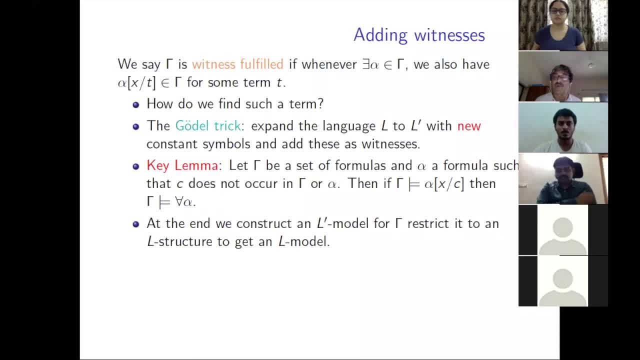 many texts and but what we will see is, I would like, I mean I'll introduce a slight variant which is our own trick, which is to say that look, after all, you don't have to mess with this expanded model and restricting I mean expanded language and restricting the language and all that. 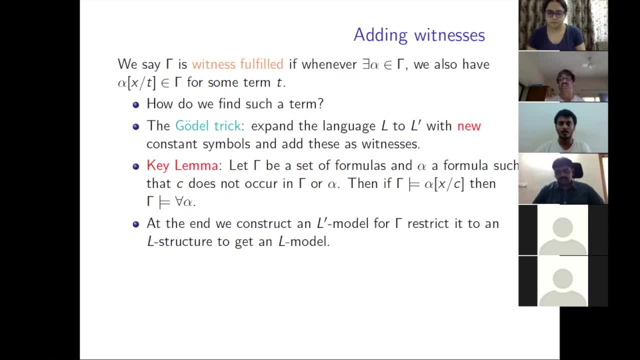 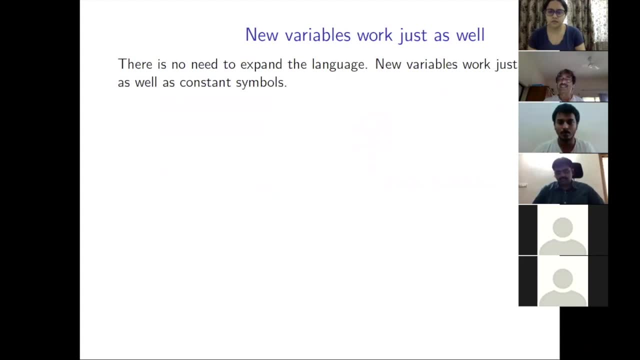 It's perfectly alright to work within the same language, And for this you make an observation And what you realize is that I don't need new constant symbols. New variables work just as well as constant symbols. Now, how is a language defined If a stutter language is defined? 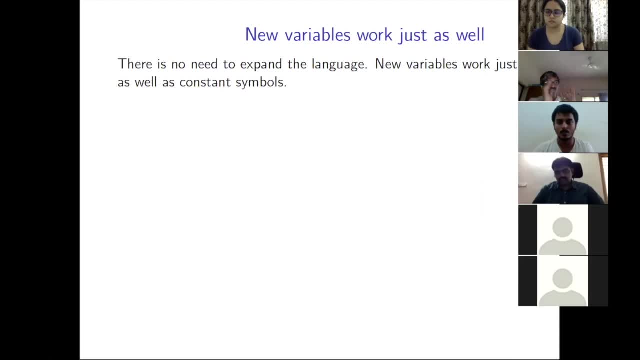 what are the parameters? Some bunch of constant symbols, some bunch of function symbols, some bunch of predicate symbols, Right And then, for to get the syntax of terms, you take a countable set of variables and do the whole business. Right Now, the variables are not part of 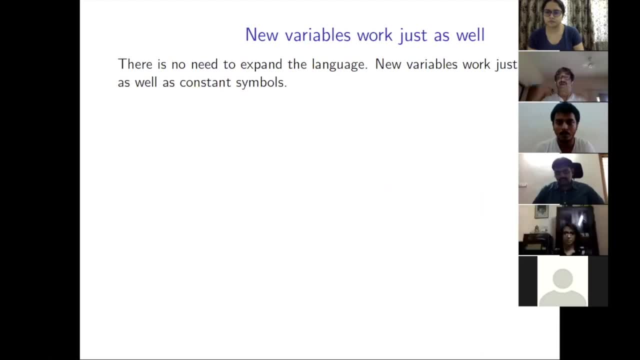 the language Right. This is just part of the logical structure. Exactly like you have your connectives, quantifiers and so on, you have variables. Variables are always there and you can always use new variables. Now, where will you go for new variables? Well, we start with the consistent set gamma. 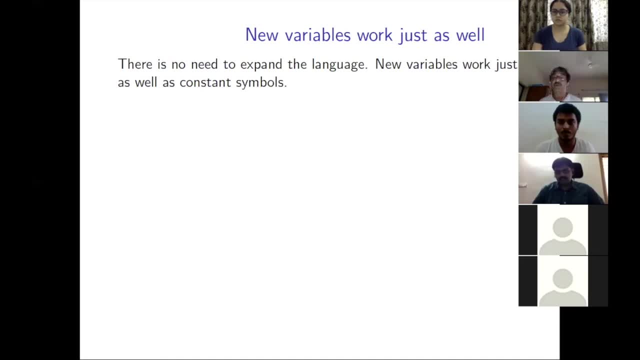 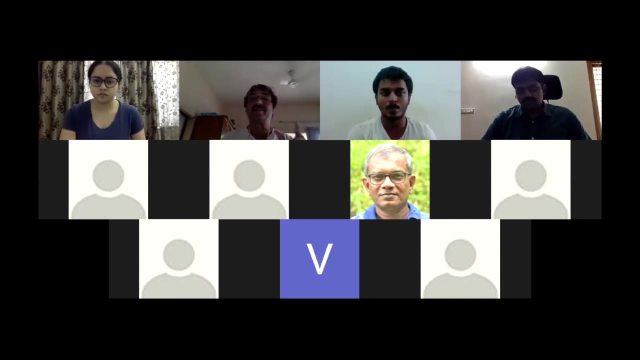 And whenever I see there exists x alpha use, find a variable that's not in gamma right And use that as the witness. Okay, let me ask you: how do you so you understand the logic of what I'm saying? right In the, in the bomb construction, you enumerate: 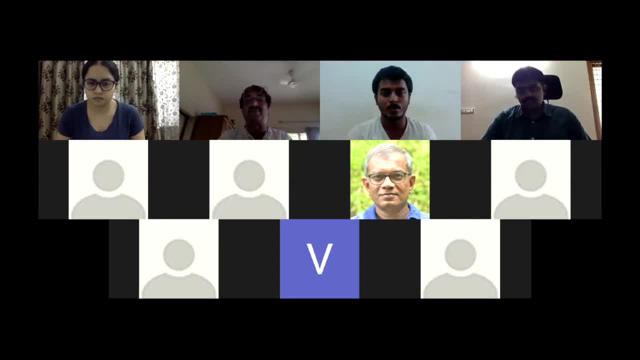 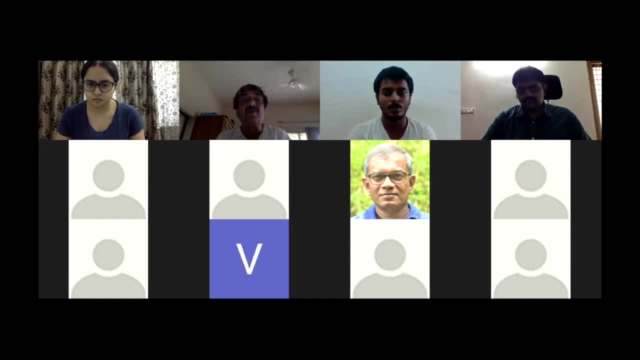 the formulas Anytime you see there exists x, alpha. right, You're going to throw in alpha with x, replaced by a variable y that is not used. in so far, Why would such a variable exist, Siddharth? what do you think, Sir? because the set of variables is: 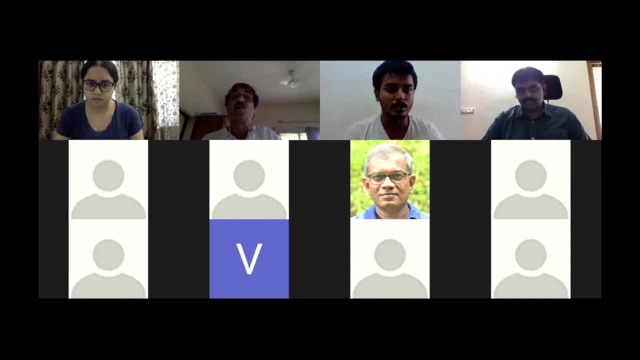 countably infinite. we can always bring in a new one. How, What do you mean? bring in a new one? Look at all the variables used in gamma right, And then you have to pick something that's not used in gamma. 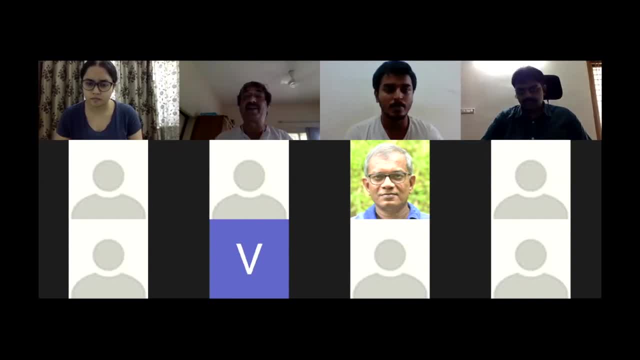 And you might be just unfortunate, because gamma uses every single variable that you've got. What's stopping me from writing p x alpha, px0,, px1,, px2, etc. For all xpx, right, But I have actually chosen to write it as that. 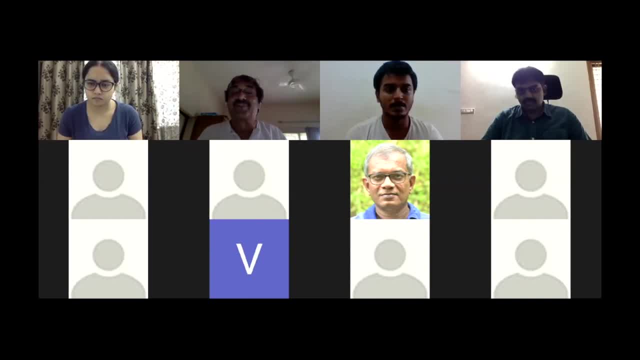 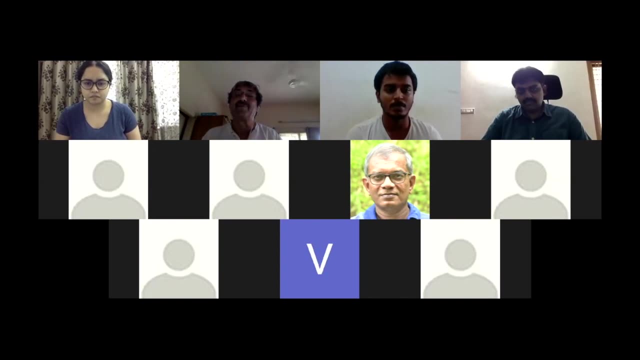 You can't stop me from writing a consistent set of formulas like this right. So, for instance, I could have just written p xi r, not p xi. True Right: p x r, not p x, is a tautology right. 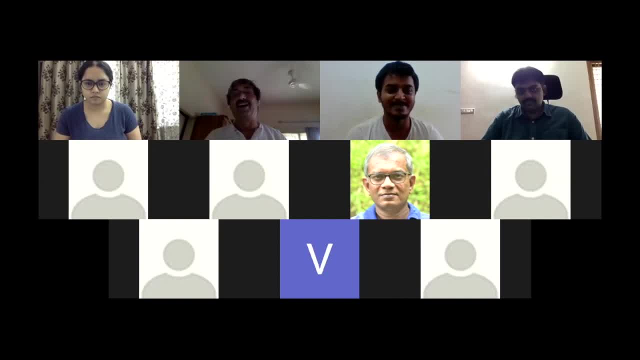 right. I simply sit and write it for every single variable and add it to gamma. perversely, You understand the point right. So you can't make some assumption, simply because it's an infinite set, that there is a variable waiting around for you. Yeah, So you have some work to do for that. 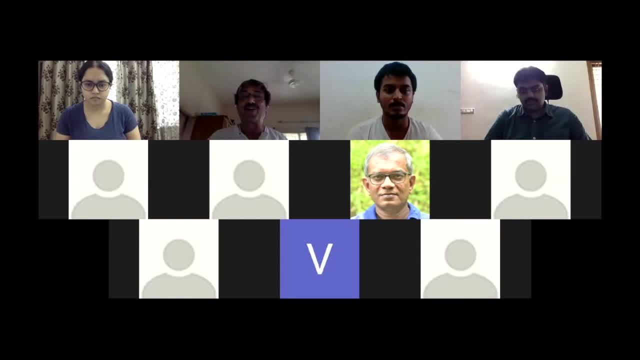 But I mean, like you said, after all, these are infinite sets and you can always find room. So you know of Hilbert's Hotel, right? Have you heard of Hilbert's Hotel Anybody? Ananya, have you heard of the Hilbert's Hotel? Okay, Hilbert's Hotel is a place where 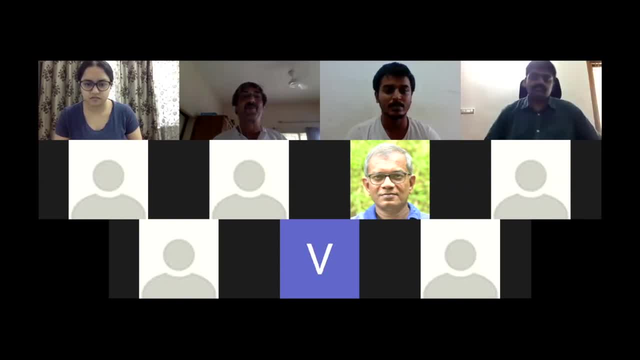 there is this guy. he was working as a clerk and so it has infinitely many rooms, countably. And so when people come, there is always room. And then one day a truck came which has infinitely many people, countably, many people. That truck holds countably many people. And the guy said: 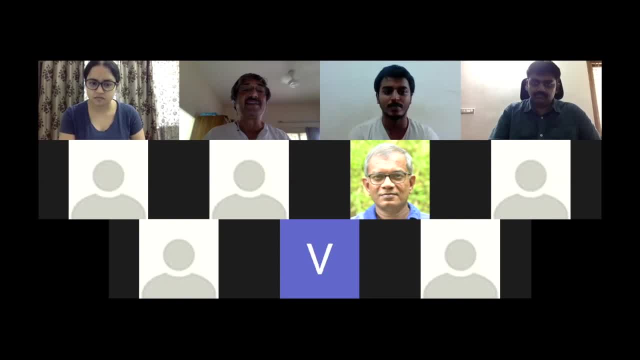 no problem at all. How do you accommodate this truck full of people in the Hilbert's Hotel? Yes, Ananya, It's full. The hotel is full, But the clerk says: no problem, I will accommodate the entire truckload. 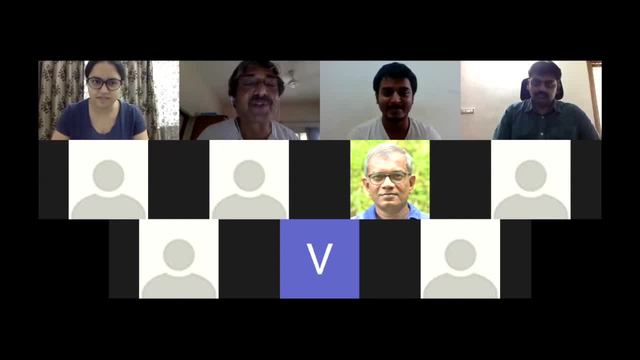 Yeah, Sorry, I couldn't hear what you said. Ananya, Yeah, Yes, but how? Yes, but how? So you go to the public address system and announce that if you are in room K, you move to room 2K simultaneously, So expect that the lower 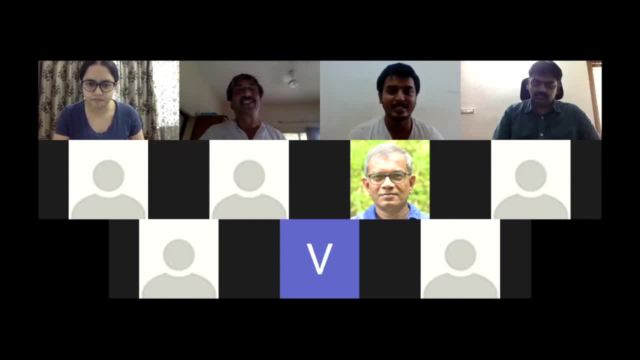 number of people will have to wait a little bit so that the higher number people move first, Right? So at the end of the day it's the size. all the even numbered rooms are full and the odd numbered rooms are vacant and you accommodate your truckload. 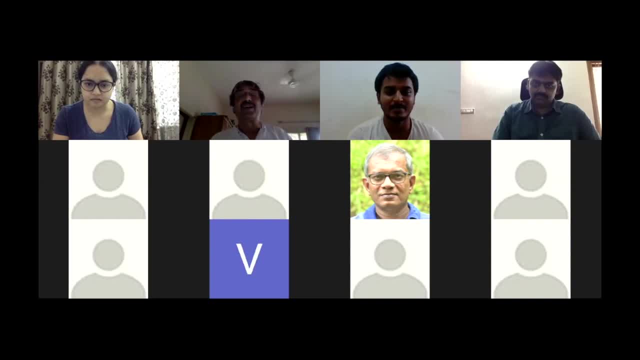 Right, Right, Yes, Yes, Sir, Yes, Sir. and then it turned out that after an hour there was a rock concert. and then he looked in the garage- you know parking lot- and found countably many trucks each having countably many participants. so did the clerk accommodate them? that's up. 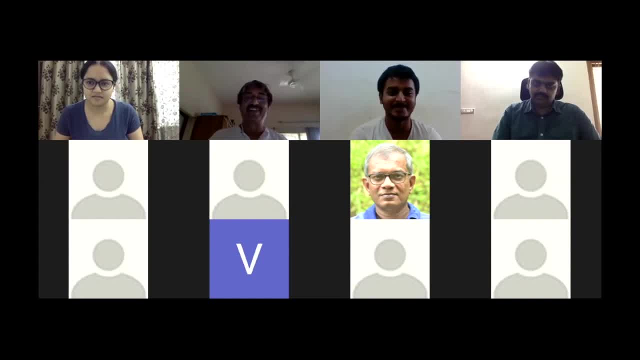 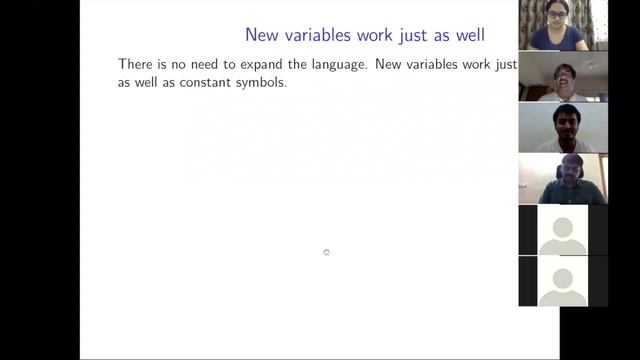 to you to figure out, okay, so let me get back to the lecture. so, and that's the basically the idea, right? so what we do is you have the countable set of variables. so in the given consistent set we replace every variable xi by x to y. right now all the odd index variables are: 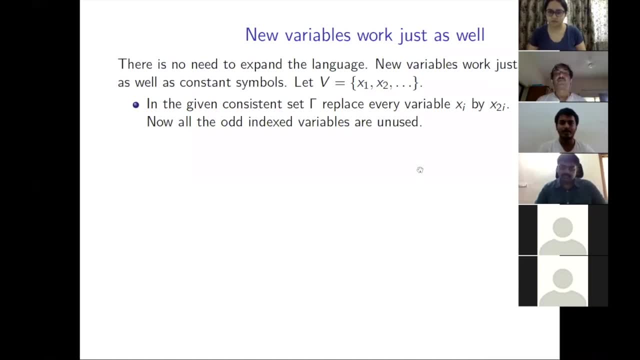 unused right, so you get. but of course you have to show that the new set gamma prime is consistent as well. that's important right, because you are given a set gamma which you are assured is consistent. you have done something, some mess with it. whatever you've done, 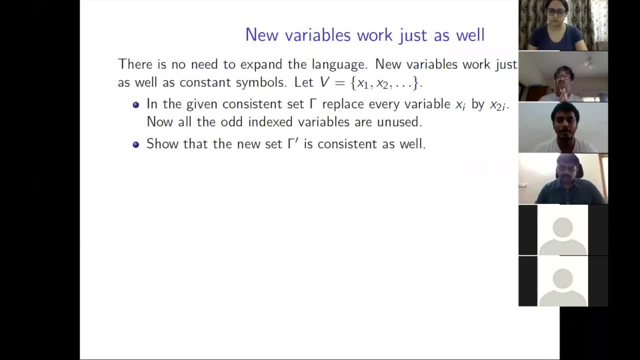 we have renamed all the variables right, so now you have given countably many new variables available for siddharth to take and put in formulas. but you also have to prove that what you've got is consistent. how do you prove that it's consistent? well, 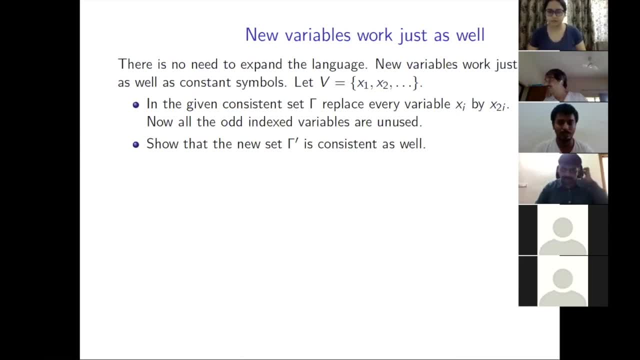 suppose it's not consistent. it's inconsistent, then something is derivable from that. you have to use that together and this is where you have to use axioms. right, you have to use axioms and inference rules to make sure that replacement of variables preserves consistency. yeah, 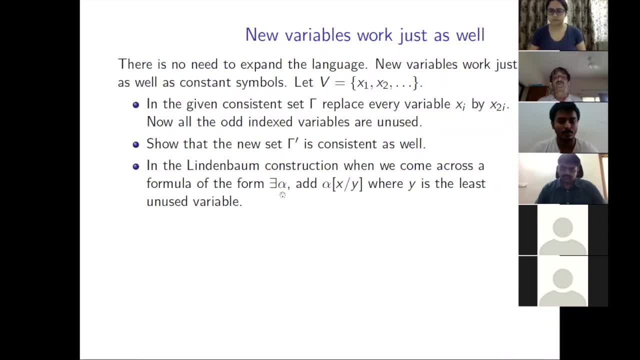 so in the lindenbaum construction, when we come across the formula of the form i keep that's a cut and paste problem. everywhere you'll find the same thing. it's obviously. there exists x, alpha, not the x and alpha, with x replaced by y, where y is the least unused variable right. 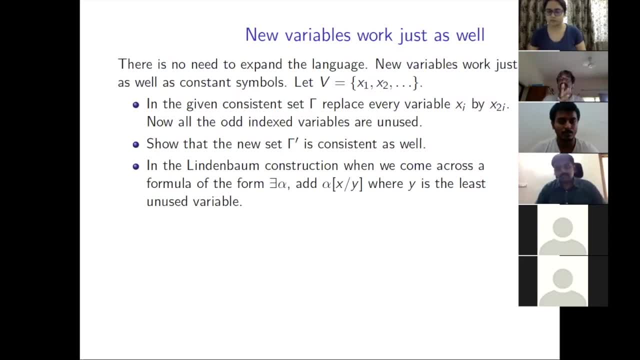 so why? because when i start a construction i know that there are there's a contablet supply available. at stage k i would have used utmost k new variables. so yes, there is a new variable. there are lots of unused variables. pick the least among them in the index and use that as a 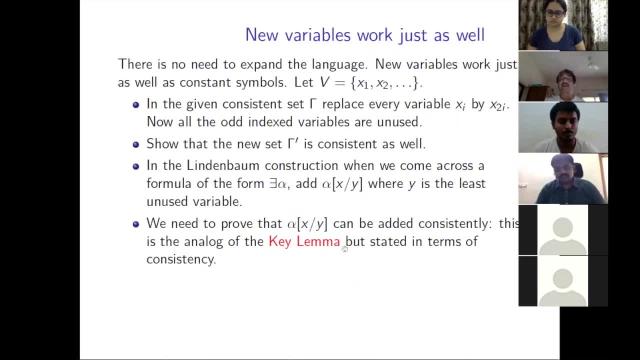 variance. we need to prove that alpha, with x replaced by y, can be added consistently. this is the analog of the key lemma, but now stated in terms of consistency. right, you remember what we said: with constant symbols, we have to do with variables, and we'll prove that once. 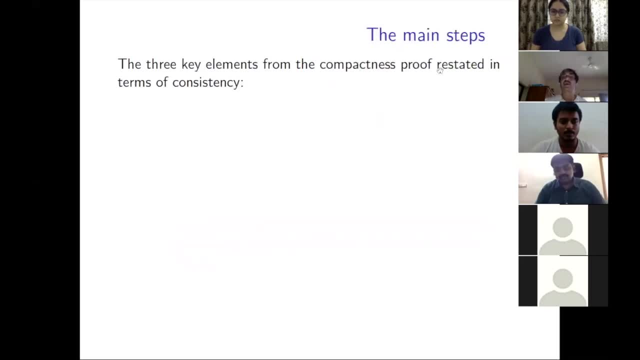 you do that, this is okay. so the Cree: what are the main steps of the proof? so, if you remember, from the compactness argument, there are three key elements from the proof, restated in terms of consistency and once you fix this, these were the main things, with compactness, with quantifiers, and that's exactly the 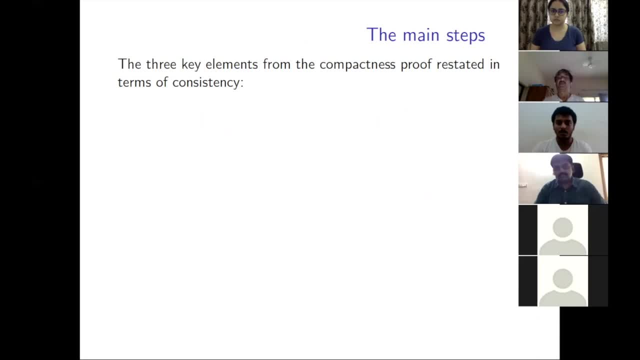 main thing that we need to do for doing completeness theorem of quantifiers. what are the steps? first, I already mentioned that we defined this binary relation on terms and we have to show that it's a congruence based on the fact that Delta is a consistent and complete set. 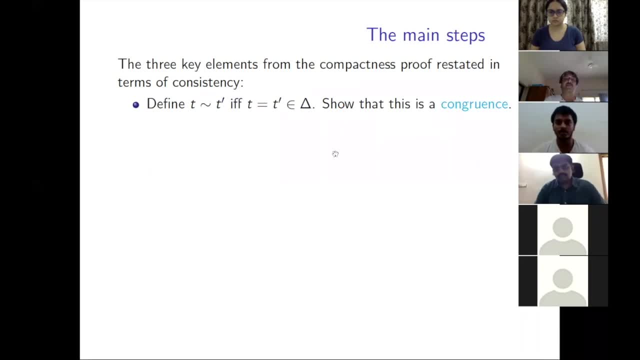 so this will involve some exams and rules. surely? second step- and remember this, this was a pain that we all went through- right, given any Alpha variable, X and the term T, there exists a variant formula on four prime such that Alpha is equivalent. alpha prime is not just valid, but it's actually terrible. and T? 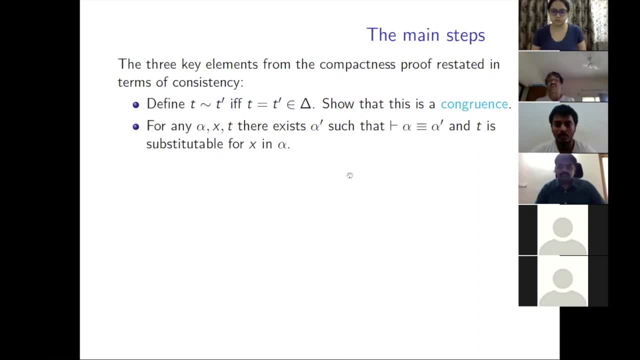 substitutable for its knowledge. you give me any formula, variable, x and the term t. in general, t may not be substitutable for x and alpha, but i can always rewrite alpha to an alpha prime for which- and this is not alpha here- it should be alpha prime. yeah, sorry, and so there exists an alpha prime, such that the given term 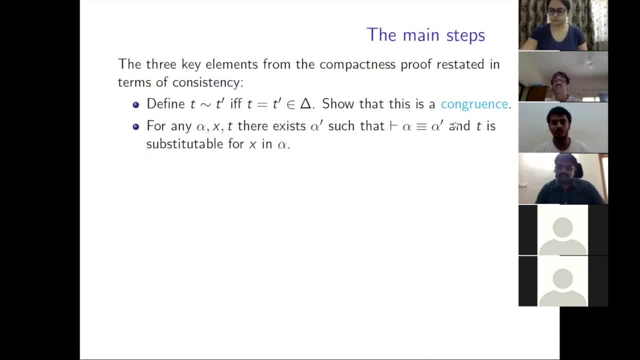 is substitutable for x in it, and these two are logically equivalent, right, and that's something that i can derive. so this will again involve some axioms and proof rules, because how will you derive this without having appropriate axioms? and then here what we just observed, and this is: 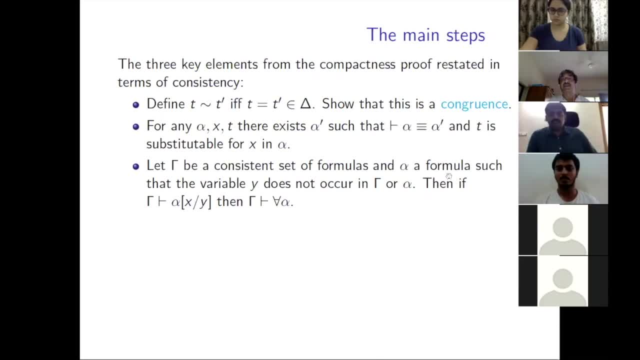 important. if gamma is a consistent set of formulas and alpha is a formula such that you have a variable y which does not occur in gamma or alpha, then if gamma derives alpha with x replaced by y, then gamma derives for all x alpha. yeah, so again the same mess. okay, so this is the 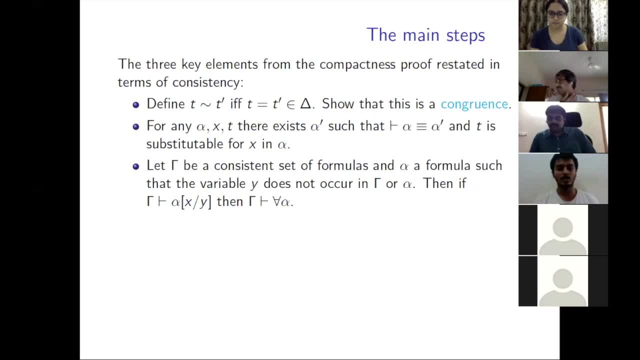 key lemma from: instead of generalization from constants, now you have generalization from new variables, right? this we need to prove, and this again involves some axioms and inference rules. so if you've come up with axioms and inference rules such that we can prove these, i mean pretty much everything is done, all the steps are in place. 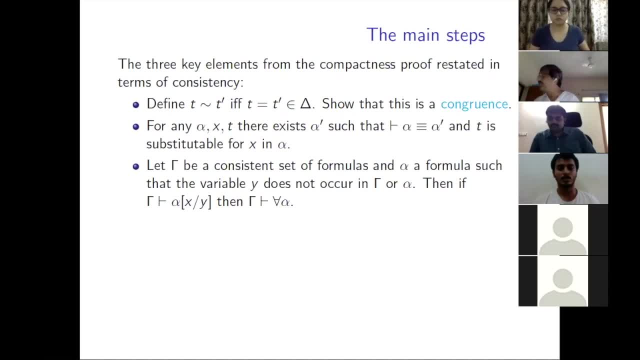 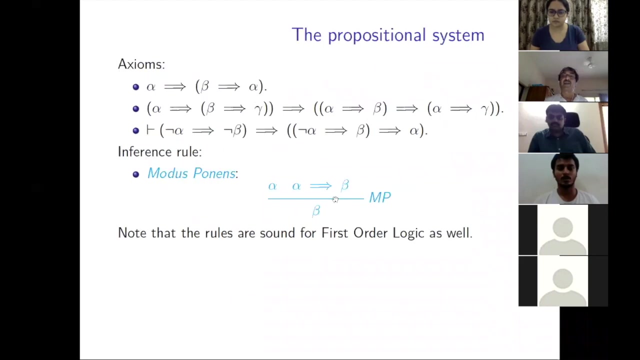 and you can show that the system is complete. this is the main steps of the proof that we're going to go through, so we need axioms and rules to prove. these is the you know proof structure, the idea. clear any questions on this so far, because now we'll start embarking on the actually doing these things. 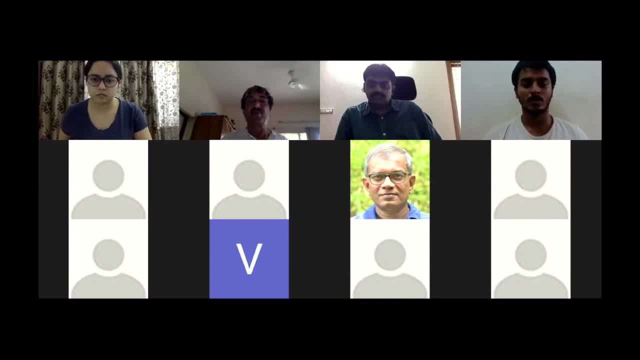 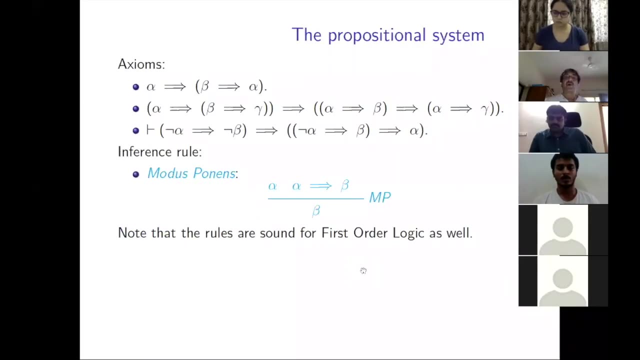 so any questions before that? okay, yes, the Yoga theory is really dramatic, and so we only have a few minutes left with the rule, and the answer is that, for the basic deduction that you've had, you start by writing down the model of the problem and then, when you finish, you start writing down. 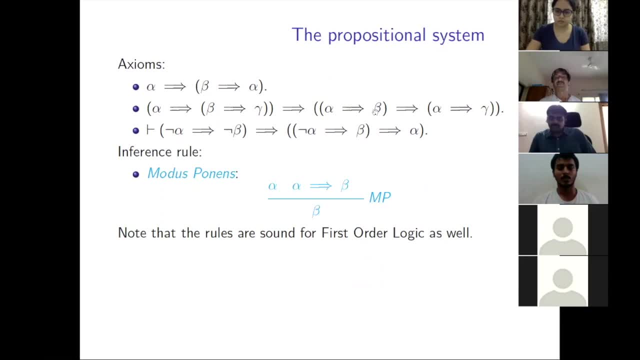 what is the argument for the problem? you can take and you can solve the problem. you can take and solve the problem. you can break down the problem with the problem. you can tell the problem. at this point, if we can get into the basic winners and losers, here we go, yeah, so here's what we came up with, the first one and then the second one. 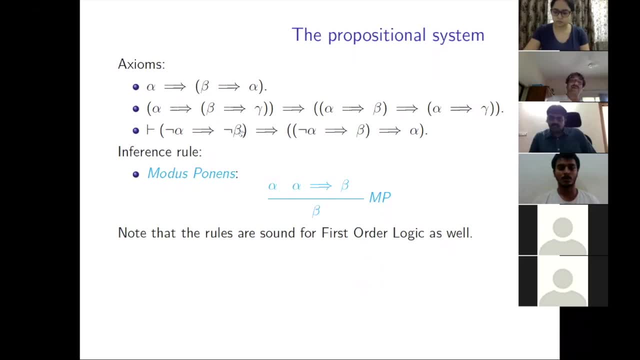 we'll tell you what it was. and it is not a good one, because the first one is the problem. here is the one that you have to solve, and the second one is the idea of what we will do in the next three times. we have to show the error. we might even have to show an argument. 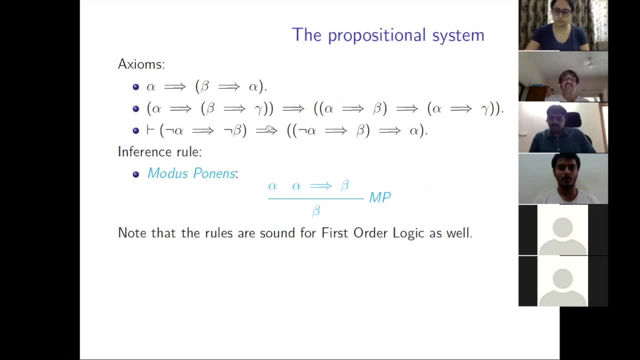 property and you know, with these three, pretty much. so, basically, the you know what you need in the truth lemma that you know a propositional formula, alpha belongs to Delta F, and all this, this takes care of it. and note that these rules are axioms, sorry, the rule. axioms and rules are sound for first order logic. 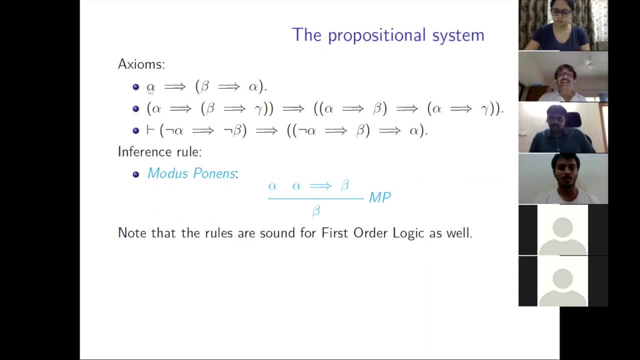 as well, right, by which I mean these alpha beta are schemes. you can substitute any formula earlier, you could substitute any propositional formula, but you can substitute any first order formula here, and still soundness is maintained. that is, this formula is valid even if you put any first order formula. 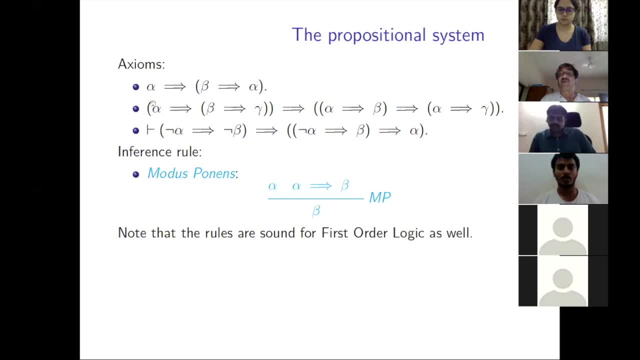 alpha, and that's very easy to see right. take any model M suppose this is not true in that model. that means that model mistake. make alpha true and it must make beta implies alpha false, which means it must make beta true and alpha false. so it makes both alpha true and false. so that's not possible. now this is: 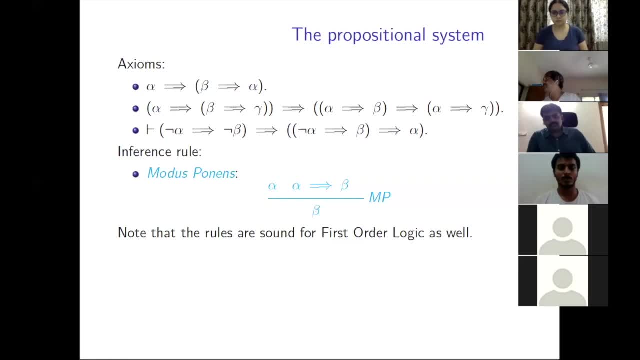 nothing to do with the fact that, whether you are doing first order or propositional logic, right, I mean, the thing is absolutely the same. so as long as you have the classical meaning for negation and implication in your logic, whichever logic that you are talking about, this is. 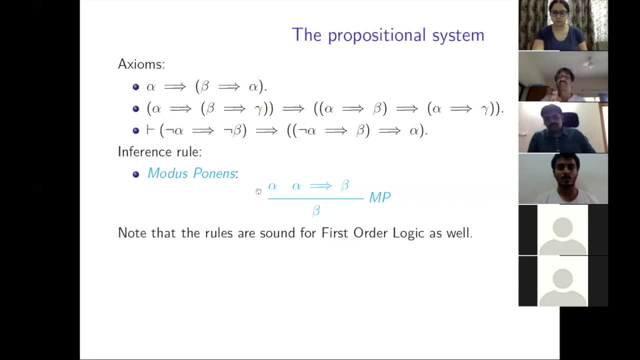 a valid formula, and so this is how you build Hilbert style proof systems that you have something for an underlying logic, and this is where we are using the monotonicity of the consequential relation. remember, the monotonicity of the consequential relation says that if alpha is consequence of gamma, I add more. 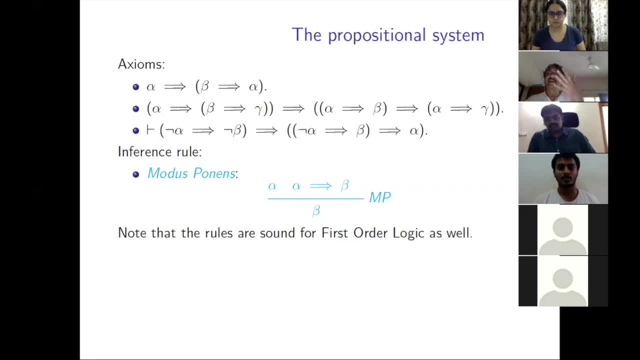 stuff. alpha continues to be a consequence of the logic. so so you can build up conservatively. so we know that our axiom system- I can always keep these axioms and this rule- and at least the propositional fragment of first order logic will work fine, is this? do you understand what I'm trying to say? 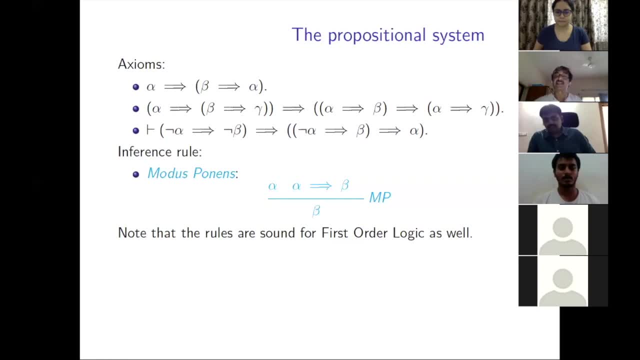 all those things that I proved- properties of consistent sets, properties of consistent and complete sets- everything holds for this logic as well. is this clear? yeah, I mean, there is absolutely no reason for any of them to become false now, because propositional logic is contained in this logic and these are: 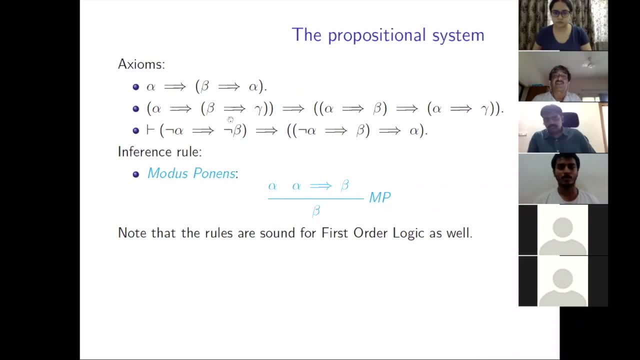 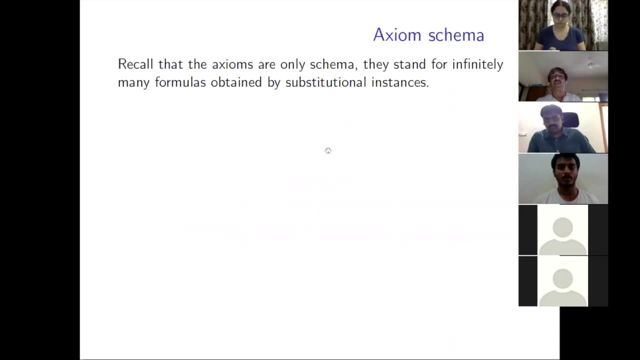 independent of what atomic formulas you have got right, everything else is identical. so the axioms are only schema and they stand for infinitely many formulas obtained by substitutional instances, and the substitution instances are first order formula, for instance what I just said. I mean I can write something of the form. 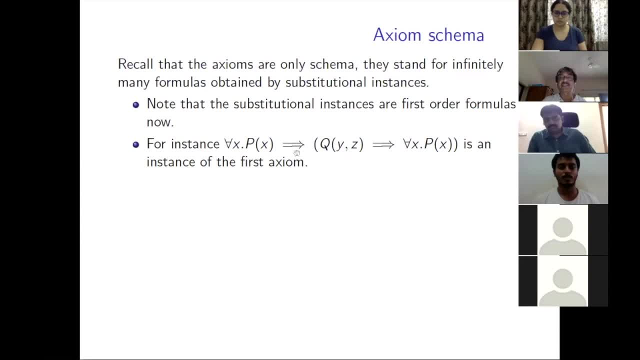 alpha implies beta implies alpha right for all x, P. X implies Q, Y. Z implies for all x, P, H. where this is- and this is an instance of the first axiom and this is valid right now- note that substitutions like this instances may come with three variables. right here is- this is not a sentence- is the formula with three. 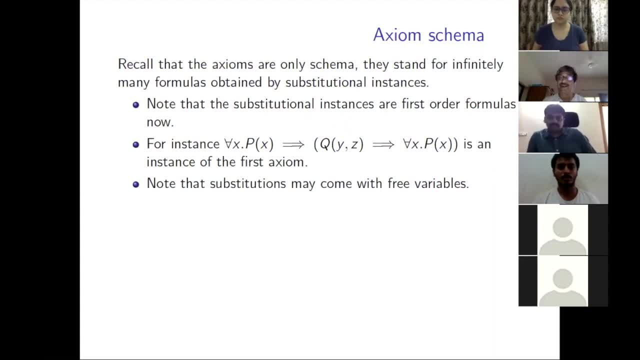 variables, It doesn't matter, It's still valid, right? This continues to be a valid formula. Any model m, it doesn't matter what, whatever assignment of free variables that you've got, it doesn't matter- must make this true right, Because the truth of this formula only depends on the fact that 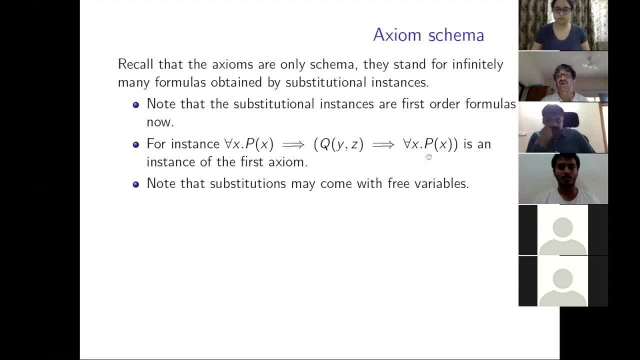 you can't make this for all x p x true as well as for all x p x false. That's all So and this is you know. if you think about it, it's funny stuff, But what is? very simply, 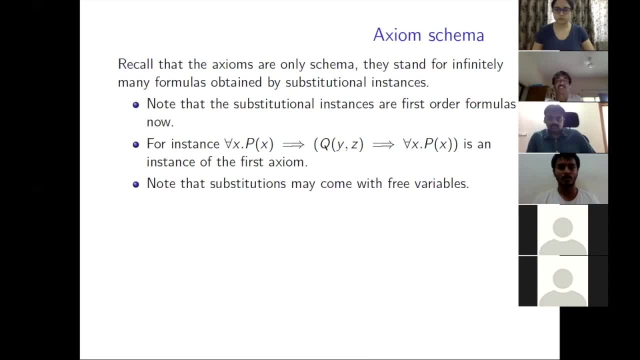 nice is that you can actually conservatively build the whole edifice. So whatever we did goes through like a dream for all the things that we are doing now for first order logic as well. So now, so far, we talked about schema as formulas, and you can substitute whatever. 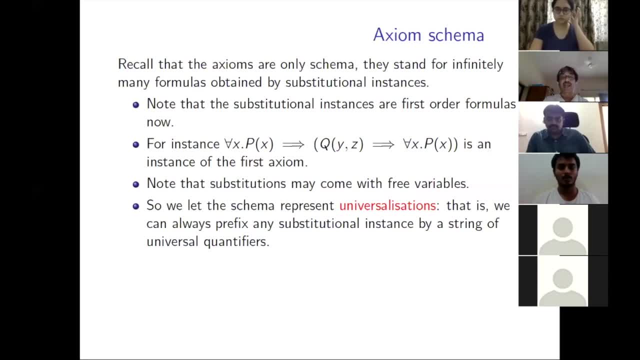 subformulas by formulas. right Now we're going to add one more thing: right, We let the schema represent universalizations. That means like for things like this: right, Q, Y, Z, it's got free variables. Now you can always throw in a for all Y in front of this. 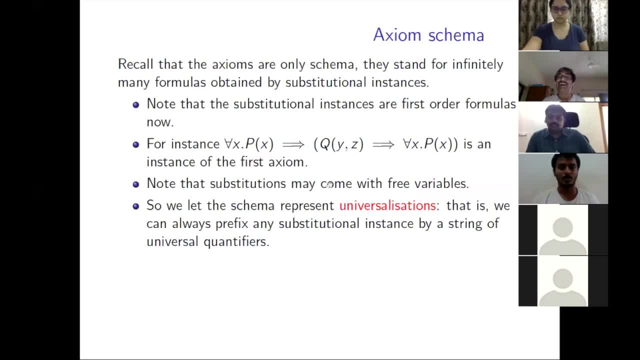 You can always throw in a for all Z in front of this. You know it will continue to be valid right. So we can always prefix any substitutional instance by a string of universal quantifiers, And no problem at all, As long as you always. 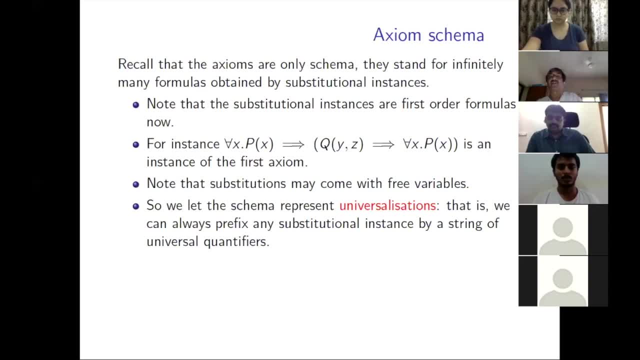 add it as a prefix in the beginning. So this is because if a formula, alpha is valid, for all, X, alpha is valid as well. Do you see that? That's kind of obvious? because suppose alpha is valid, How do I show: for all X alpha is valid? Well, suppose not. Consider a model. 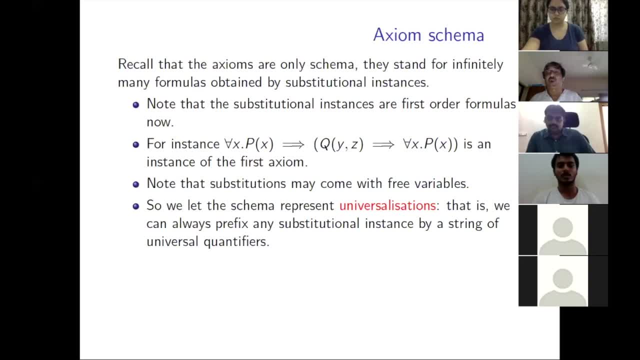 Well, in that model, that model, for all X alpha is not true, right? That means for some choice of element, domain, element D, M with X getting D violates alpha. But then how is alpha valid? Alpha is valid means it's true in all models, right? All models include assignment of elements to free variables. 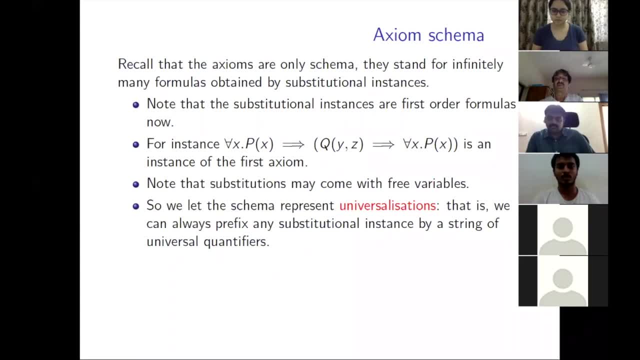 So, therefore, if alpha is valid, surely for all X, alpha is valid. So you can always throw in any number of universal quantifiers as you like, So for instance the universalizations of P, X, Y itself, including the null set. right, You don't need to put it, I'm just saying that if you want, you can. 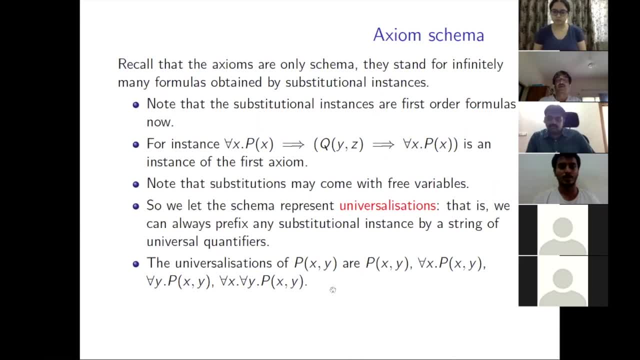 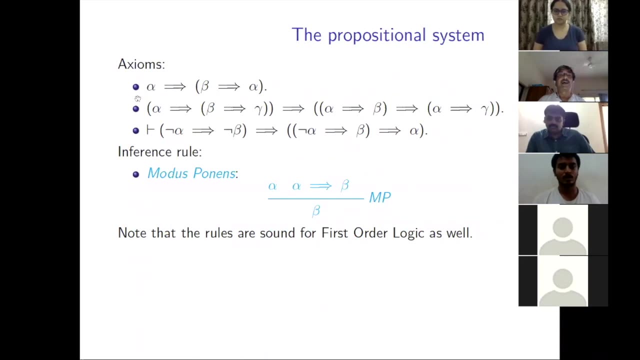 You can put for all X. you can put for all Y, for all X, for all Y, Yeah. So why is this important? It's important in the sense that, when I look at an axiom like this right This axiom represents. 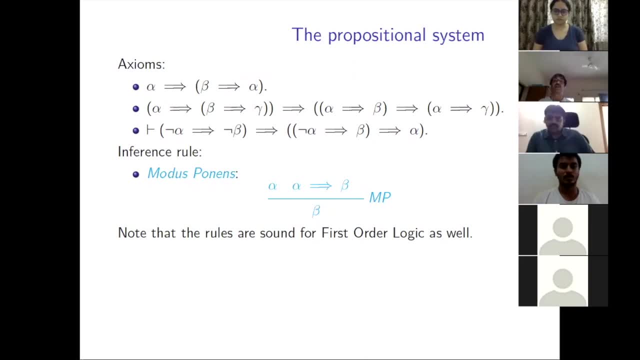 it's a schema that represents infinitely many formulas you can obtain By substituting for alpha, beta, alpha, some sort of formulas, and putting any number of universal quantifiers in the beginning. So notice that suppose Z is a variable that's not used anywhere at all. 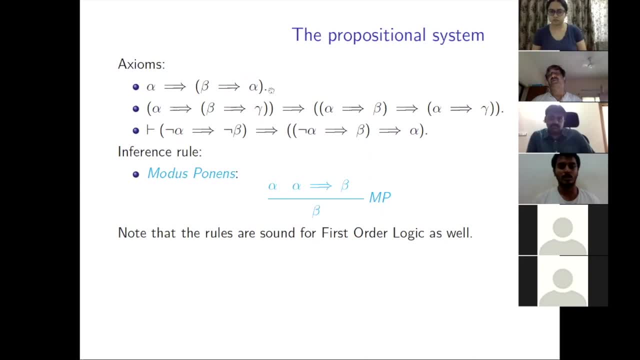 It doesn't hurt to put for all Z in front. So that's the point. So universalizations come for free. You can use it anywhere. So this is something that we'll keep in mind as we go along. Is this clear? 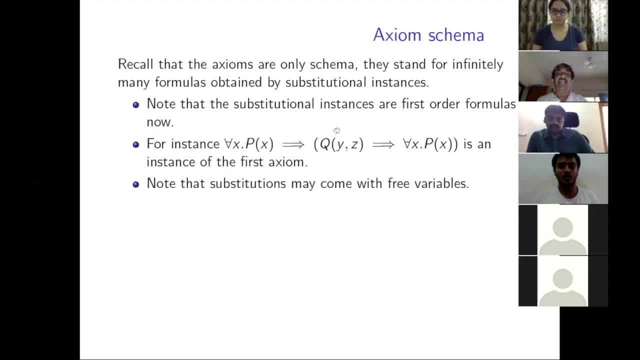 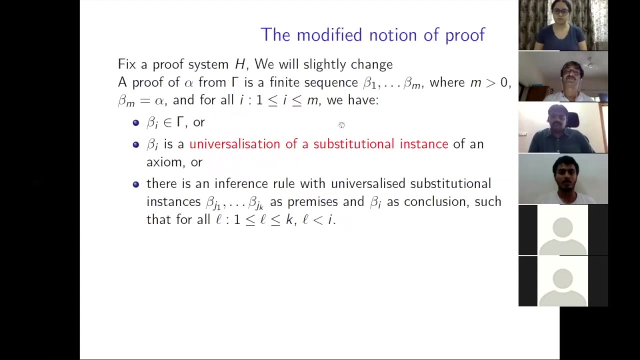 Any question? Yeah, So these are axiom schema in the sense that they are templates for infinitely many formulas obtained by universalized substitutional instances, And so then, accordingly, I have to modify the notion of proof as well. What is the modified notion of proof? Fix your proof system. H. Slightly change the definition. 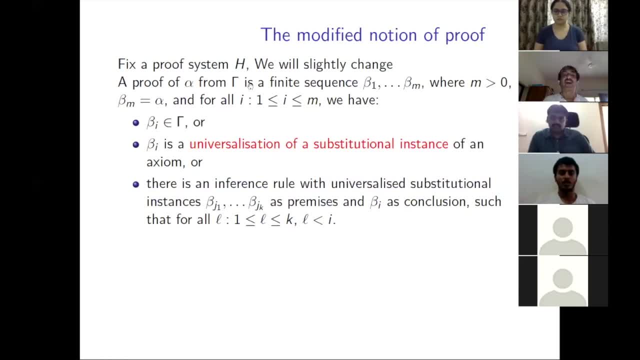 I'm sorry I didn't complete it there. A proof of alpha from gamma is a finite sequence, beta one through beta m. where m is greater than zero, Beta m is alpha And for all i in between we have beta. i belongs to gamma. 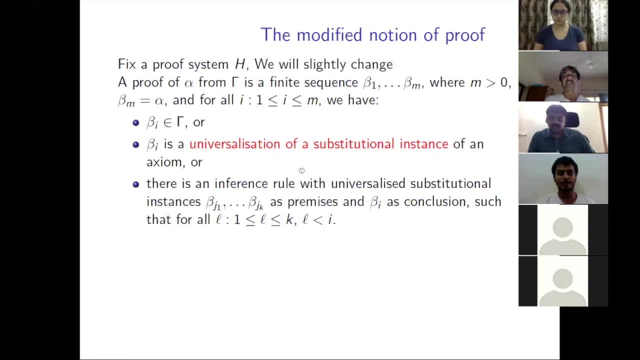 Or beta i is a universalization of a substitutional instance of an axiom, Or you have an inference rule with universalized substitutional instances, beta j one through, beta j k as premises And beta i as conclusion, such that the same problem See that It's again a cut and paste. 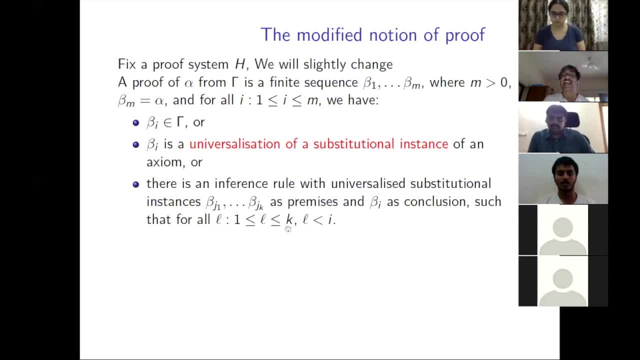 So yeah, So this is not l, but j? l. Right One less than or equal to j? l less than or equal to k? J? l is less than i, So it's basically the same thing, Except that remember that you are allowed universalizations anywhere. 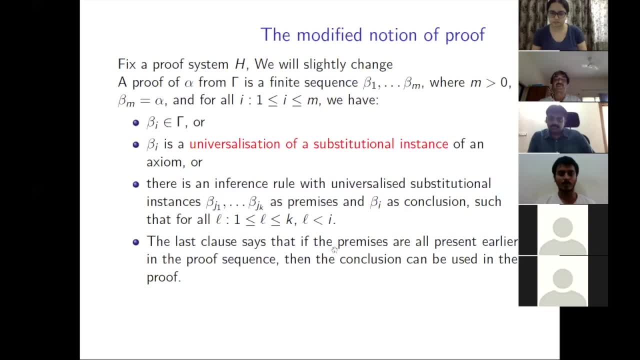 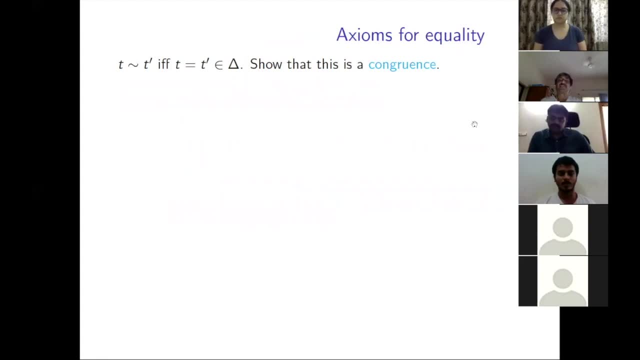 And the last clause says that if the premises are all present earlier- So it's basically the same thing, Except that remember that you are allowed universalizations anywhere in the proof sequence- then the conclusion can be used in the proof. So now let's start with the first step. 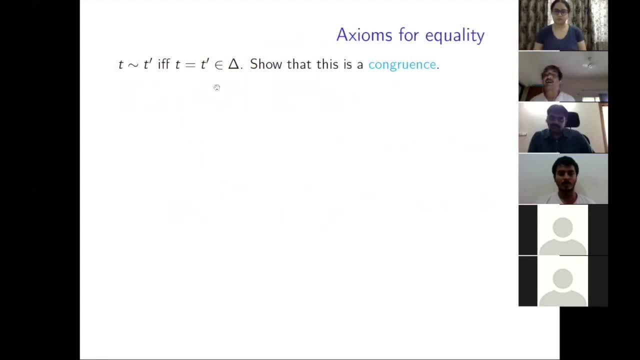 You are going to assume that you have somehow built a set that is consistent, complete and witness-fulfilled. To build a model, anyway, we have to define this relation. We have to show that this is a congruence, Right. 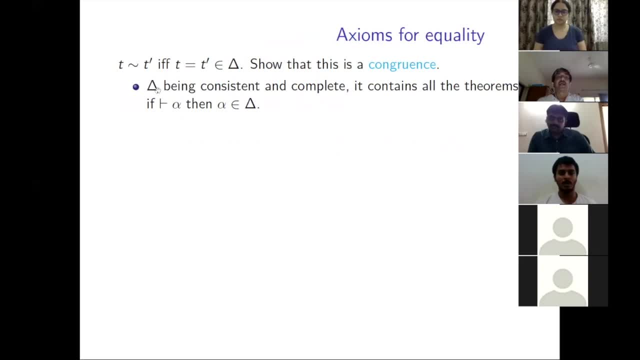 What does this proof involve? Well, delta being consistent and complete, we know that it contains all the theorems. If alpha is derivable from the empty set, it's a theorem right. It's simply a derivation from the axioms and intuitions. 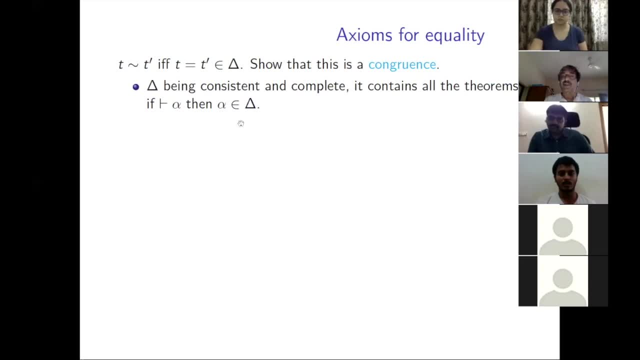 Then alpha must belong to delta, Why It's complete. So if alpha is not in delta negation, alpha belongs to delta. That means delta derives, not alpha. Well, delta derives alpha as well, Because there is a proof of alpha from the empty set. 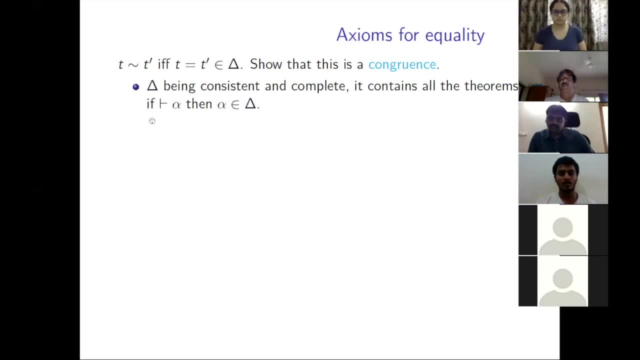 The empty set, therefore, is a proof of alpha from delta as well. So delta derives alpha, Delta derives not alpha. So it's inconsistent, It's not possible. So whenever you have a theorem, alpha must belong to delta. 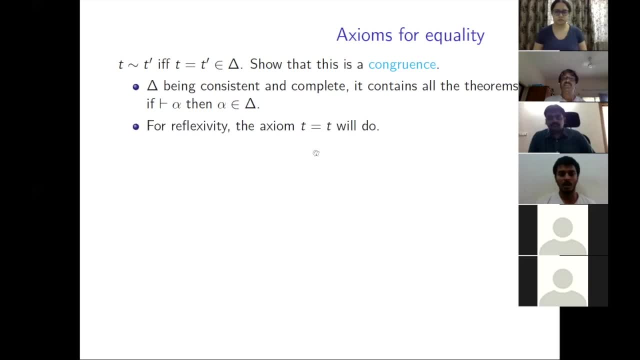 So this is something we can make use of. Well, I want to make sure this is reflexive Right. What does that mean? For every term t, t equals t must be in delta Right, Because we want t is equivalent to t. 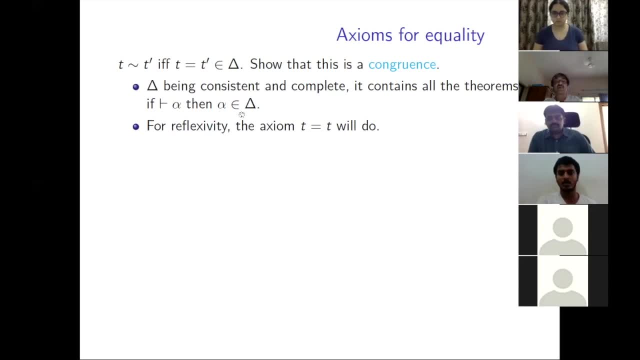 Therefore, t equals t should be in delta. How do I make sure that t equals t belongs to delta? Make sure it's derivable. Well, add an axiom Right. Add an axiom: t equals t. Then it belongs to delta, as we want. 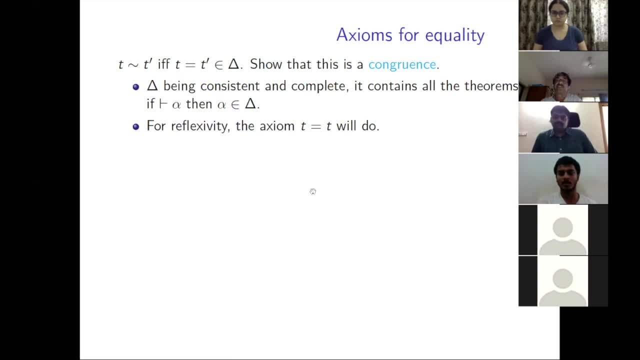 Is it clear. This is the trick, Right? So we are going to use. this is what we want, and we keep adding axioms to make this go through. So reflexivity says I must have an axiom. T equals t. What about symmetry? 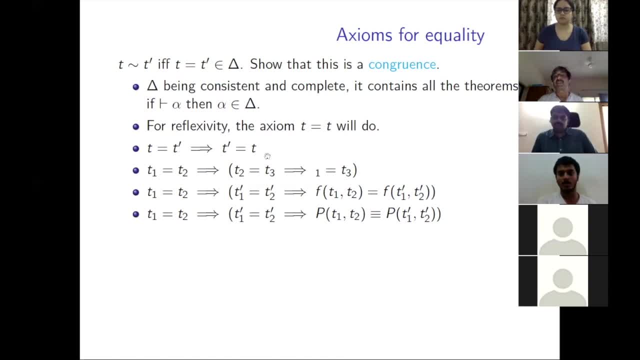 Well, t equals t prime implies t prime equals t, Right? So if suppose t, we want to show that this relation is symmetric, Right? So suppose you have got t's till the t prime and t prime till the t. 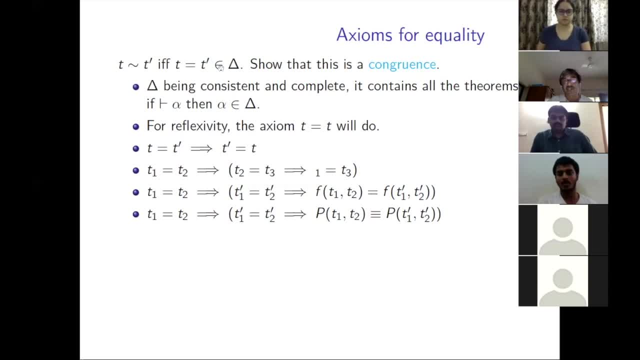 I mean, suppose you have got t till the t prime, Then you know that t equals t prime belongs to delta. Since this is in delta and this in alpha implies t, Alpha implies beta, Then this is in delta as well. So t prime equals t is in delta. 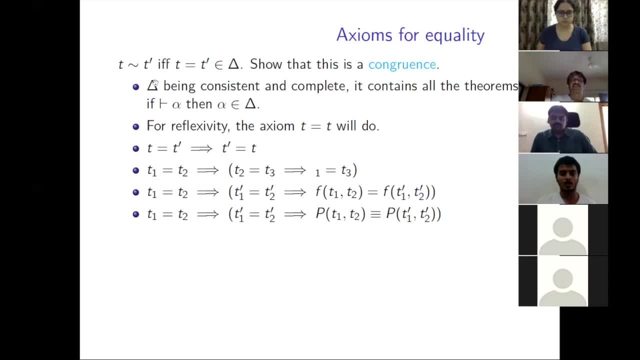 Therefore, t prime is equivalent to t. So therefore, this relation is symmetric. This is it, So this is. if you have this as an axiom, symmetry will go through. Now, if I have this as an axiom: t1 equals t2 implies t2 equals t3 implies that's t1 equals t3.. 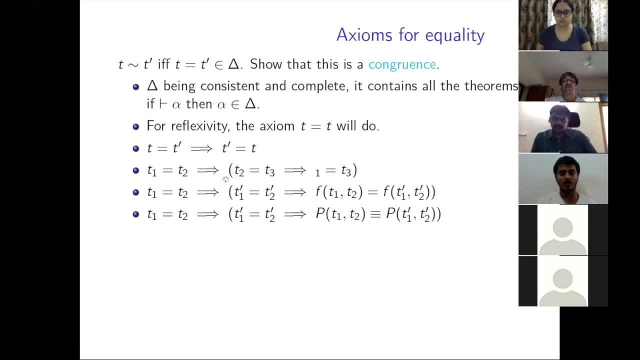 Yeah, This will ensure that this relation is transitive. Why? Because if t1 is t1 till p2 and t2 till t3 are given, then you know that t1 equals t2 belongs to delta. Therefore, this implication belongs to delta. 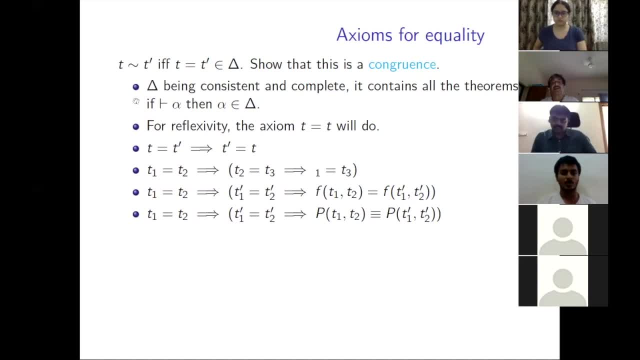 t2 equals t3 belongs to delta. Therefore, t1 equals t3 belongs to delta. So axioms of this kind is what we are looking for Now. I have written this for a binary function symbol, a binary predicate symbol. 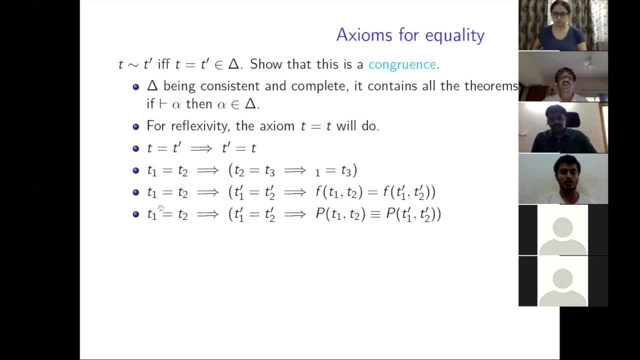 But in general you have to have this for k Right? So you have to have: if t1 equals t2 and t1 prime equals t2, prime f of t1, t2 equals f of t1 prime And here p, t1, t2 is equivalent to p. 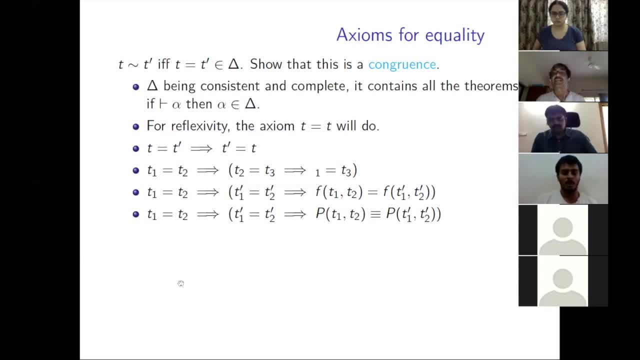 So this kind of thing. So if you have axioms of this kind, you can prove that in fact that is a congruence And then use that to quotient the domain set of all terms and build your term. 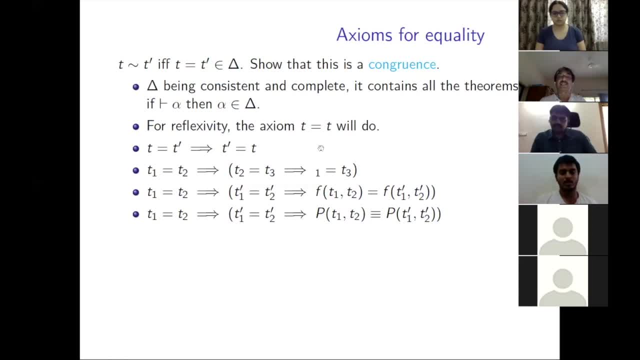 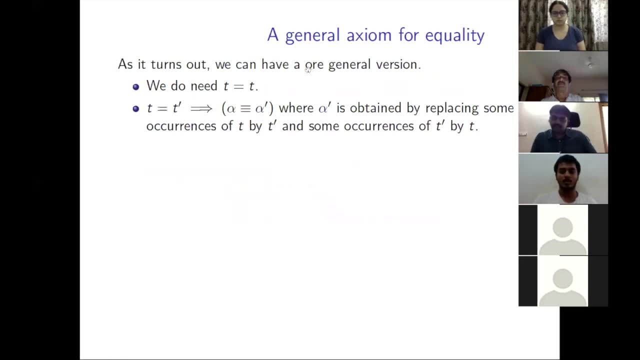 So the first step can be done if you have these axioms for equality. So, as it turns out, we can have a more general, more typos, more general version. We do need t equals t And then you have a single axiom which is t equals t. prime implies alpha is equivalent to alpha prime. 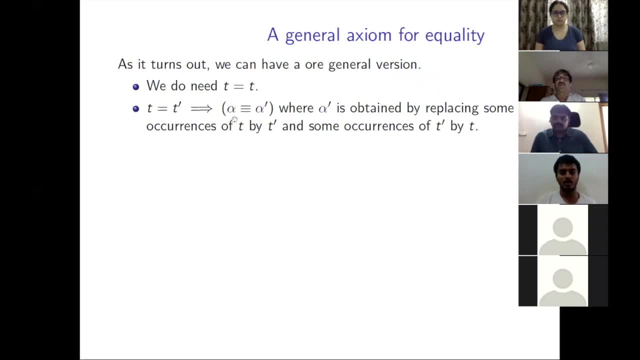 where alpha prime is obtained from alpha by replacing some occurrences of t by t prime, some occurrence of t prime by t Right. Basically you have taken this formula: alpha. I know that t equals t prime, So go in that context. 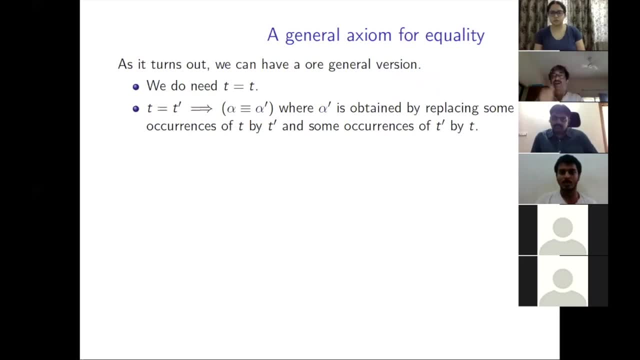 Doesn't matter what it says. If you take t and replace by t prime, there's no problem. If t prime occurs in alpha, replace it by t, no problem, It continues to be logically equivalent. Now, this is the principle of substitution of equivalence in expressions inside equations. 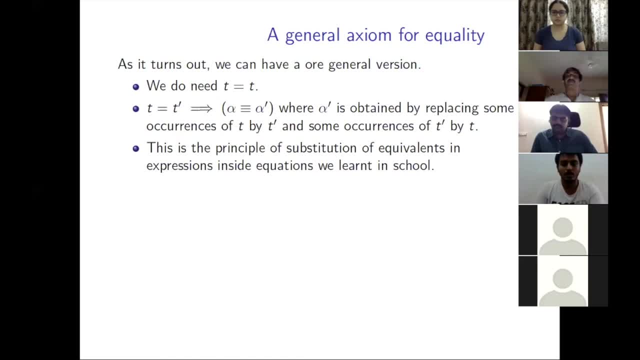 that we have learned. We learned in school. Right, When you have- you know- trigonometric identities, you have these complicated expressions or algebraic expressions. It doesn't matter where you are. Somewhere it says x squared plus y squared plus 2xy. 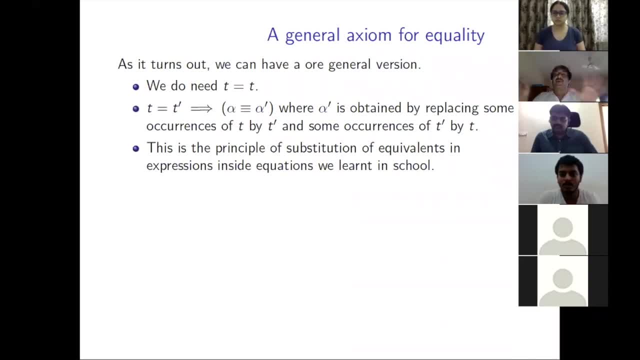 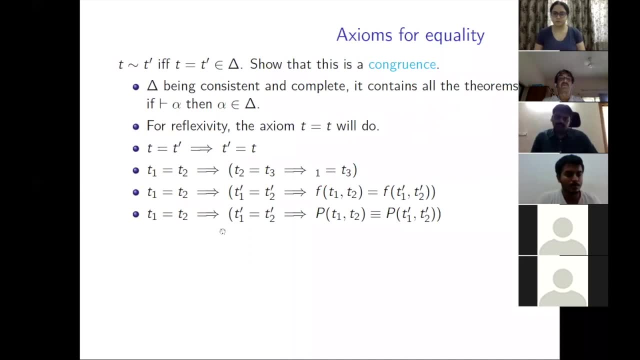 I can always replace it by x plus y, whole squared. And here you know this kind of thing that we have done many, many times. Right, And that's all that this is, And note that this is different from uniform substitution. 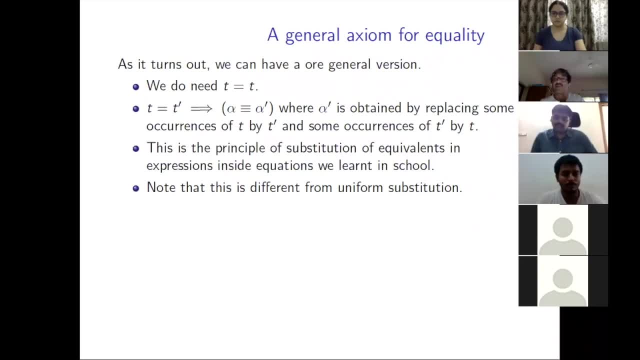 I'm not saying that you uniformly substitute wherever t occurs by t prime, Right? You can choose to replace it in one part and ignore it in another part, Doesn't matter, Right? And I mean you have x plus 8 coming here. 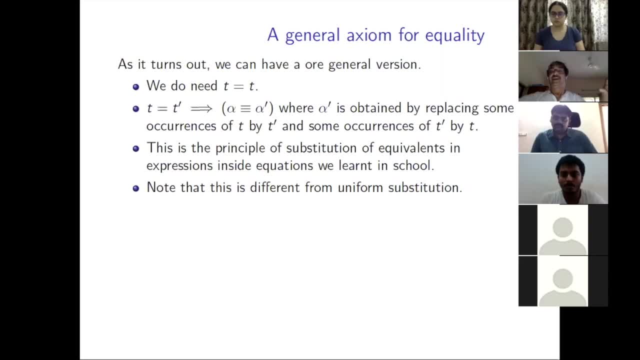 One place you might replace it by x plus 5 plus 3.. Another place, you might replace it by x plus 12 minus 4. Doesn't matter, You know. And now you have to show that this is sound, And once it is, that means it's a valid scheme for every formula alpha. 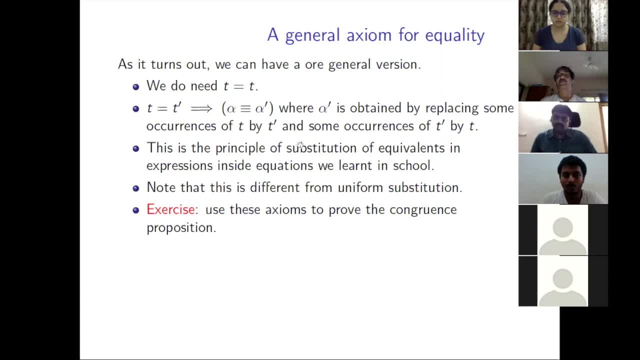 And then you can use it to prove the congruence proposition Right, That all these are derivatives. Transitivity, symmetry, congruence with respect to function symbols, predicate symbols, all these can be. That's natural. Yeah, F of t1, e of t2 equals f. 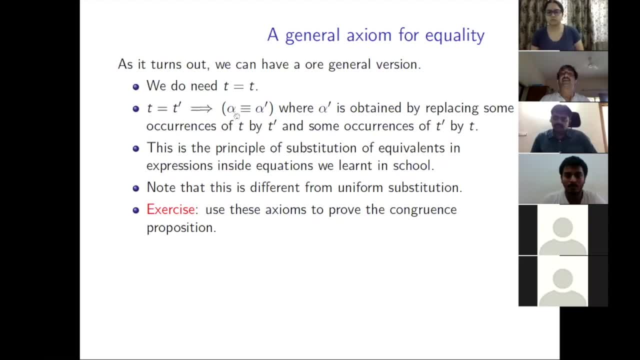 That's a formula, Right. It's a method of replacing And similarly predicates symbols. Yeah, So is this clear? So this is the first step in our completeness proof, And this is something that goes through easily. Any questions about the first step? 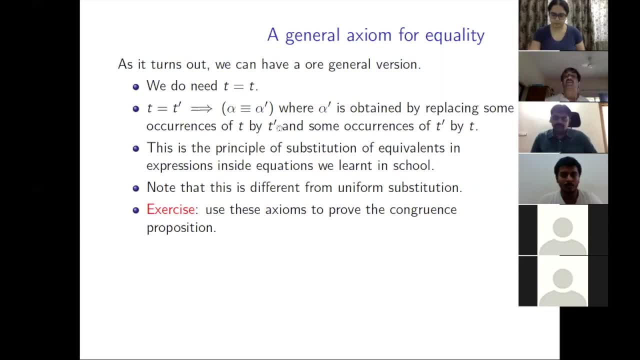 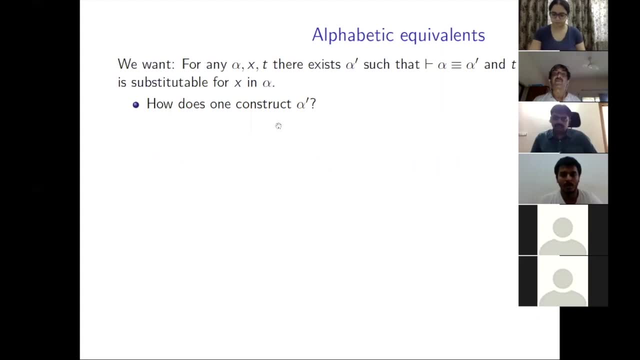 So, once you have the axioms for equality, the first step of showing congruence is something we know how to do. Okay, Let's get to the second, And this is the thing about alphabetic equivalence, as they are called. 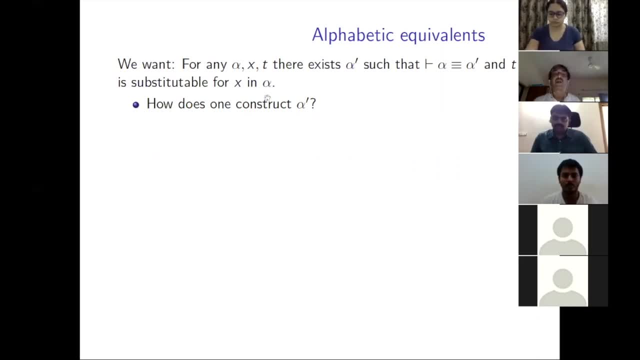 Alphabetic variance. I think we call them. What is it we want? For any alpha, x, t, there exists a term, there exists alpha prime, such that alpha is equivalent to alpha prime and t is substitutable for x in alpha prime. 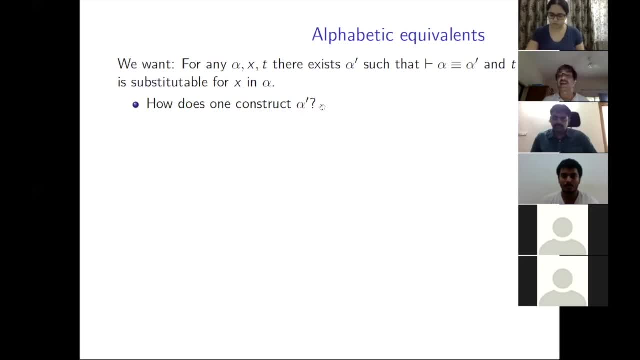 This is alpha prime here. Now how does one construct alpha prime? Remember what is the problem? You are given a formula, alpha, a variable x and a term t. In general, t may not be substitutable for x in alpha. 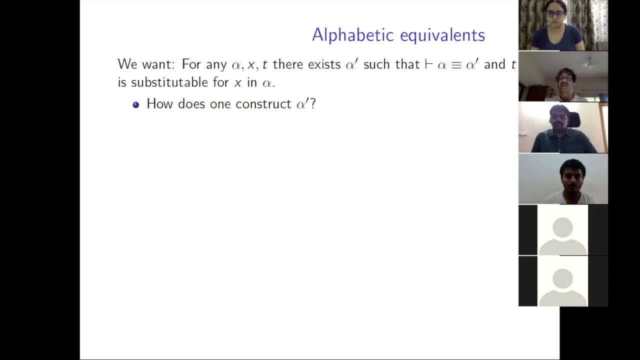 And you want to construct a formula, alpha prime, which is logically equivalent, but t is substitutable for x in t. How does one do that? By bound variable renaming Right. Rename all the variables in t having bound occurrences in alpha. Remember those are the ones that clash. 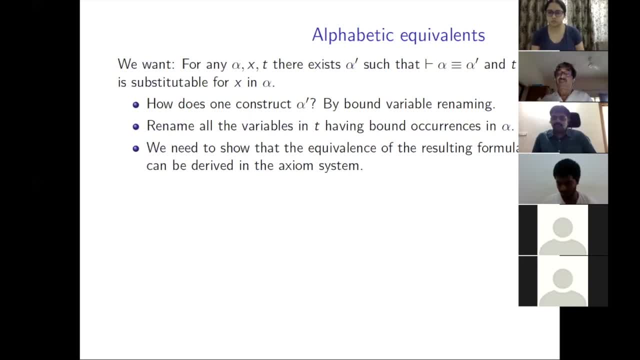 You look at the term t, it's got some variables. Those variables have bound occurrences in alpha. you know that they create problems, Right. So what we want to do is to take those variables and rename them with an alpha. That will give you alpha prime. 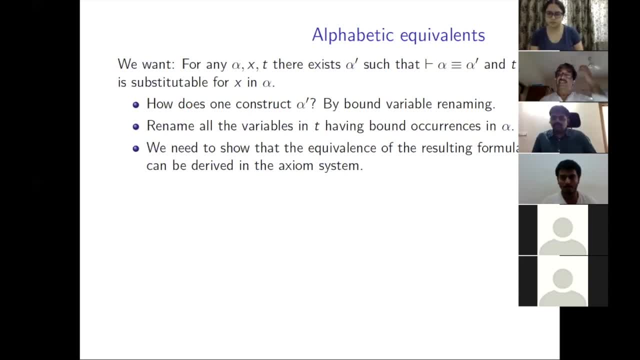 And once you have renamed them, there is no clash and t is substitutable for x in alpha. That's all. So we need to show that the equivalence of the resulting formula can be derived in the axiom system. Right, This is the critical part. 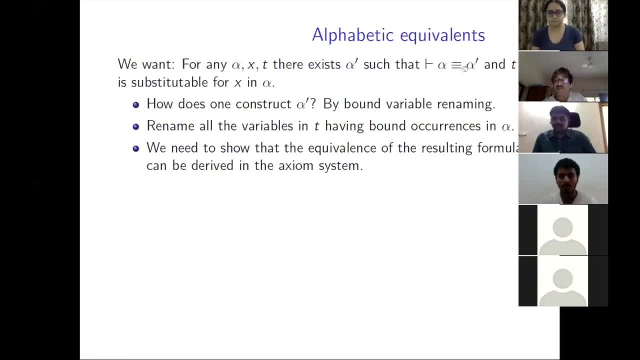 It's not just that it's logically equivalent semantically, but I should be able to derive that these are equivalent. So if you think about it, it suffices to show that basically, bound variable renaming is okay. That is, for all x alpha is equivalent to for all y alpha, with x replaced by y where y is a new variable. 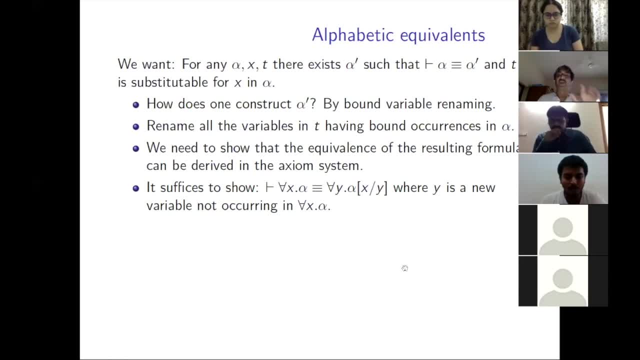 not occurring on the left-hand side. Right, If you take a formula of the form for all x alpha, find a variable y. Right, It's a bound variable. x is a bound variable, So you rename it by another variable, y, with replacement inside here. 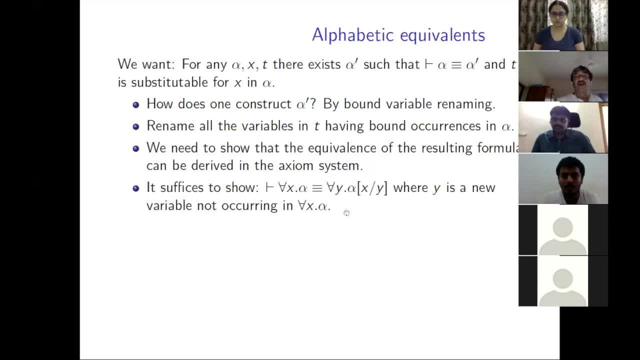 This is the bound variable, And y is a new variable, not? And? once you have this, this is all you will need for alpha prime. Systematically keep doing one after the other And you will get your alpha prime, And at every step you are preserving logical equivalence and 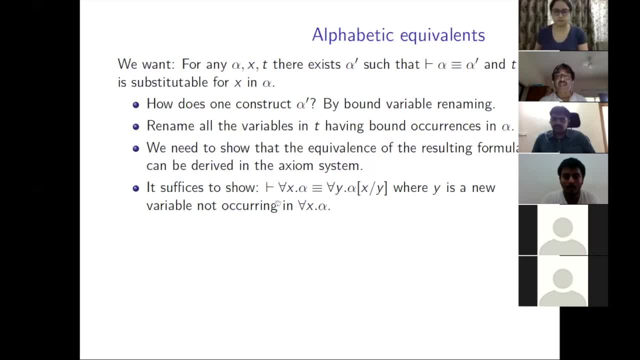 So this is all you need to do, But to make this derivable you will need some axioms, Clearly Right. Why else would this be derivable? Because from the propositional part you can't derive this. From the equality rules you can't derive this. 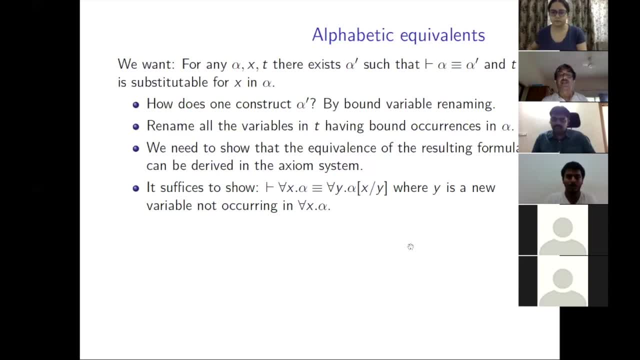 So you need some new axioms. So what are the axioms that you will add to make this go through? And it's amazingly simple, And but something that requires the quantifier axioms. So what is it that we want? 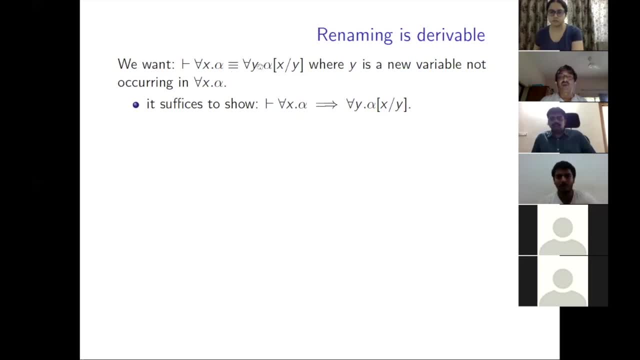 We want for all x alpha is equivalent to for all y alpha, with x replaced by y, Whereas I said y is a new variable, not Actually, I claim that one direction is all, that we need The other direction. how will you prove? 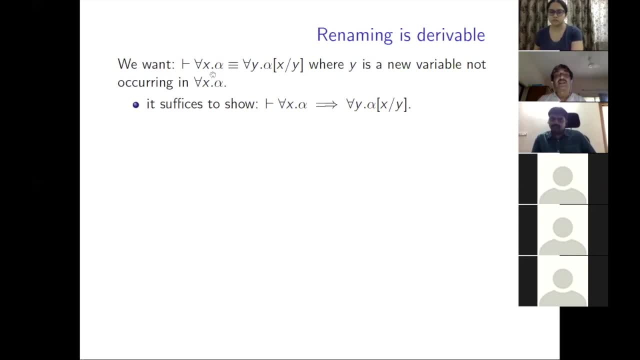 I'm saying it suffices to prove that the left-hand side implies the right-hand side. What about? the right-hand side implies the left-hand side. Why don't I need to prove that Anybody? Is the question clear? I claim that it suffices to. 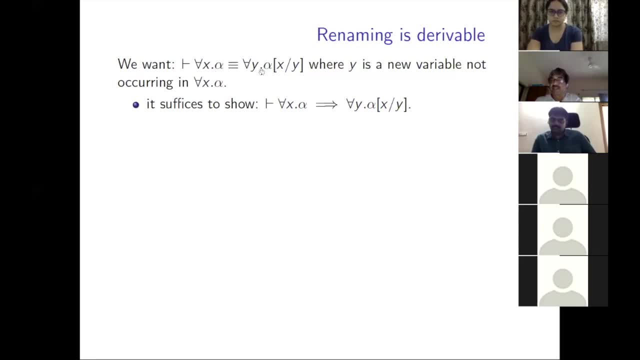 We need to prove the equivalence right. You have to prove left-hand side implies right-hand side and right-hand side implies left-hand side. My claim is that the only non-trivial part is left-hand side implies right-hand side. Why? Okay, look at this. 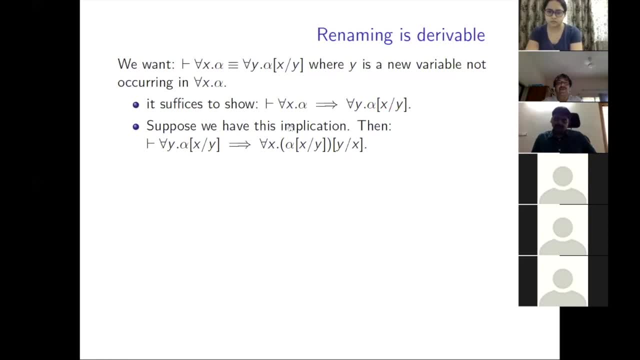 Suppose we have this implication, Then what about for all y alpha, with x replaced by y? Consider this here, right This? Now, if I look at this formula, x doesn't occur anywhere here. Why? Because x has been replaced already. 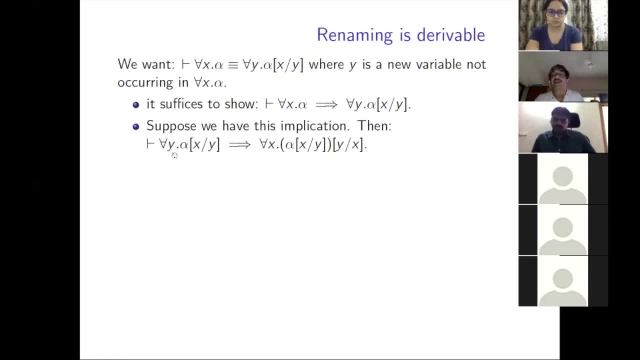 Right, y is not equal to x. That's a new thing. So, and I have replaced this. So x doesn't occur anywhere, So I can use this theorem that I have proved. So what will I get? I will get, instead of y, I have x. 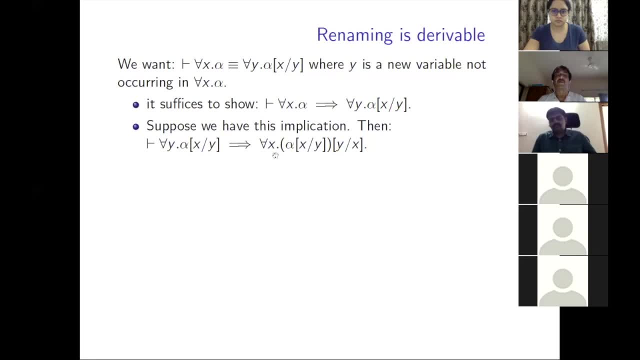 Instead of that, I have y here And some formula, So I can always write formula. So I can always write for all x This formula from the left-hand side, with the replacement that I am doing here. Is this clear? 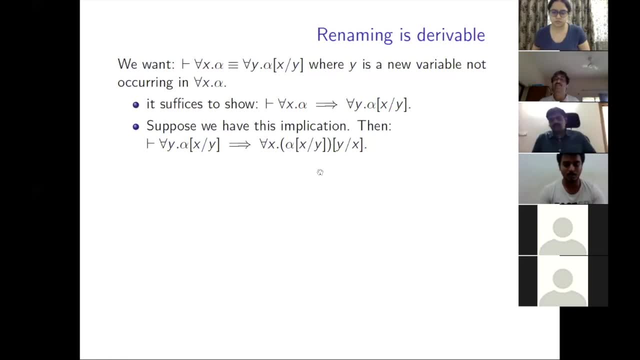 This is simply a substitutional instance. now, Suppose I have proved this implication, I just apply the same one substitution for this. What is that? Instead of x, I put y. Instead of alpha, I put alpha, with x replaced by y. 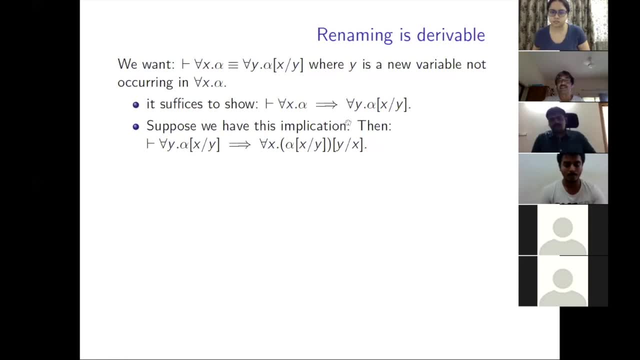 And then, on the right-hand side, I consider Instead of y, I consider x. So what should I get? This is the left-hand side alpha, with x replaced by y. The left-hand side is this formula, with y replaced by x. 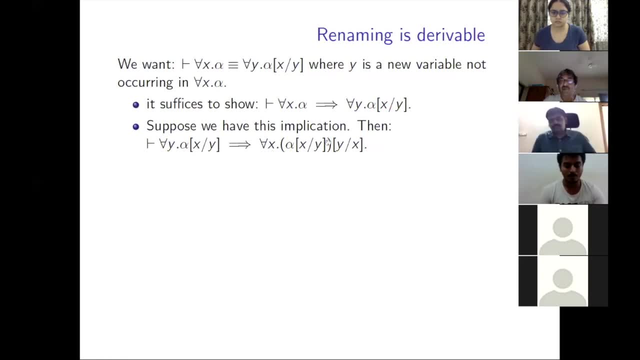 But now you look at this. What is this? This is a for all x formula, with this, with a substitution, But that is the same as But alpha with x replaced by y, in which y is replaced by x, is the same as alpha. 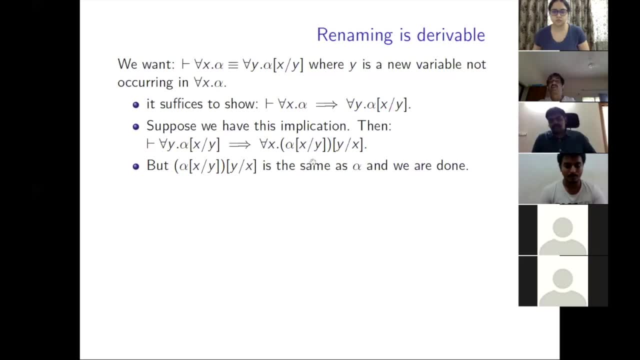 So therefore, what you have got is for all x alpha. So if you prove left-hand side implies right-hand side, automatically you also get right-hand side. So we are done. I hope you. There is no magic in this. 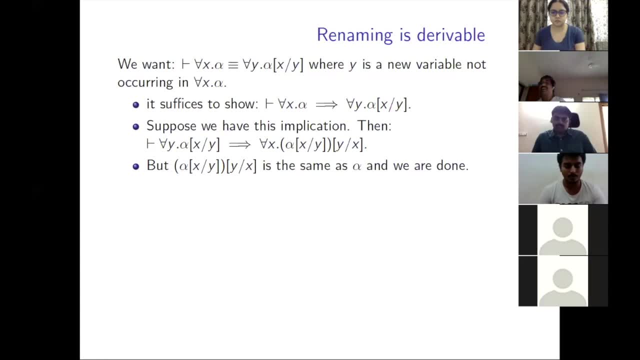 It is just, I mean bound variable renaming. The point is that it does not matter which direction you look at it: Bound variable is bound variable, New variable is new variable. So, and this is something that we need- some work We want. 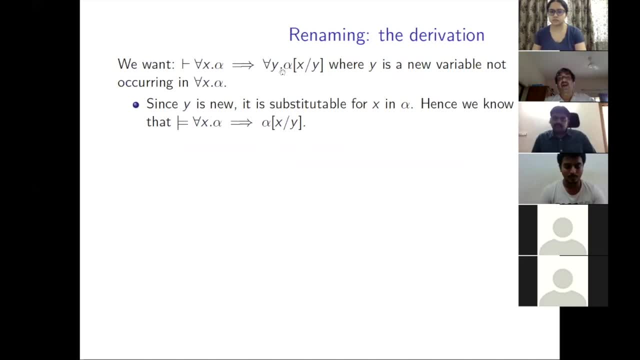 For all x alpha. For all x alpha implies for all y alpha, with x replaced by y, where y is a new variable. Now notice that y is a new variable, Right? So it is substitutable for x and alpha. Remember one of those painful exercises I gave in problem set 1, 2, part 2 or whatever I forgot to know? 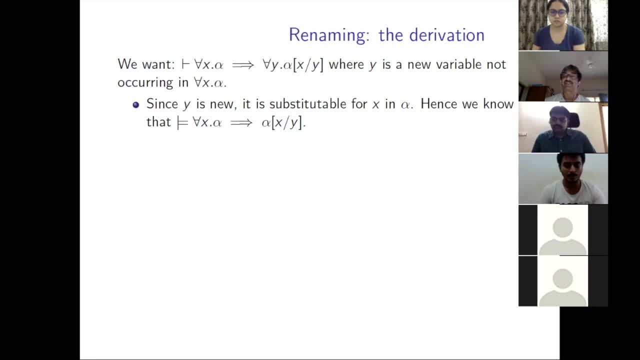 Is to talk about. when is x substitutable for t? t is substitutable for x, Right, A new variable is always substitutable, So there is no issue at all. So we know that this is a valid formula For all. x alpha implies alpha. with x replaced by y is a valid formula. 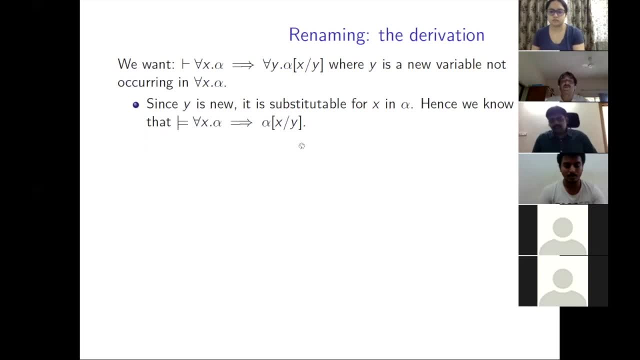 Right. One of the earlier arguments that we gave was: if t is a term substitutable for x and alpha For all, x, alpha implies this is a valid formula. Hence I can always add this as an axiom: Right, Once it is a valid formula. 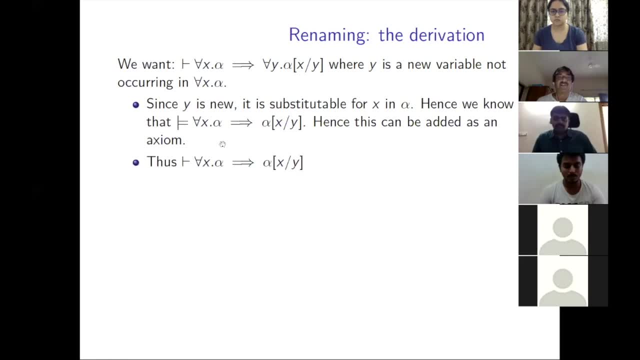 I am allowed to add it as an axiom. So therefore this is derivable, Right? So for all x. alpha implies alpha, with x replaced by y. I will get like this. The trouble is, I want a for all y. How do I get a for all y now? 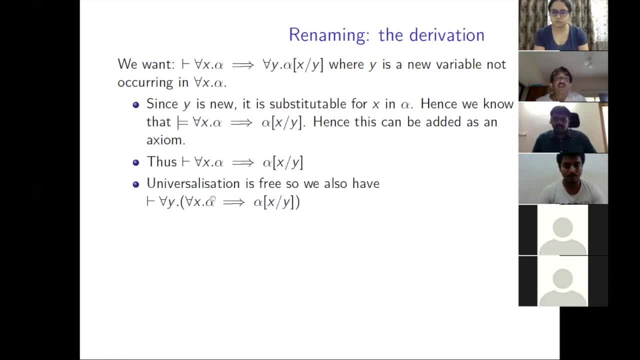 There is no for all y here. Well, remember that universalization is for free Right. Whenever you have something derivable In proofs, You can always throw in universalizations Right. So once you have this implication, we also have for all y this implication. 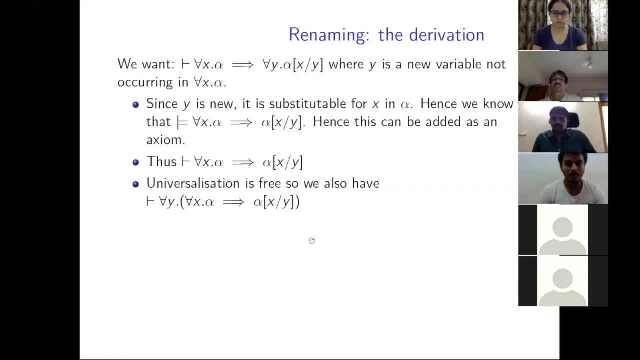 Yeah, If this is derivable, so is this. But now, if somehow we could distribute for all over implication, Right, We would get All y for all x. alpha implies the right hand side that we want, Right. But so why should we be able to distribute the universal quantifier over implication? 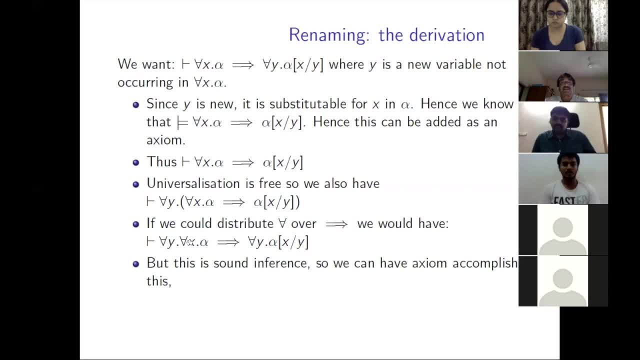 Well, this is sound inference. Whenever you have this valid, this is valid as well, So we can have an axiom to accomplish this. Yeah, And finally, for all x alpha. Now, this still doesn't do the job. We need to somehow link for all x to this. 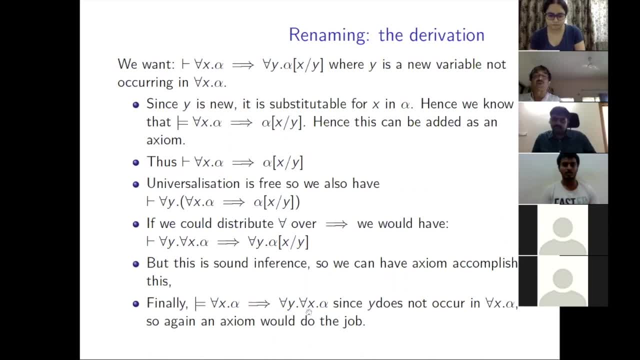 Well, for all x alpha implies for all y, for all x alpha. Why, Remember, y does not occur free on the left hand side. Yeah Right, This is really of the form. beta implies for all y beta. Well, that makes sense. 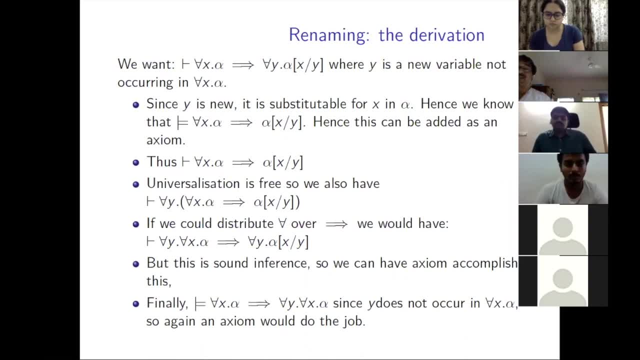 Because y does not occur at all in it, Right, Why does not occur in beta? Beta, of course, implies for all y beta. So one more axiom will do the job. So I need an axiom of this kind. What is this kind? 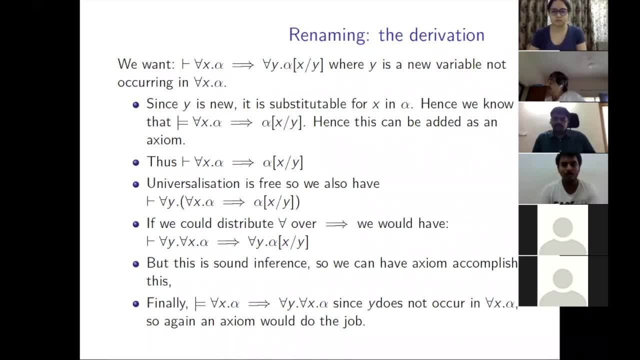 It says that for all from, for all x alpha, I can get alpha with x replaced by t, That t is a substitutable. I need an axiom to say: beta implies for all y beta If y doesn't occur in beta. In fact y does not occur free in beta. 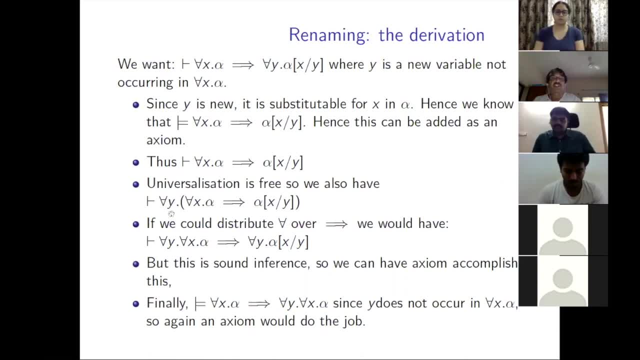 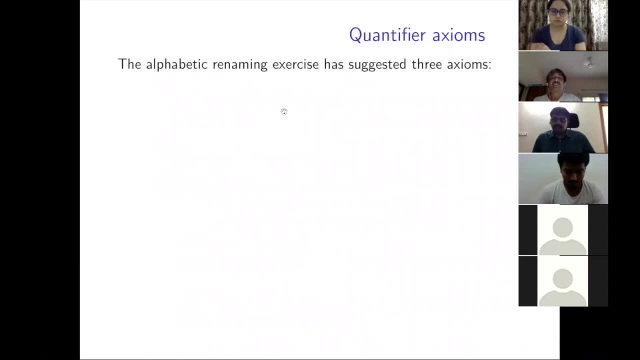 And we need somehow to distribute universal quantifier over implications. And these are exactly the quantifier axioms. So this alphabetic renaming exercise suggests three axioms, And the first axiom is: for all x. alpha implies alpha, with x replaced by t. 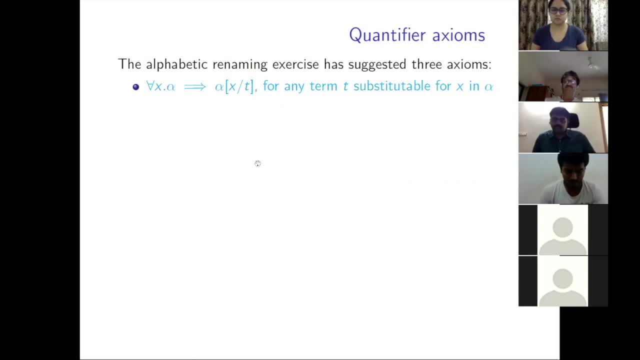 For any term, t substitutable for x alpha. Alpha implies for all x alpha, where x is not a free variable of alpha. If it occurs bound, who cares? Right, It occurs free. That's a problem, Of course. Right? If you have x equal to 3, it doesn't mean for all x. x equals 3.. 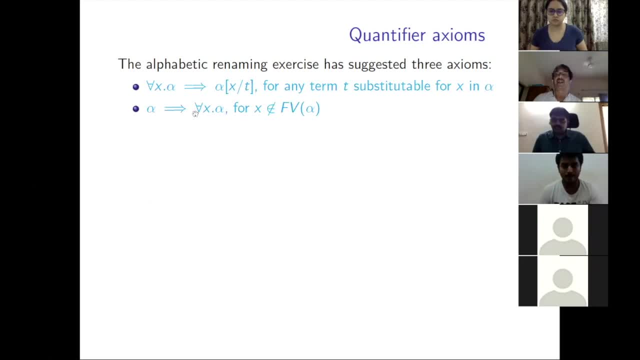 Right? So if it's a free variable, we can't do this, But If it's not a free variable, who cares? Right? So if alpha is true, Then Yeah, So this is a valid formula. 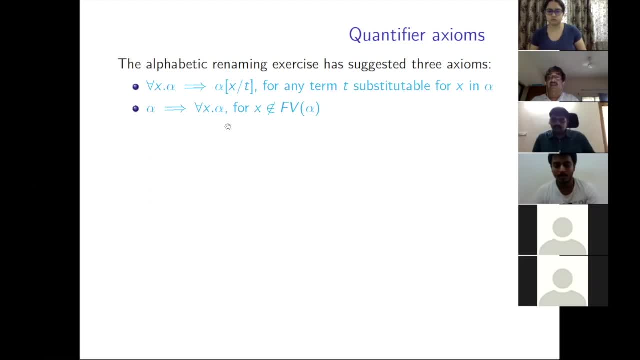 And this validity is very important. Again, How do you show that this is a valid formula? Take any model M, Suppose it violates this. That means that the model satisfies alpha, But the model doesn't satisfy for all x alpha, Right? 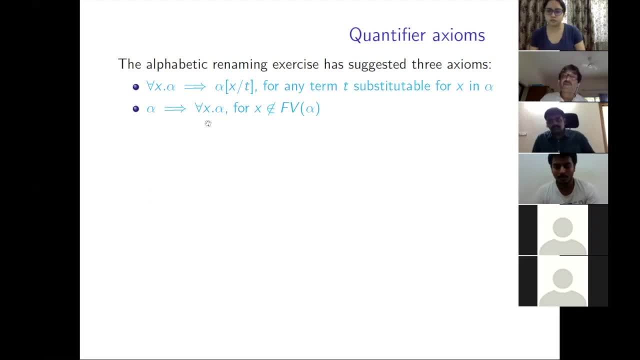 Okay, But remember that the model satisfies alpha And we have already shown that. Yes, What have we shown? The truth of a formula in a model depends only on the free variables assignment. Right Assignment to free variables x is not among the free variables. 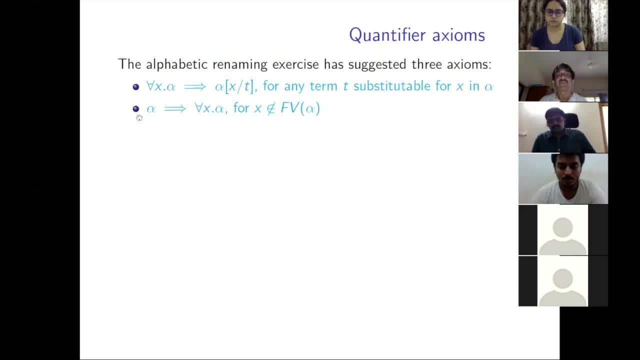 So it doesn't matter what is the decision made for x here. So here, If it's violated For some domain, element d, It's not matter. These are two models, m and m prime, That agree on all the free variables of alpha. 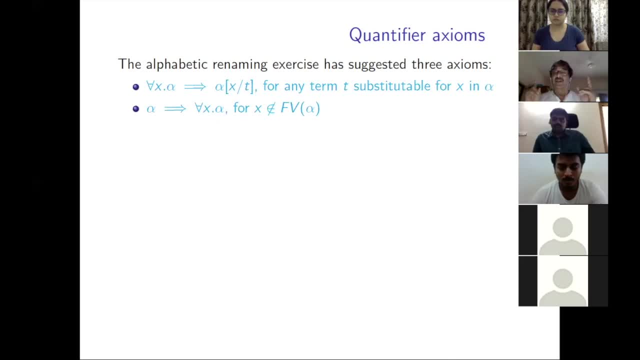 Then They must both make it true or make it false. You remember, one of the earliest propositions we proved Was that If two models Given a formula alpha, If two models Agree on, I mean based on the same interpretation, Same structure. 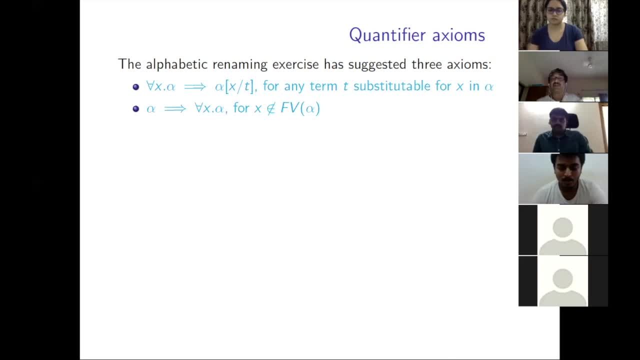 Yeah, Underlying structure is the same. If they agree on the free variables, They must agree on the formula Right. So Since Alpha doesn't occur free in this, Then If these two models agree on them, They must. 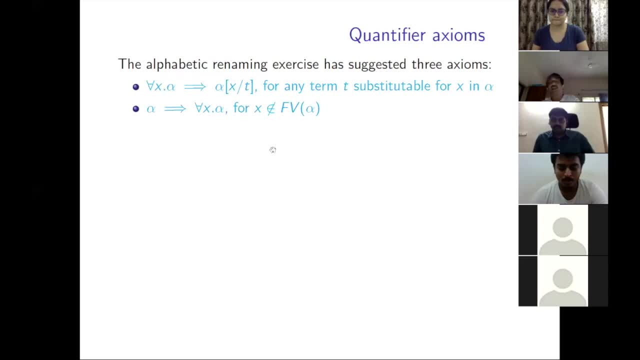 So Please go through the proof of the Validity of this formula To make sure that you understand. And the third one is the distributivity of Universal quantifier over implication. It says: For all x, alpha implies beta. For all x, alpha implies for all x. 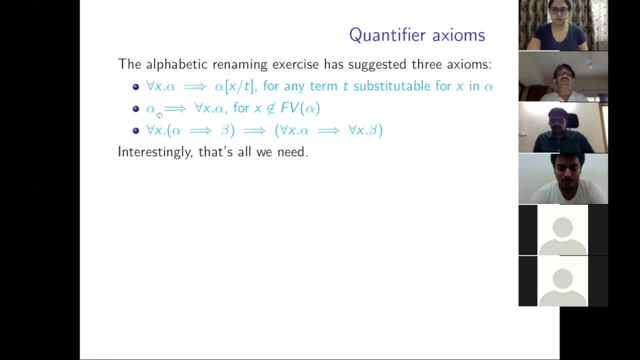 And this is a very reasonable one, And this is reminiscent of. If you look at these two, Does it remind you of the Hilbert axioms For propositional logic? What was the First axiom for propositional logic? Beta implies alpha implies beta. 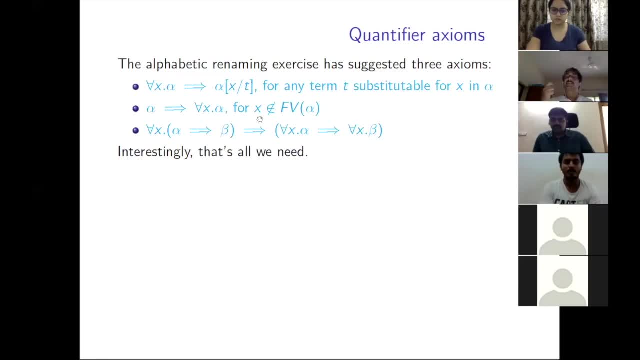 So this is Roughly similar in structure. In the There is a notion of combinators from this. It's very similar. And then this one says, If you remember, Alpha implies, Beta implies, Gamma implies Alpha implies, Beta implies. 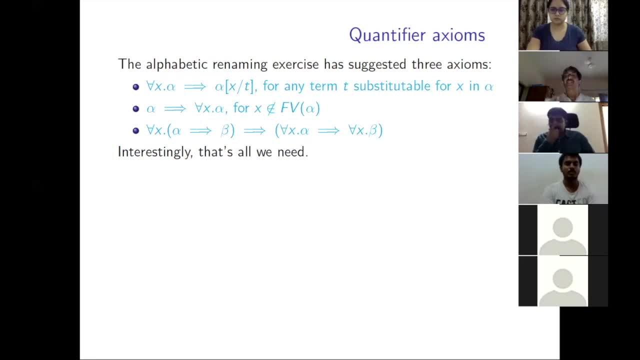 Gamma implies, So that That Implication distributes. So Similar thing is being said here. So, Hilbert, axioms Always have very, You know, Particular Implicational structure, And that's very important. And 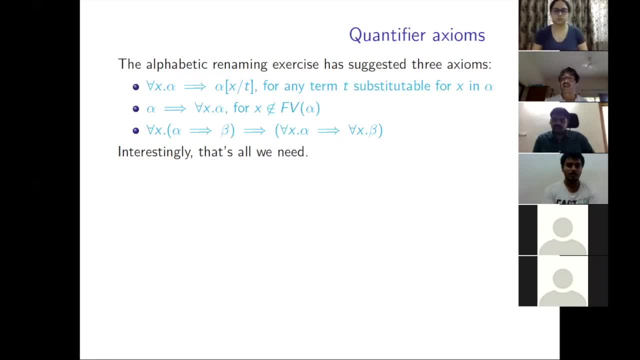 This, So, And the only other thing was The Reductio ad absurdum Formula. So This is the semantics of negation, And here This is the semantics of. So this is the semantics of implication. That one was the semantics of negation. 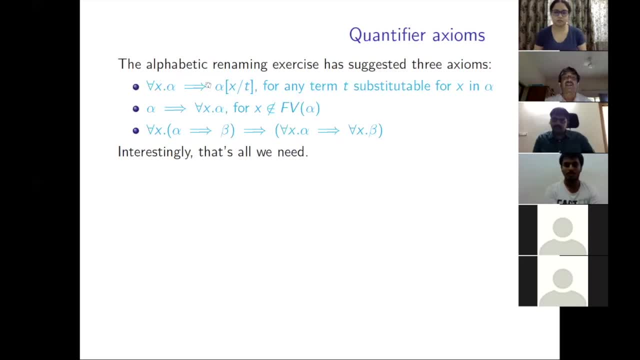 And this is the semantics of quantifiers, Right? This is the essence of quantifiers, Once you understand this. So, And Interestingly, That's all we need, And What is very interesting is that These axioms, I am introducing them. 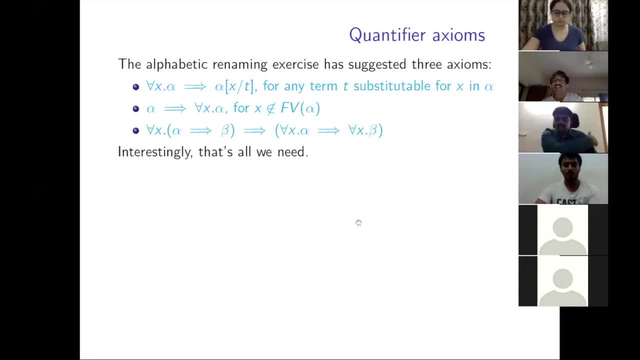 For proving something that looks completely trivial. What is that? Bound variable Renewable And This, This, This, This, This, This, No Bound variable Rename. That is the context in which we got these And that's it. 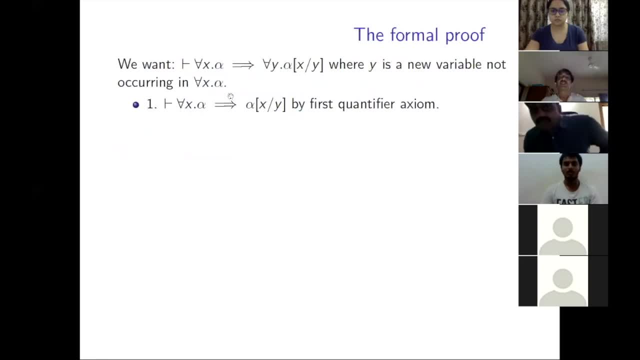 These are the axioms You will need for month. So Let's go over the formal proof What we just did. Let's now make sure that we have got it all We want For all x alpha. It implies for all. 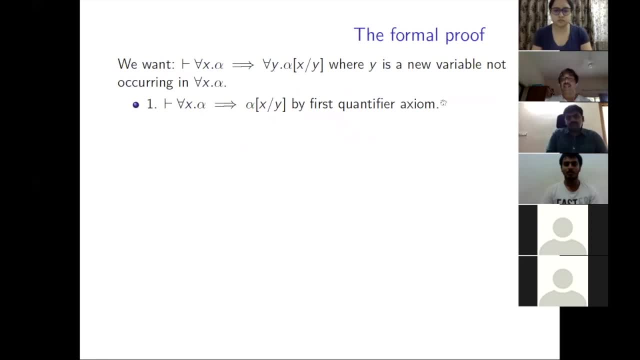 y, It takes Replace By y, Where y is a new variable Not occurring in the left hand side. So The first is by the first quantifier axiom, Because y is substituting for its Rrones. Second, The answer. 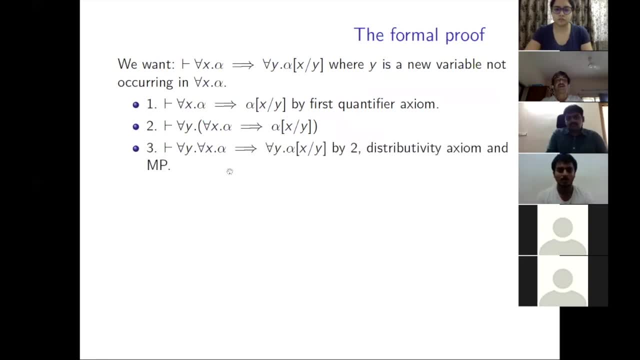 generalization is for free. third: you distribute for all by distributivity axiom on two, you will get for all y for all x alpha. in place for all y alpha. now. for all x alpha. in place for all y, for all x alpha, since y does not belong. 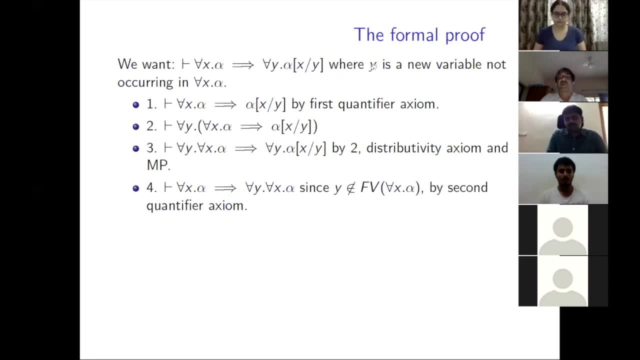 to the free variable. so we know that's a new variable. so the third quantifier axiom gives you this or second. sorry, so now chain three, four, using modus by four. three propositional reasoning: alpha implies beta, beta implies gamma, therefore alpha, and you get what you. so all the three axioms are used, that's. 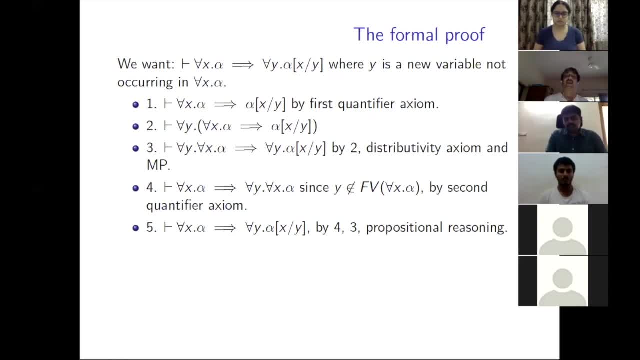 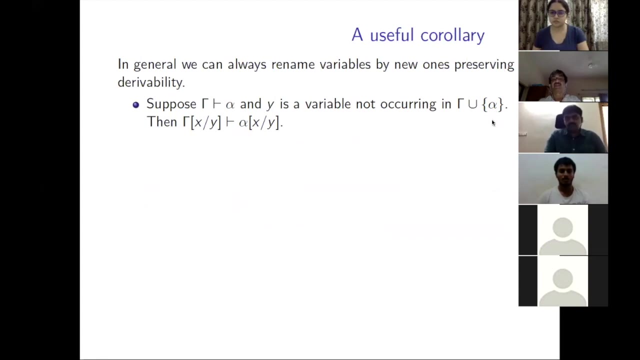 what I want you to realize, and they are used in an essential. any questions related to that related to this. so far, so it's ok, and there is also a very useful corollary and reasoning now. in general, we can always rename variables by new ones, preserving their ability. so not just this in the context of the 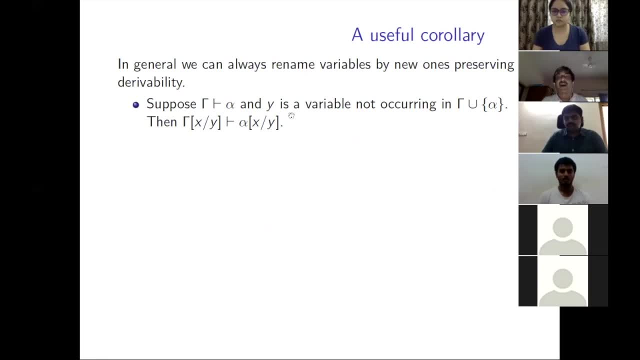 universal quantifier. suppose gamma derive alpha and why is a variable not occurring anywhere in this proof? then if I replace y by X through all x gamma, this is a notation to say in every formula in gamma I replace X by Y. from that I can get a proof of alpha. how would you do that was by proved by. 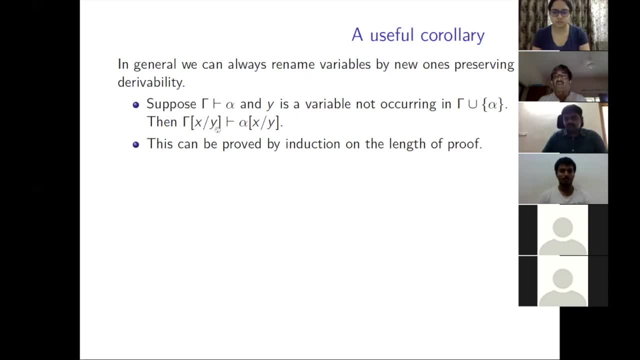 induction on the length of the truth. take this proof here, modify it and you can show that at every step it works. how will you show that? well, if it belongs to gamma, then the corresponding formula with the thing replaced also belongs to gamma. no problem, proof can be rewritten if it was an axiom. we just observed that. 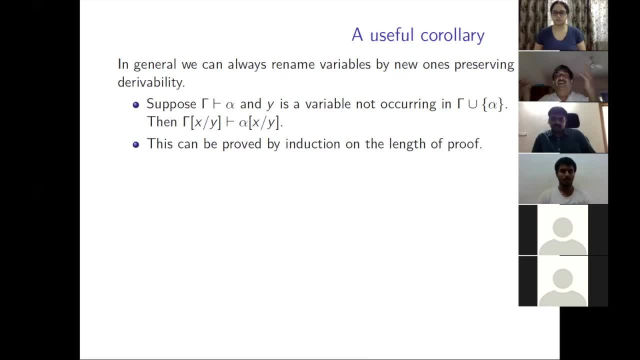 variable renaming in an axiom doesn't work at all right. if it's a valid formula, it will continue to be a valid formula, so with axioms also. and then you use the induction hypothesis, use modus ponens, and so it will work correctly. so this also shows, and this is something important and we are going to need very 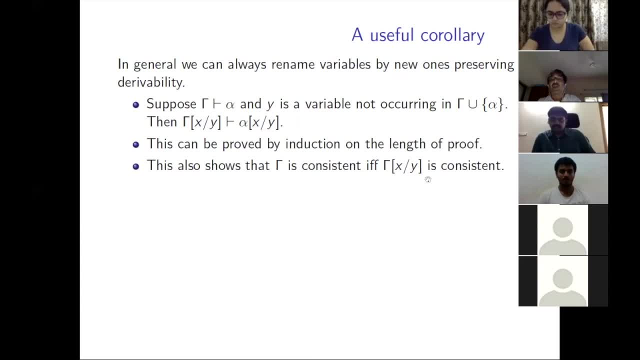 soon is that gamma is consistent if, and only if, gamma with X replaced by Y is right, that is, if the original set was consistent. after variable replacement, it continues to be consistent. if the original set was inconsistent, the bound, the variable renaming, is not going to affect anything. why am I telling you this, remember? 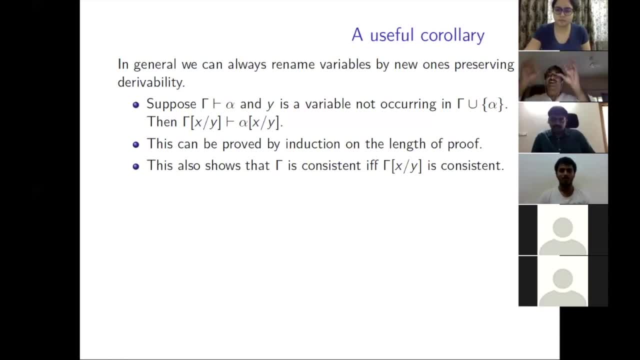 Siddharth, that original point that we made. right, start with the consistent set gamma. I said you're going to rename all the variables. odd numbered variables will all you know X I will. we have to prove that the resulting set is consistent. right, the original set was consistent. 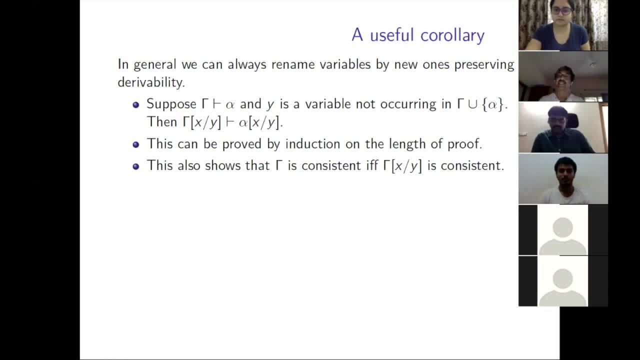 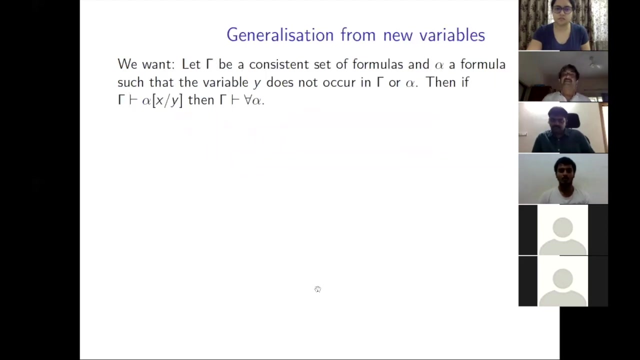 this is exactly right and that's why I'm saying yeah, that this is an argument that will show that by doing these jugglery with the variables, you have not heard. consistence- I mean, these are somewhat pedantic things, but fairly important. and then generalization: remember, the key limit that we had earlier was 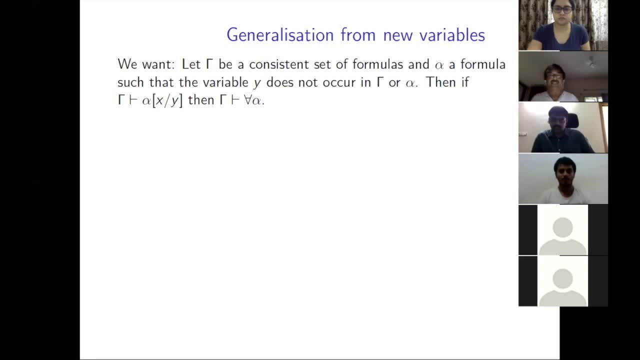 the generalization from constant. now we want generalization from new variables. what is that is the third step. so let gamma be a consistent set of formulas and alpha is a variable. alpha is a formula and such that a variable Y does not occur. then if from gamma we can derive alpha with X replaced, 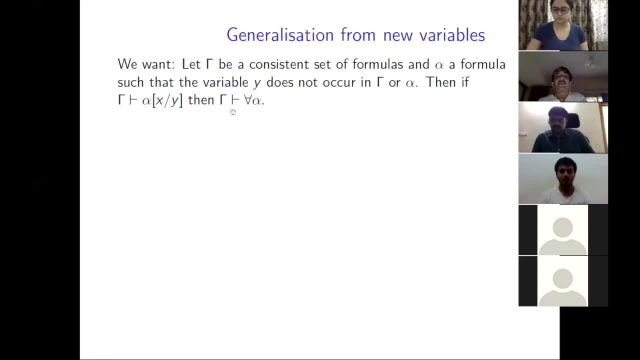 Y, then from gamma we can derive alpha with X replaced by Y, then from gamma we can derive alpha with X replaced by Y, then from from Y, from negative gamma, we can derive for all x alpha. So this is this, you know the key lemma, which is what we had. 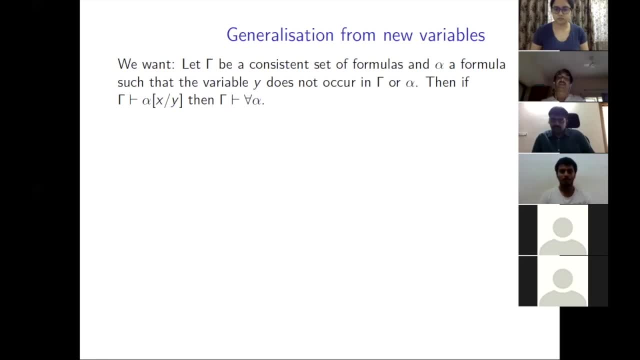 a generalization for constants earlier. Now we want to do that with new variables. How would you do this? Well, suppose let pi equals beta 1 through beta m be the proof. right, We know that there exists a proof. Let pi be the given proof. We will transform that proof, as usual, to a proof. 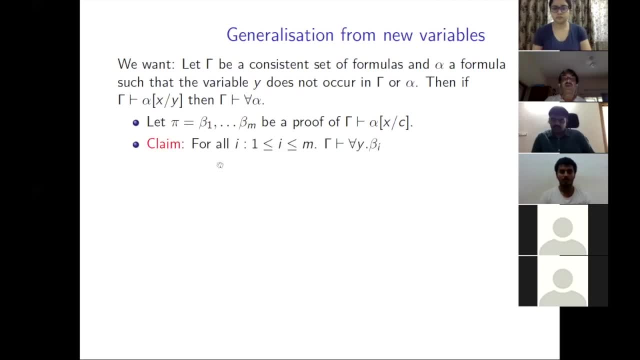 of this. Well, the claim for all i 1 less than or equal to i, less than or equal to m, gamma derives for all y beta i. y is the variable. If I prove this, what will I get? Assuming the claim? we will get for beta m, which is alpha, replaced with x, replaced by y, I will get for all y, alpha. 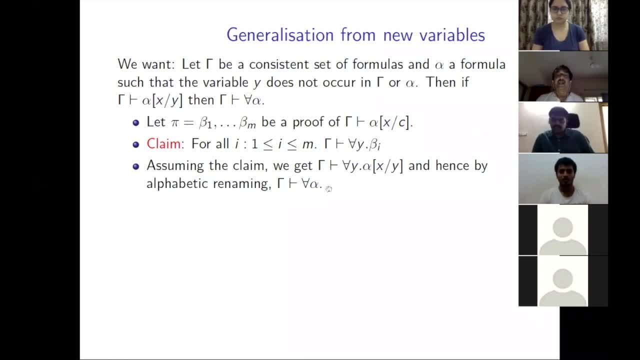 x replaced by y And by alphabetic renaming, which is just what we proved recently. I will get not for all alpha, for all x alpha. Yeah, so you remember. we just went through this trouble to prove. So of course you get what you want. So it suffices to prove that at every step that you have got. if I have derived, 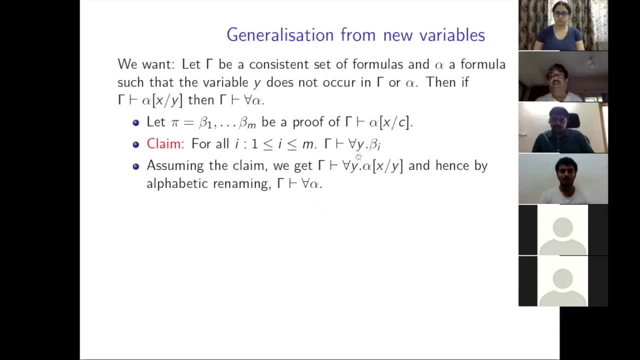 beta i, I can derive for all y beta. Is this clear? So I just proved this. And how do I prove this? by induction. This is the whole thing about proof transformation. right, and this is the kind of thing that you've seen before. Ok, Is the idea clear? Now let's do the induction proof. So we want for all i gamma. 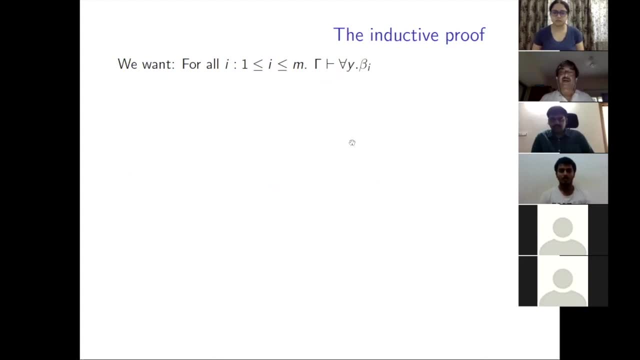 derives for all y beta. i Well suppose the proof is of length 1.. Then I know that beta i must come from, from lambda, and the other thing is that if you want to use this thing, then term an axiom or beta. I belongs to gamma, but gamma has no occurrence of the 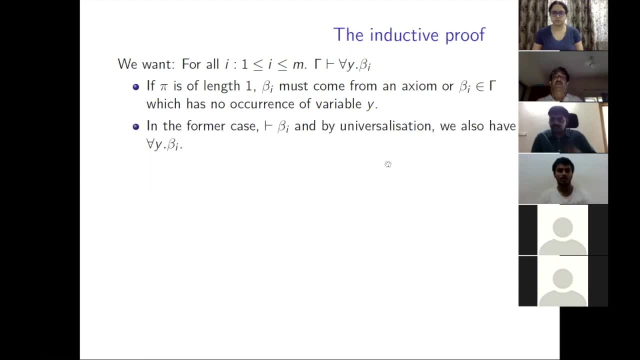 variable Y will keep that in. well, in the former case, beta is an axiom. so there is a proof of one simple for me, time by universalization we also have for all Y beta. right, for all Y beta is also remember you are always allowed in the same. in the latter case, right beta, I belongs to gamma, but it's got no. 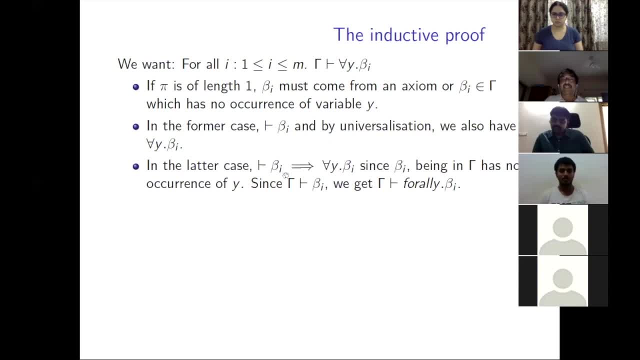 occurrence of the variable Y by our axiom. therefore, beta I implies for all Y, beta. I is an instance of the axiom. remember what does it mean for all Y, beta. I is an instance of the axiom. remember what does it mean for all Y, beta. I is an instance of the axiom. remember what? 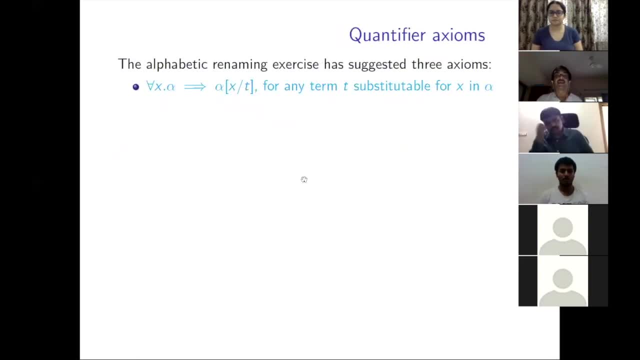 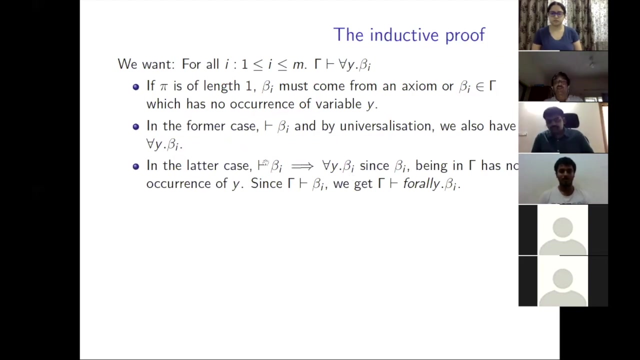 was the axiom, sorry. yeah, this one alpha implies for all X alpha. if X is not a free variable, so we can make use of that right. so Y has no free occurrence here. so beta I implies for all, since gamma beta i. therefore gamma derives- okay, there is a typo here. for all y beta i. 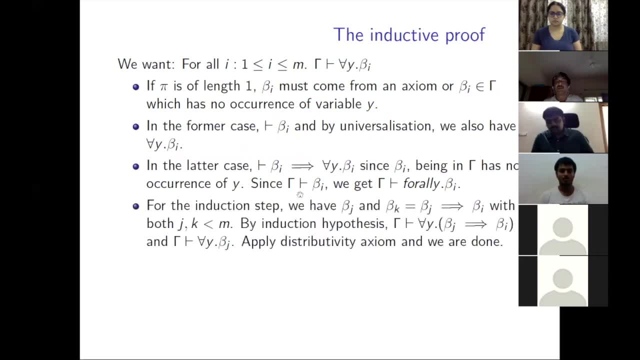 so this is the. that takes care of the base case for the induction step. we have beta j and some beta k, which is beta j implies beta i, with both j and k less than i. you have already proved beta j and you have proved beta j by induction. hypothesis gamma derives for all y. 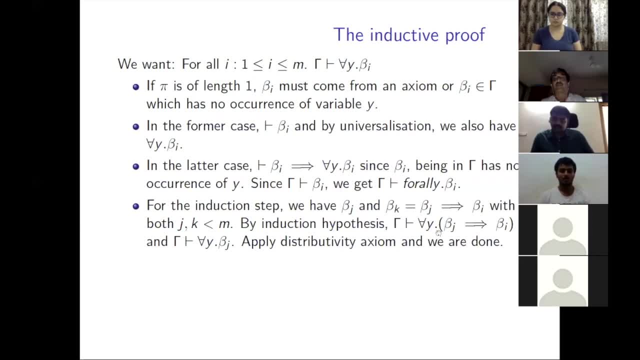 beta j implies beta i and gamma derives for all. y beta j. right, but now you apply the distributivity axiom, you will get: gamma derives for all. y beta j implies for all y beta i now, but gamma derives. this. therefore, gamma derives for all, and we are done so with the quantifier axioms that we have. 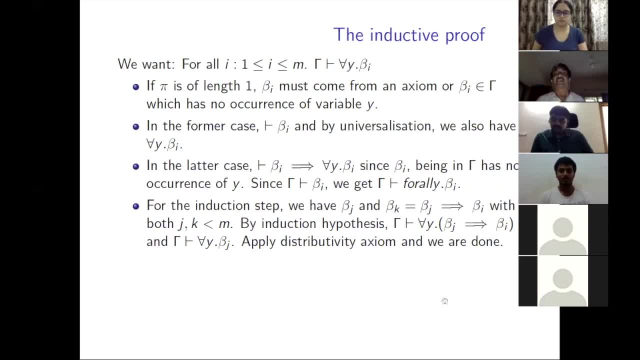 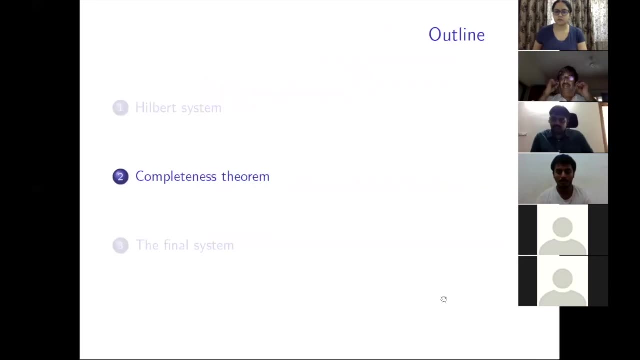 got. we can actually prove the generalization from here. so basically, all the three important steps that i pointed out- you for the stepping stones, for the completeness proof, they are all there for us. so now we are ready to prove the complete. still one moment. i'll switch on the light. it's getting. 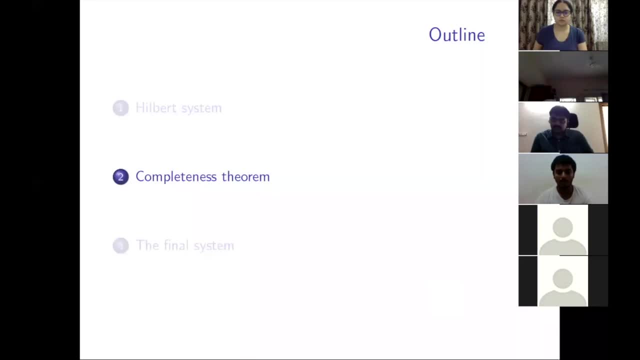 dark. okay, yeah, so ready for the completeness theorem. so this is Gerald's 1930 theorem. given a consistent set gamma show that it is satisfying. but i'll just go over the steps that we said and we'll now go over the details and steps for which you've got all the things in place. extend. 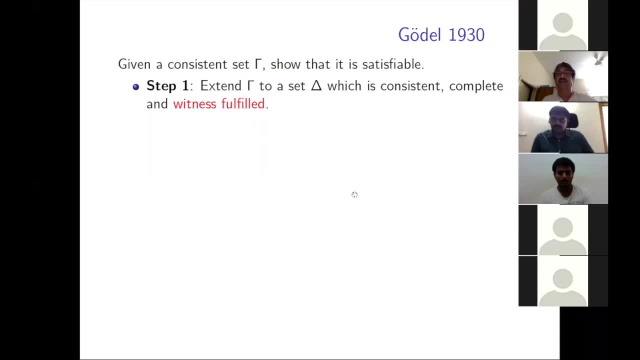 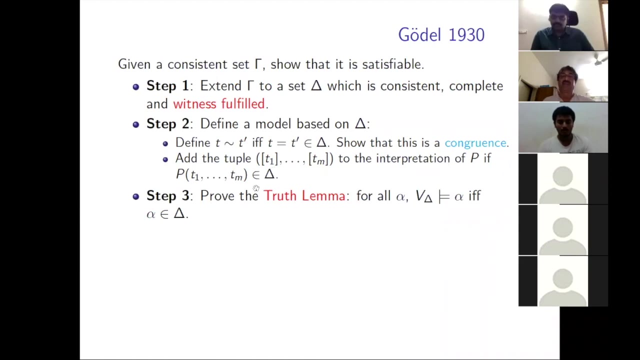 Extend Gamma to a set Delta which is consistent, complete and witness fulfilled. Define a model based on Delta for which, first you define this binary relation and show that it's a congruence, and use that to define the interpretation for the predicate symbols, and then prove the truth. lemma. 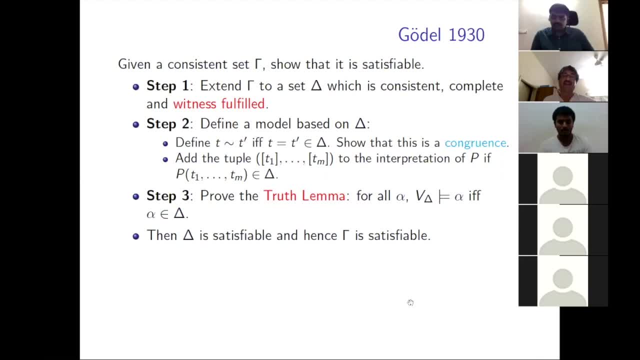 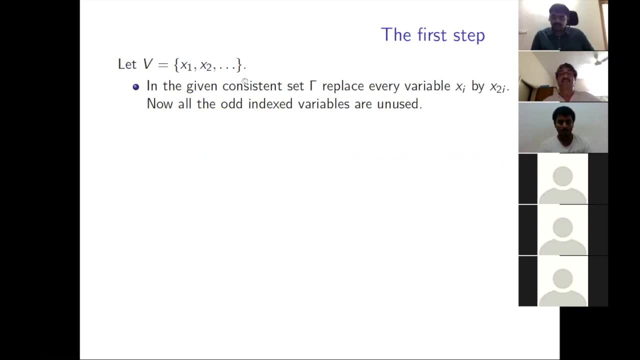 So there's not V Delta here, it should be model M Delta. So what is the first step? We have a bunch of variables In the given consistent set Gamma. replace every variable by xi, by x2i. Now all the odd index variables are unused. 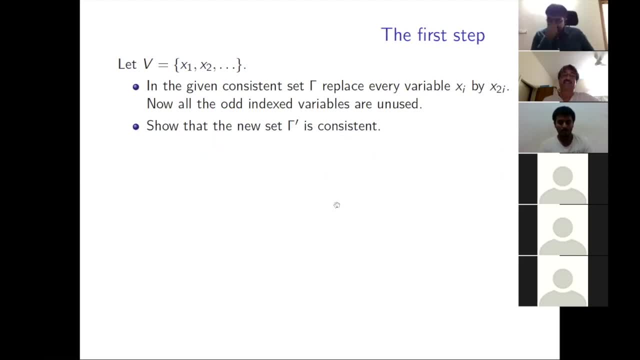 Now we want to show that the new set Gamma prime is consistent. How do I show that? Well, some bit of trickery involved here Suppose not. Let Gamma1 be a finite subset. that is inconsistent. Well, let x2n be the first variable not occurring in Gamma1. 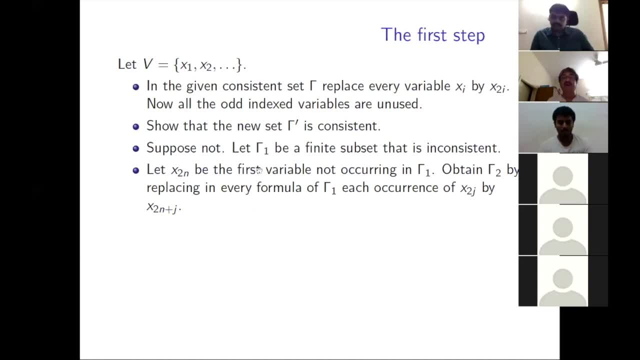 Obtain Gamma2 by replacing, in every formula of Gamma1, each occurrence of 2j by 2n plus j. Basically, I'm shifting all the occurrences in Gamma1 to get Gamma2.. What is the main advantage? Gamma2 uses new variables not occurring in Gamma1. 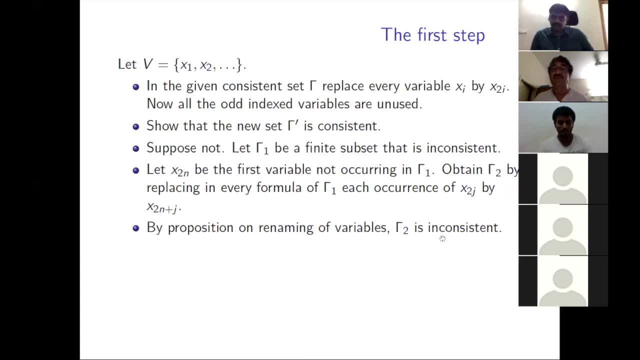 Right. So In my position on renaming of variables, Gamma2 is inconsistent, Right? Remember that when I use new variables and rewrite, one set is consistent if and only the other is So. Gamma2 is a finite set and that is inconsistent. 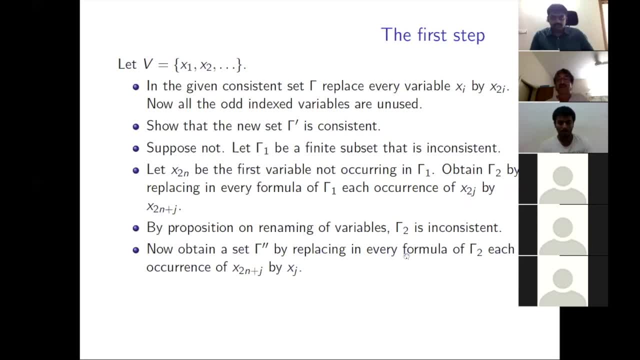 Now obtain a set Gamma double prime by replacing in every formula Gamma2.. Take any occurrence x2n plus j by xj. Again, these are new variables. So What I have done is Now gone back to j. Right, What will happen? 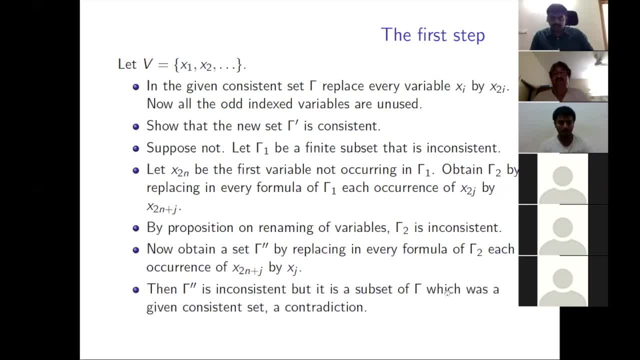 Now, Gamma double prime is inconsistent, but it's a subset of Gamma Right, Remember, that's what we started with and these are all variables in Gamma originally So, but that was a given, which is a consistent set, and that's a contribution. So, basically, this is make sure that you understand. this is a little bit of jugglery, but you actually 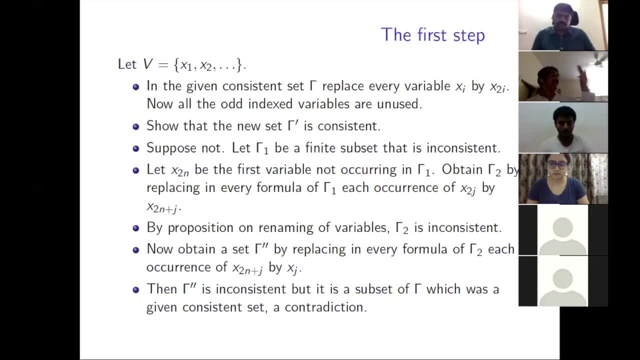 need it, Mainly because Why I started with the original consistent set. I have renamed everything and I want to show that the new set is consistent. Well, if it's not, there is a finite subset and I have to argue that if this set is inconsistent. 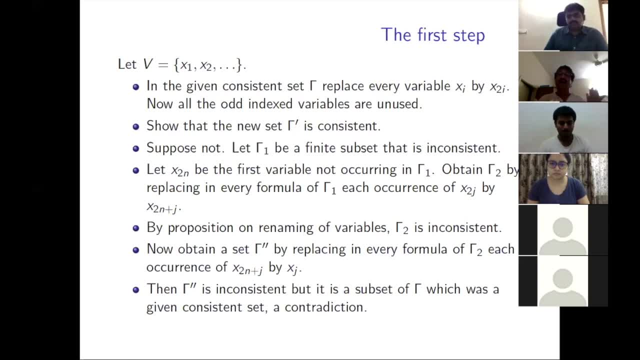 the original set is inconsistent as well. Now for that. I can't refer to the. I can't say, hey, take all this doubly index variables Right. I can't say they are all new variables. Remember, there is a, you know. 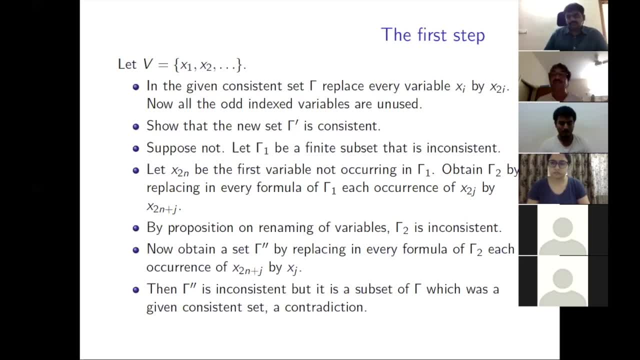 You know That's because of the scheme that I used Right Where i became 2i Right, So the. if I look at a variable eight, it doesn't mean much Right. I mean so in general the odd variables are unused, but even variables were there in the. 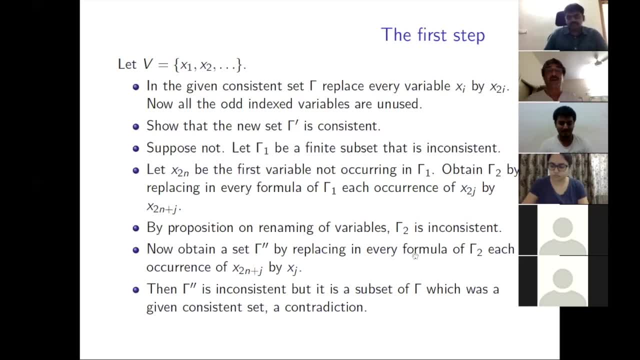 original set as well as in the new set. So that's why all this jugglery is needed, but make sure that you understand the steps. but it's fairly simple, Right, Because it's because I've taken a finite set. Therefore it's there is a maximum there. 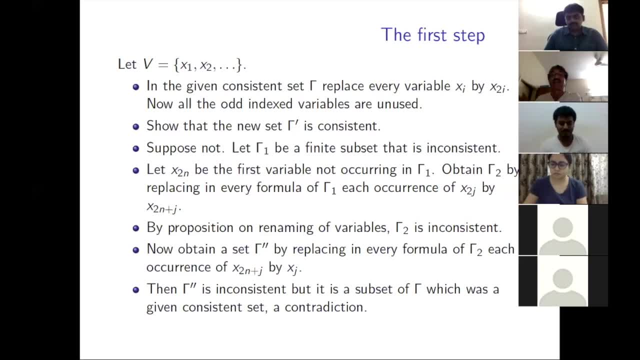 So you always go far enough and rename the variables. that will always be new variables available, New for gamma one. That gives you gamma two, which is inconsistent. You've gone far away. Now you replace and get the original set gamma and you will find your inconsistency. 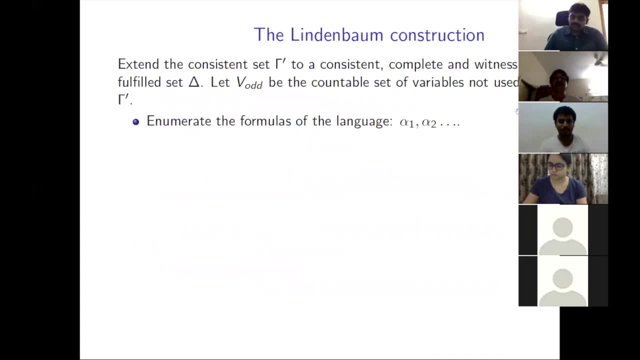 Okay, Now the Lindenbaum construction. We now have an consistent set Gamma prime. We want to extend it to a consistent, complete and witness fulfilled set delta Question. Yeah, please, I mean, why can't we just scale back and get the original set? 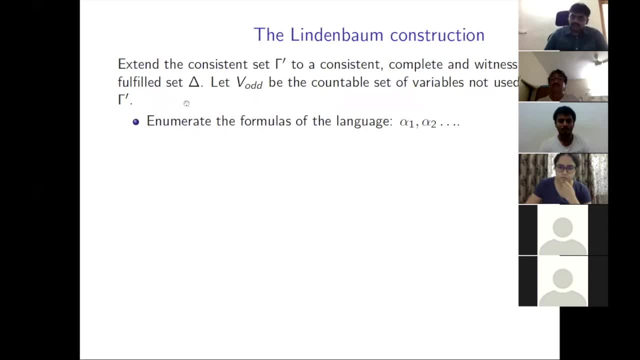 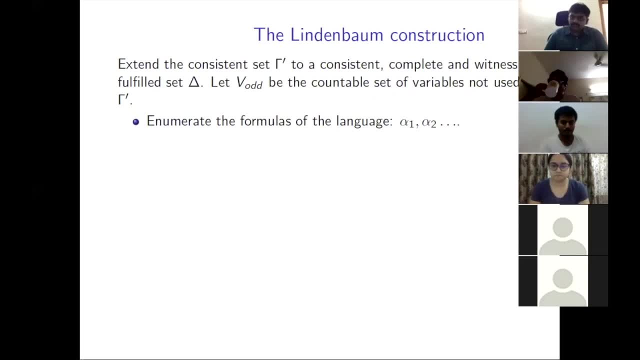 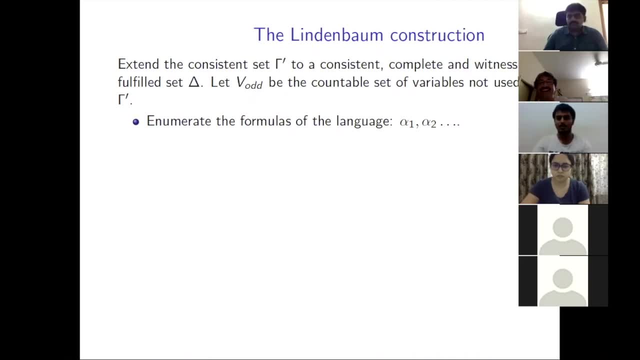 Okay, okay, thanks, yeah, so it does a trick. any other question? okay, and this is the Lindenbaum construction. now enumerate the formulas with the languages: alpha 1, alpha 2, etc. examine them in turn and add. that is idea. define a sequence of sets: delta 0, delta 1, and so on. delta 0 is the original set, gamma prime that we have. 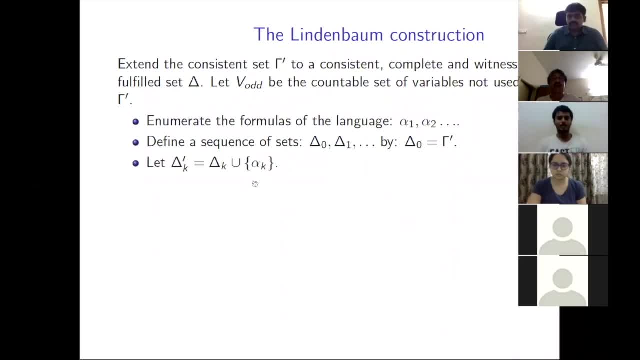 got and at every stage we look at alpha K. let delta K prime be delta K union alpha K. we have to examine whether delta K prime is consistent if it is call that delta K plus 1, except that in the case of existential formulas we have some. 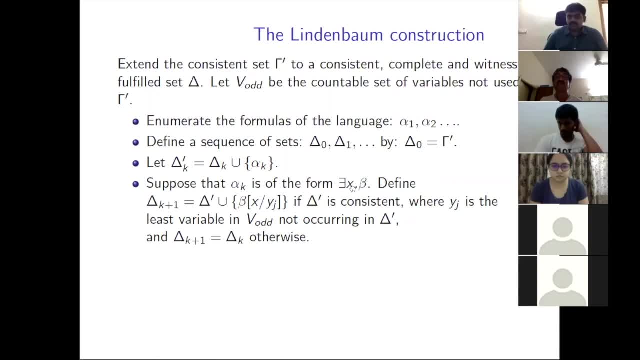 work to do. suppose that alpha K is of the form there in 6 beta. define delta K plus 1 to be this set delta prime union. along with whatever I have got, I have to add a witness for beta for X, so that is beta with X replaced by Y, J if delta prime is. 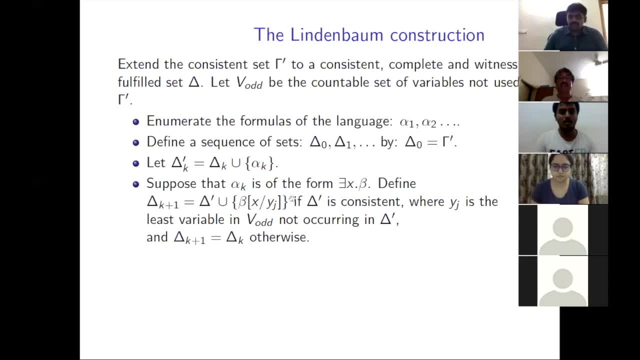 consistent where Y, J is the least variable now not occurring in delta. why should such a variable exist? and is the important point when I start this induction, none of the variables in B odd is used. that gamma prime doesn't have any of them, so by stage K I would have used 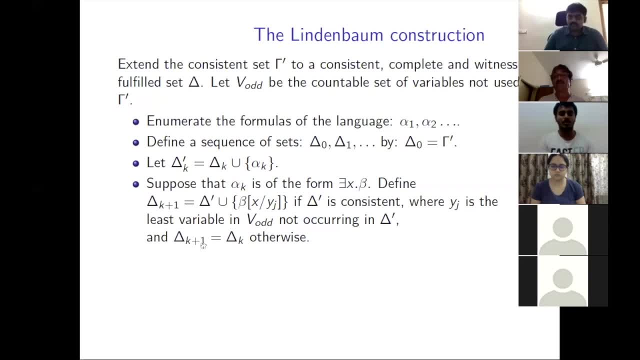 up at most K variables here, probably fewer. so there is, since that's an infinite set, this there will be variable not occurring in delta prime. take the least among the enumeration and put that in. we need something specific right to make it the terms. and then delta K plus 1 equals delta K. otherwise, where they're, 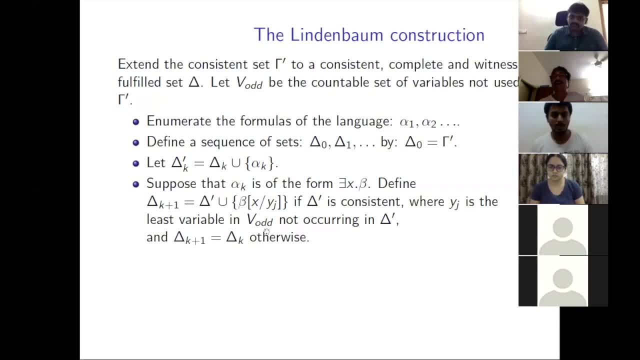 not touching it if this is not consistent. anyway, you can't add right. and what we have proved is that if this can be added consistent, I mean if there exists X beta can be added consistently. you can also add beta with X replaced by Y, J, consistent. this is what we prove moment ago. if I'll come, alpha K is not. 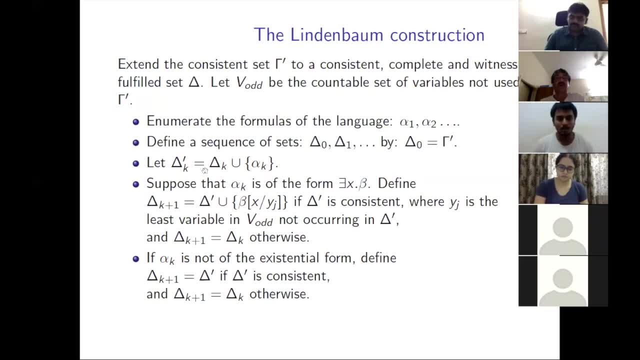 of the existential form define. let's take a: plus 1 equals this: if this is consistent, and that's okay. otherwise, now define Delta to be the union over all: K, Delta, K, and we can show that Delta is consistent, complete and it is perfect. how do you prove this? well, first you. 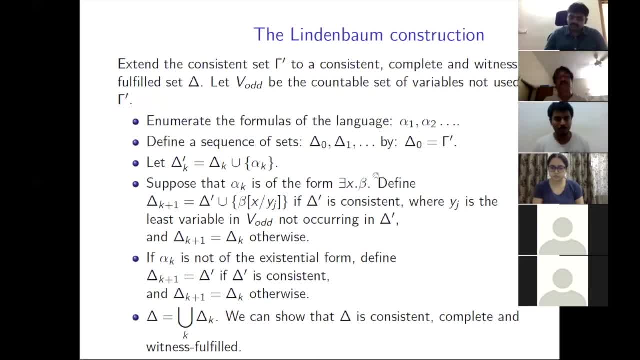 prove that for all K does that create consistent? how do I prove that? well, here is a step that where we need to prove. suppose there exists X beta, I can add: consistently. this set is consistent then with the witness also. it is hard to prove that, well, suppose not? 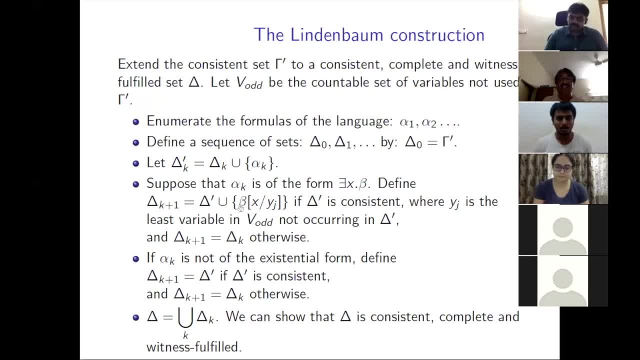 then delta prime derives. negation of this by generalization from variables: delta prime derives for all X right it. there is not beta. therefore it is for all X naught beta. but we just said that exists beta, so delta prime derives, that exists beta. delta prime derives for all X naught beta. therefore that contradicts. 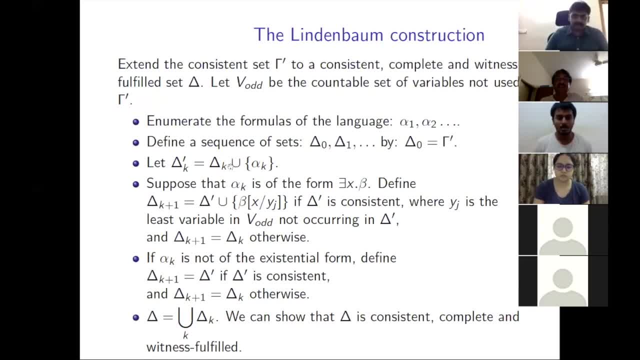 consistency of delta prime. so clearly: for all K, delta K is consistent. from that you can show: delta is consistent. okay, suppose not. then you can get a contradiction from Delta. that means you can get a contradiction from some finite subset of Delta and that's dominated by some M. but we just said: for all M, delta M is. 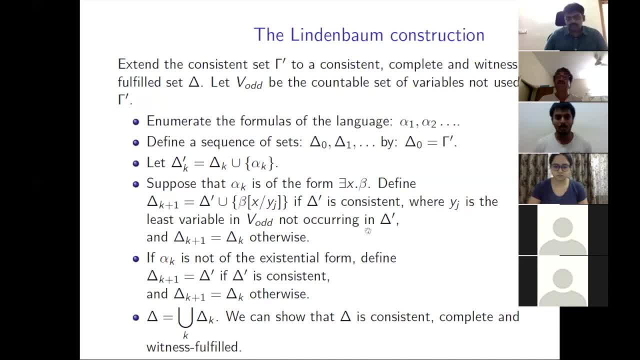 consistent. so that's what? why is it complete? well, using the propositional fragment, we can show that if Delta is consistent and alpha is any formula, either delta union alpha is consistent or delta union- negation alpha is consistent. one of them will show up in the enumeration and you. 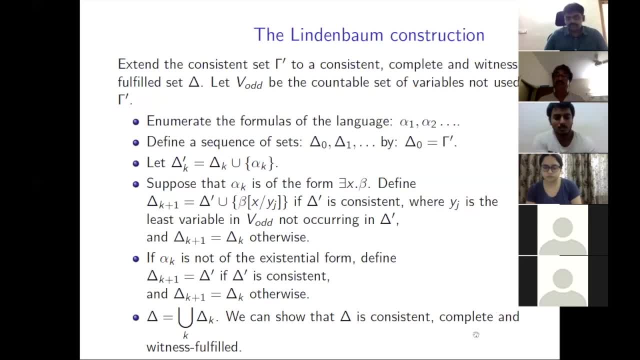 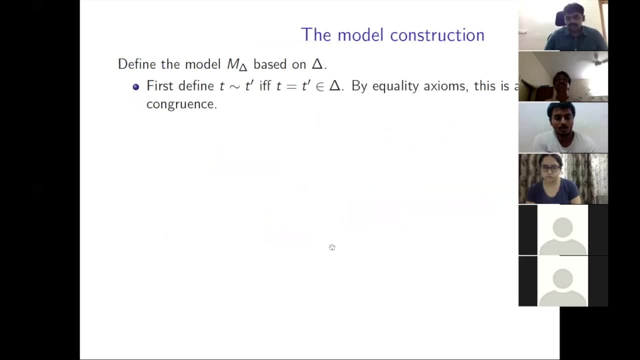 will add it. therefore, for any formula alpha, either alpha gets into delta or negation witness fulfilled is by construction. so now we have to do the model construction. define the model M delta based on delta. define the binary relation T equal to T prime, but only if T equals T prime. 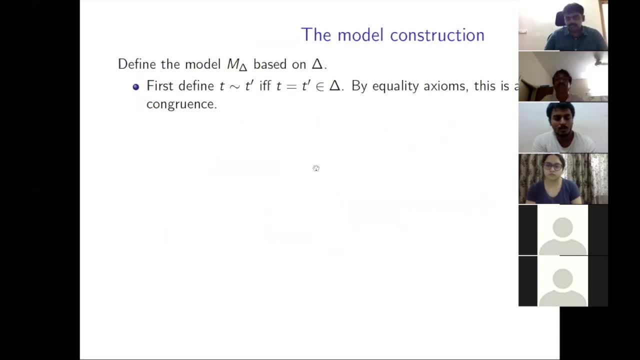 belongs to delta by equality axioms. we know that this is a congruence define. take the set of all terms quotiented by the equivalence relation, and that's the domain interpretation for constant symbols. every constant symbol is the equivalence class of C. interpretation of function symbols: well, it takes k-tuples. 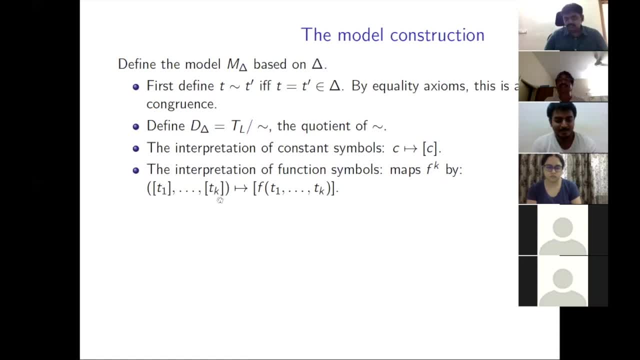 of domain elements, k-tuples of equivalence classes, and then maps it to the equivalence class of F applied. now, since that's a congruence, this is well defined. then, assignment pi: for a variable X, I have to map an element of the domain that's the equivalence class of X. we then observe: 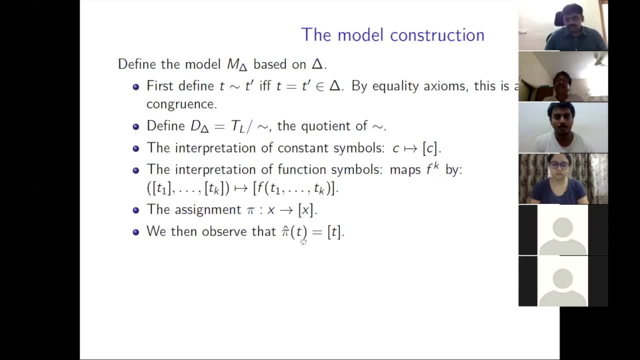 that if I lift pi, the pi hat of T equals the equivalence class of T. so this is a all stuff that we have done before. the interpretation for predicate symbols maps, and emery predicate symbol has. well, it has to map m-tuples of elements of the domain to 0 or 1. it puts 1 exactly if this formula: 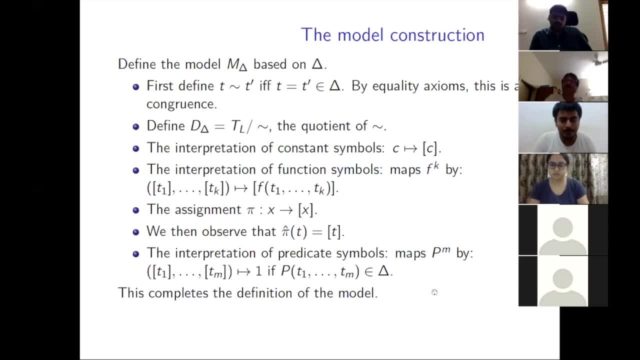 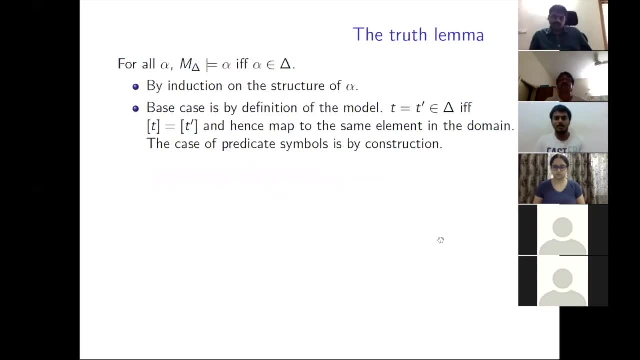 belongs to delta and this completes the definition of the model. and it's. everything is here is well defined. pi hat works exactly so. now, in this model. now we claim the truth lemma. we claim that for all alpha, alpha is true in the model if, and only if, alpha belongs to delta. now this is proved by induction on: 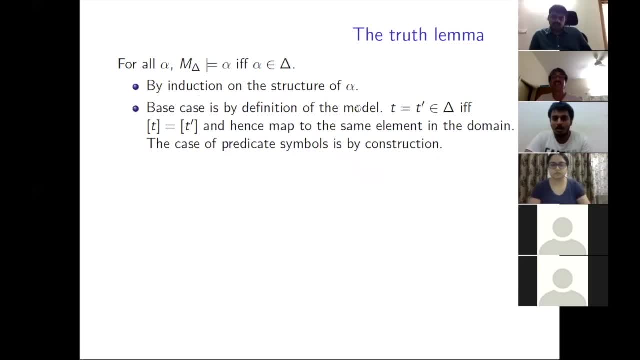 the structure of alpha base case is, by the definition of the model: T 1 equals T. prime belongs to Delta if, and only if, these two are in the same equivalence class and hence map to the same element of the domain, which means T 1 equals T 2. 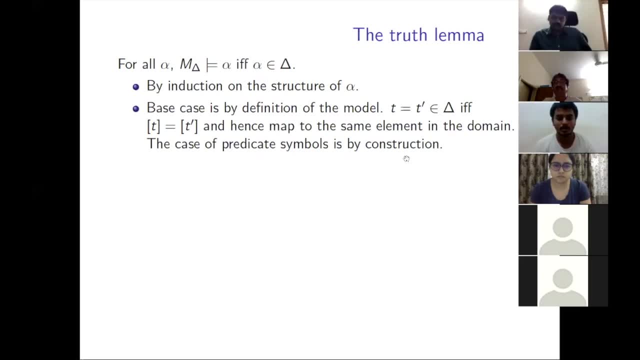 is true in the case of predicate symbols is exactly what we said by construction. now the induction step for propositional connectives follow the following steps for propositional connectives go from the fact that Delta is a consistent and complete set. this part of the proof goes through exactly like a propositional logic. just to be sure not. 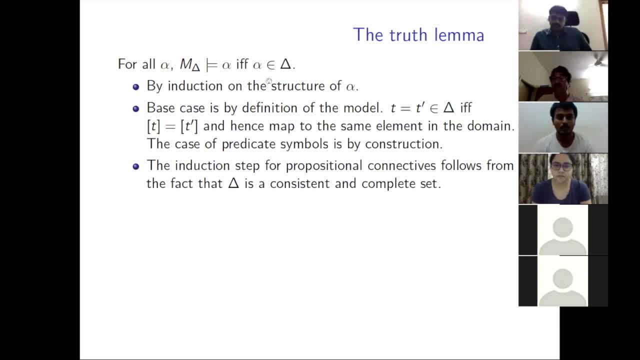 beta belongs to Delta if, and only if, beta doesn't belong to Delta by the fact that it's consistent, complete, which by induction hypothesis means in the model, beta is not true. if beta is not true in the model, not beta is true, and similarly for the implication case. 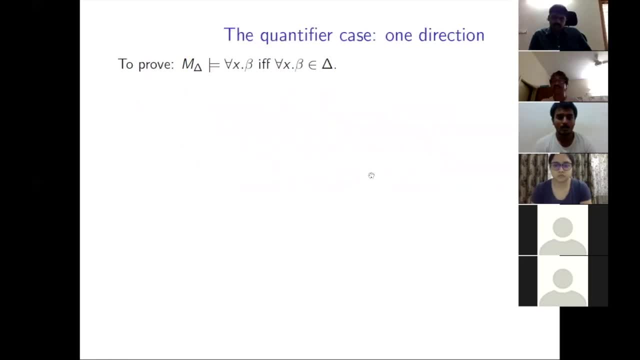 now. so basically it's a quantifier case that is left. listen said all the elements are in place. you just have to go work through the definitions. we have to show that for all X beta is in Delta if, and only if, the model makes for allx beta. 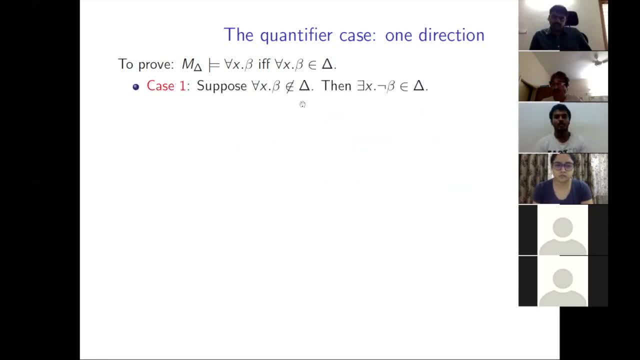 well, suppose for all X beta is not in DEL. we want to show that for all X beta is not true in the model. if for all X beta is not clear, it negation is there. that is, there exists X, not beta. belongs to delta. let Awards to delta, But delta has witness fulfilled. That means not beta with x replaced by y for some new. 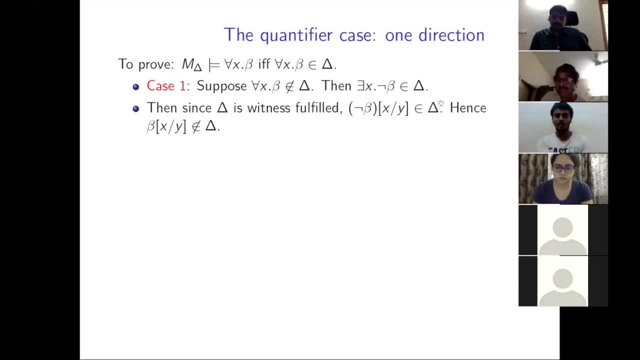 variable belongs to delta, Which means delta is consistent. therefore beta with x replaced by y is not in delta. By induction hypothesis that means the model does not make beta with x replaced by y true. Now y is substitutable for x and beta. So remember that old proposition. if the term t is 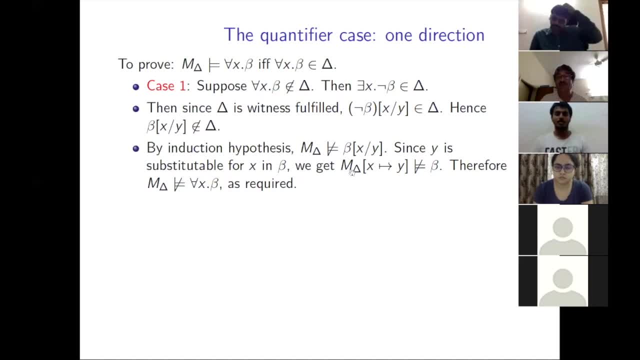 substitutable. you can push it to the left hand side. That means, if I look at the model variant, where x maps to not y, but equivalence class of y, That is- I missed that here- equivalence class of y. that does not satisfy Well. this means that there is some domain element for which the variant 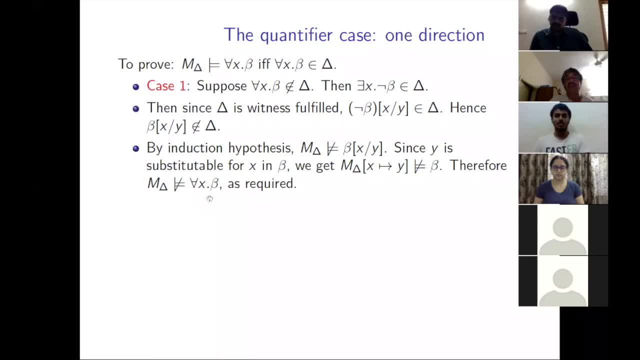 doesn't satisfy. So that is why I am saying that the model does not satisfy. So that is why I am saying that the model does not satisfy. So that is why I am saying that the model does not satisfy beta. Therefore, in the model for all x, beta doesn't pass the code. So if you remember, basically, 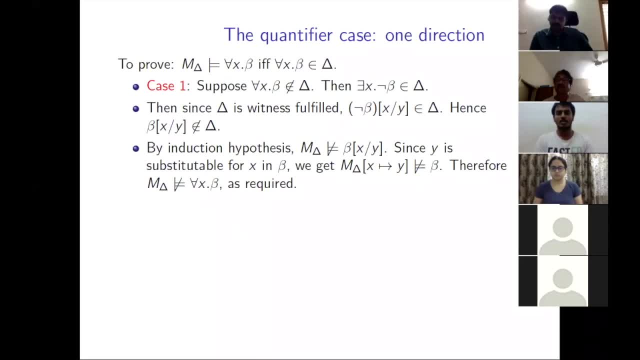 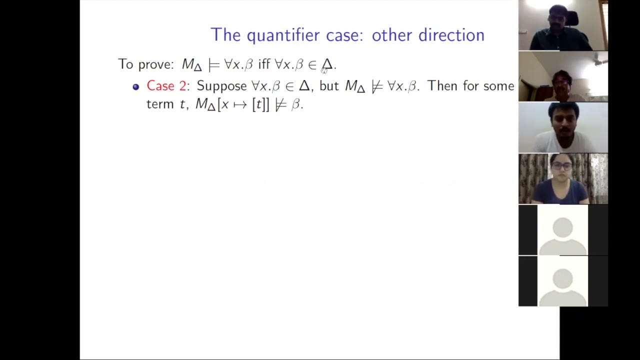 what I am mimicking is how we did the compactness proof argument, except that we are doing everything with respect to consistency here, and that is the only difference. Now there is the other direction. What is the other direction? Suppose: for all x beta. So we assume for all x beta is not in delta. 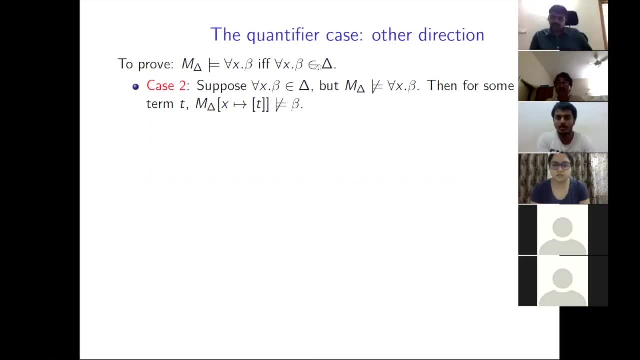 and we prove this is not true in the model. Now we have to Assume it belongs to it and then we have to show this. So suppose for all x beta belongs to delta, but the model doesn't satisfy for all x beta. Then what must be the case for some term t? 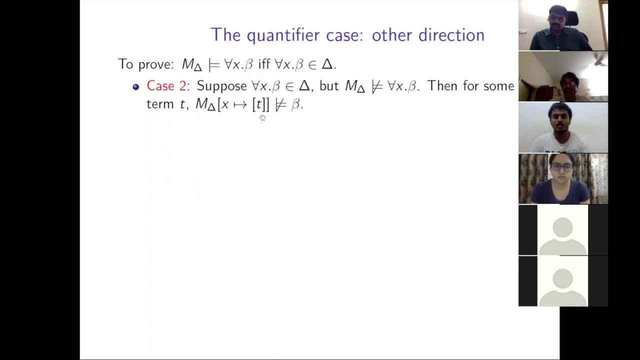 when I look at the assignment x, with equivalence class of t, it doesn't satisfy beta. Now there are two cases: whether the term t is substitutable for x in beta or not. Well, we know that in whatever it is, beta prime exists. If t is already substitutable, call beta prime the same as beta. 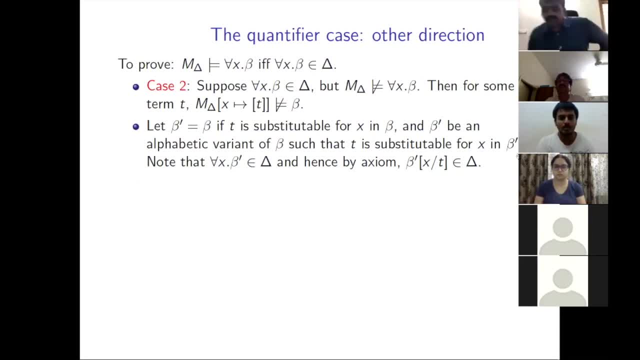 Otherwise, beta prime be some alphabetic variant, such that t is substitutable for x in beta prime. Note that for all x beta belongs to delta, Then for all x beta prime belongs to delta as well. Right, Why? Because, and this is: 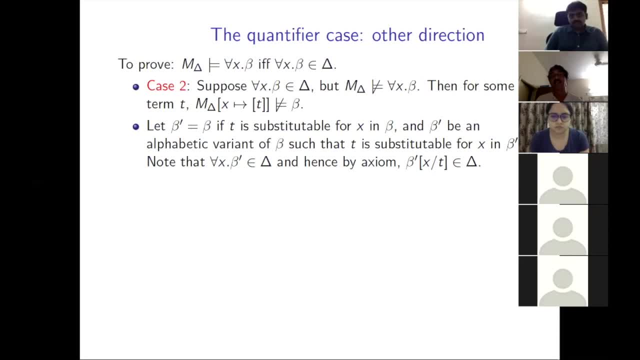 Precisely the point about alphabetic variants Right. They are logically equivalent and that's derivable. So if one of them is in delta, the other is in delta as well, And hence now for all x beta prime belongs to delta. So, by axiom, beta prime with x replaced by t belongs to delta, because t is. 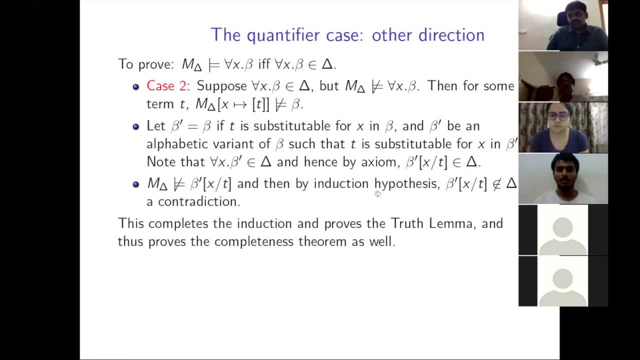 substitutable for x in beta prime Now. So, Oh yeah, Now Correct, Yeah, This doesn't satisfy. beta And t is substitutable, So yeah, So m delta does not satisfy. So basically, Basically here I've got beta prime here And m delta does not satisfy this, And then by induction, 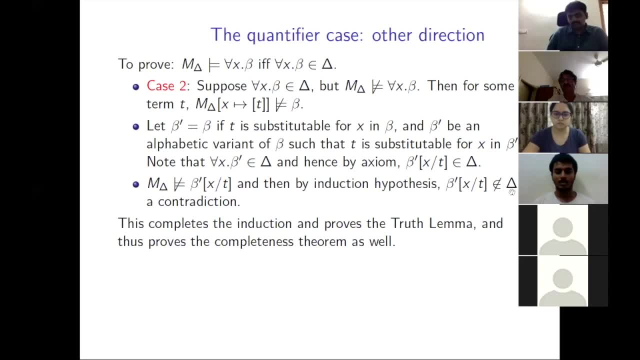 hypothesis: beta prime with x replaced by t does not belong to delta. And that's a contradiction, Because we have just proved that it belongs to delta. Okay, Yeah, So, and this completes the induction and proves that the truth lemma, and that proves the conclusion. 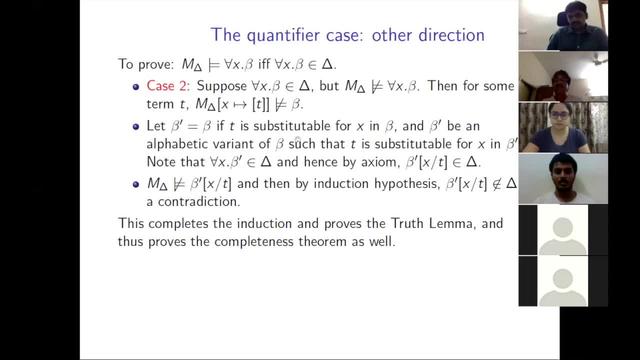 of the lemma as well, And so it's the same business that used the alphabetic variants: See: In general, the formula beta- prime is dependent on the term t. That's why we need to go this way: That there is a term t for which this is violated. And now I go over to beta, prime, Beta and beta. 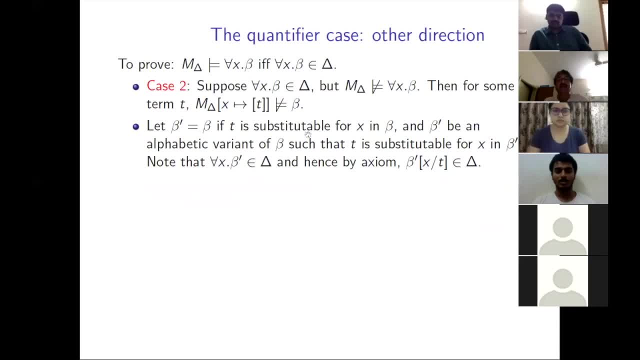 prime are logically equivalent. So any model that satisfies beta satisfy- sorry- satisfies beta prime as well. Since beta is not true in this model, it is equivalent model. beta prime also is not true. m delta with x replaced by t, By the equivalence class of t, does not satisfy beta prime. But since this is substitutable, so you can shift it to the right hand side. 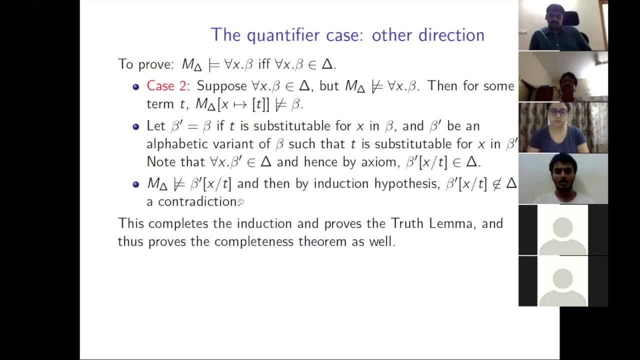 So I can say m delta does not satisfy beta prime with this. Therefore, by induction hypothesis it does not belong to delta. But that's the validity shown this and that's a contradiction. Okay, So this completes the induction and proves the truth. lemma. 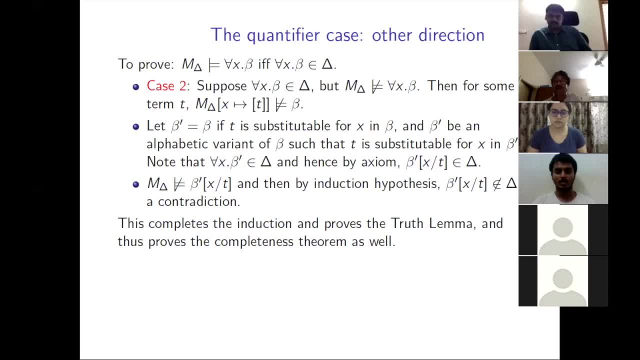 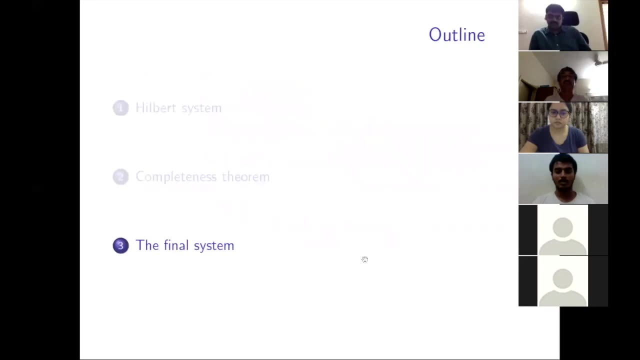 Now from the truth, lemma, you know that delta is satisfiable Now because there is a model for it And gamma is a subset of delta. Therefore that is satisfiable as well. So this completes the proof of the completeness theorem, And so final system. What is that? 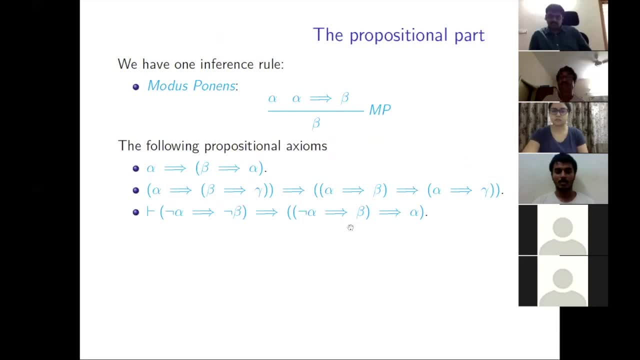 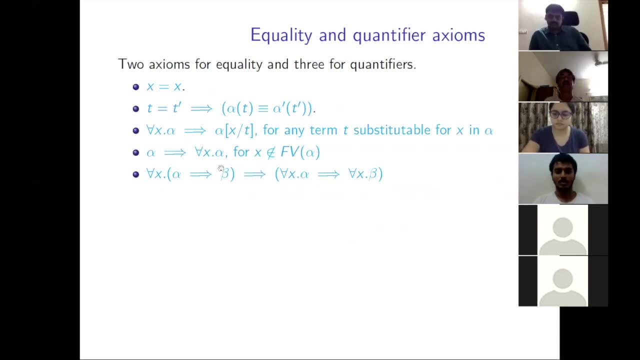 We have one inference rule Following propositional axioms, which are the Hilbert axioms for propositional logic. Then you have two equality and three quantifier axioms. You don't need t equals t, You can just put x equals x. Okay, x equals x and t equals t. 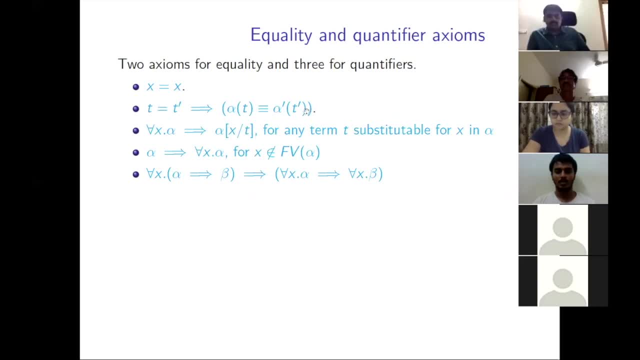 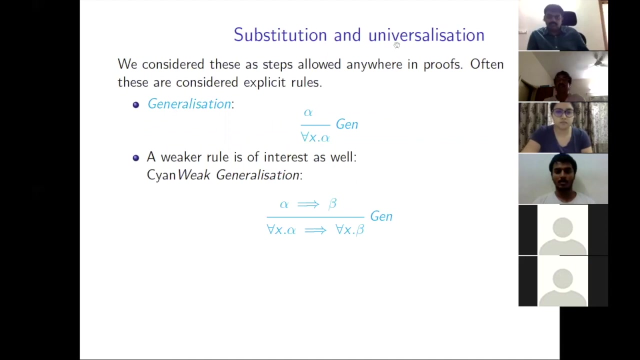 implies- This is the notation that was normally used for what I said- And then the three quantifier axioms. So this is the Hilbert system for first order logic, And here is proof that this is a complete system. Well, now we use substitution and universalization as anywhere in proofs. Now, often, if you look at the literature, 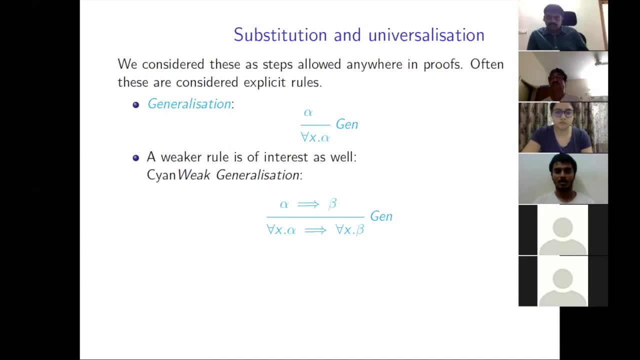 Some of the texts, You will find that these are introduced as explicit rules, The substitution rules for first order. logic is very painful. You have to prove You know, You state everything in terms of atomic formulas And use explicit substitution rule which says how you can substitute. 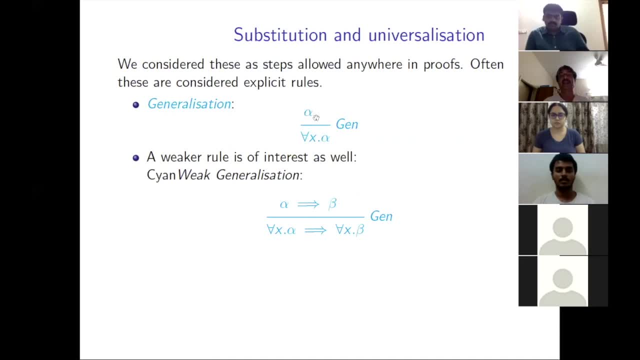 That's very painful, But generalization is very simple. Right, If alpha is derivable for all x, alpha is derivable. Now there is- This is another typo here. So there is also weak generalization there. So there is also weak generalization there.